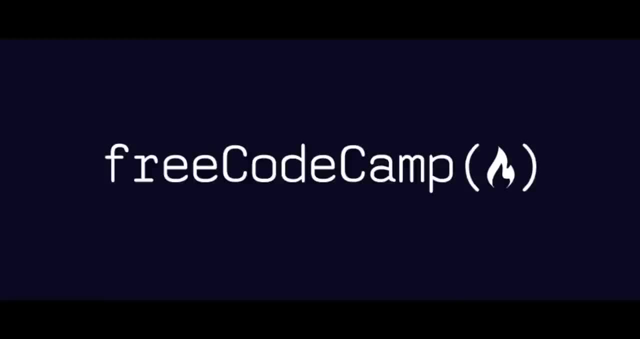 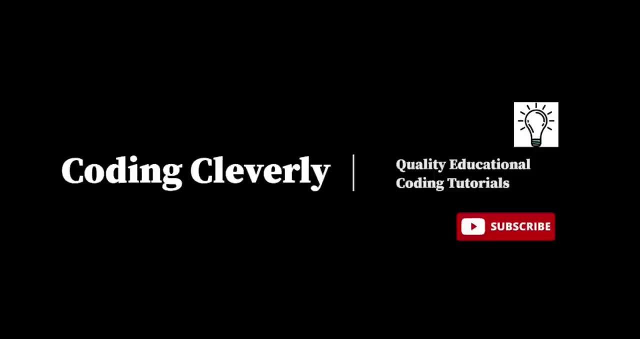 right. Coding Cleverly is being featured by FreeCodeCamp. This video will be about some of the different sorting algorithms that you can apply to almost any programming language. The language focused in this video will be C++. However, like I said, you can apply the 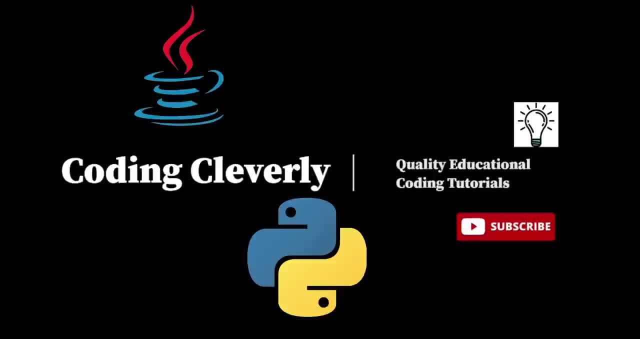 concepts to any other languages of your choice, like Java, Python, C and so on. You would at least need to know the fundamental core concepts of programming, especially the basic programming constructs like sequence selection and iteration, to understand this video Also. 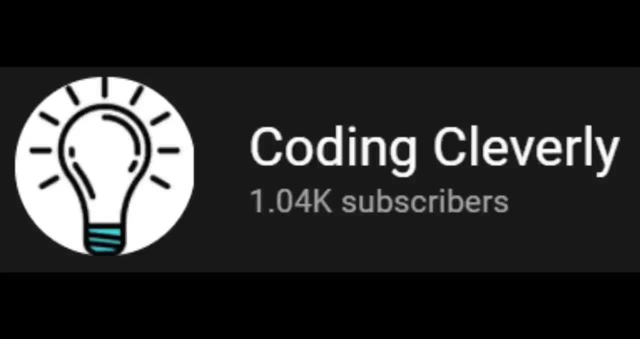 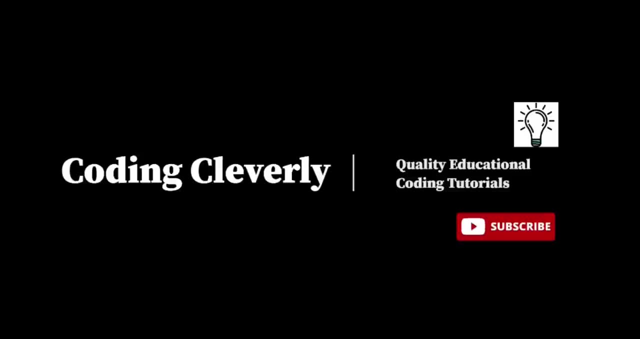 make sure to check out my channel Coding Cleverly, where I've covered almost every concept, from programming fundamentals to object-oriented programming, all the way to data structures and algorithms and beyond. Okay, so let's start by writing a simple algorithm for sorting an array. So first of all, let's 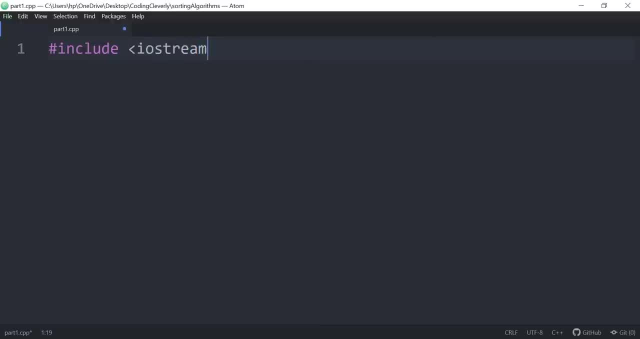 include our Iostream- And I encourage you to type along with me to get the maximum practice. So hash, include Iostream, And then we have our namespace standard, And then we have our integer main And we also have our return zero, right here. 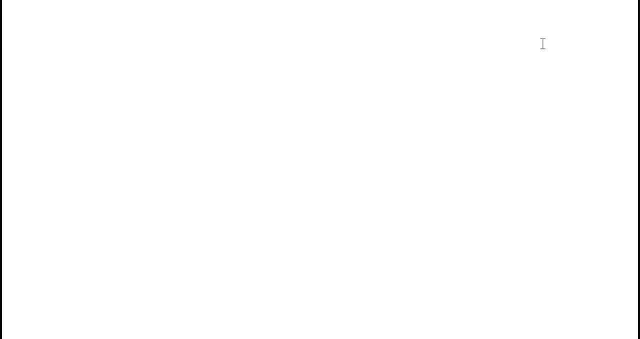 So we're going to start off with a very simple algorithm And we're going to look at its visual implementation. So suppose we have an array of four elements And that's the four sides. we have two, three, one and five And basically this is an array which is 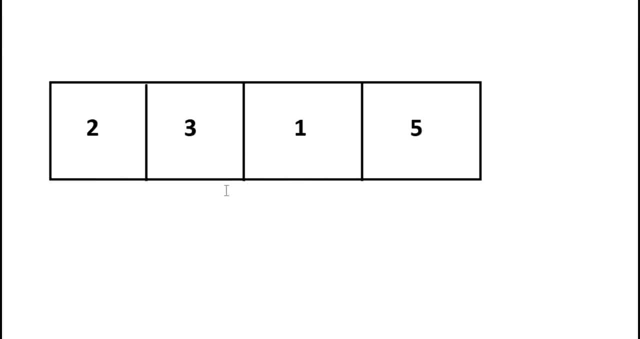 basically indexed, having values from zero all the way to three. So our job is to sort this in ascending order. we know that this is not in ascending order, So we're going to use a very simple algorithm And I'm going to create actually the implementation here. 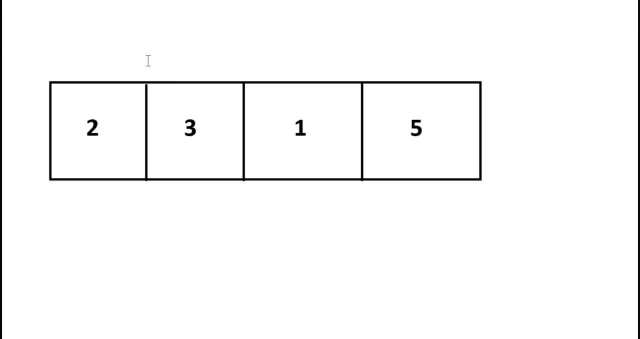 And after that we go back to our code editor and we're going to type along and it's just going to make much more sense. So suppose we have two variables and we're going to have one variable which is going to be enlisted on the top. So we're going to have that as 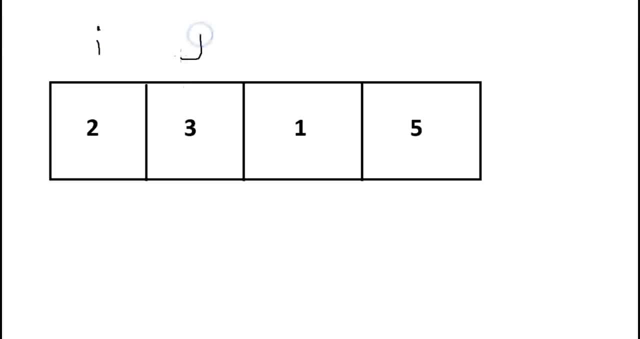 I. So that is going to be the first one which is zero location, And then we have a J, which is going to be the second one, which is going to be I plus one. So right after the is going to be the J And we're going to play, apply actually a nested for loop. So first for loop. 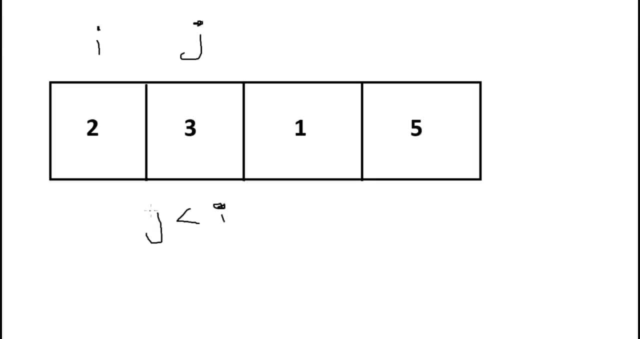 is going to have some condition. So after inside, there's going to be a condition that says J is less than I. So over here, what it means is that the array of that J and the value of that J is less than the value. 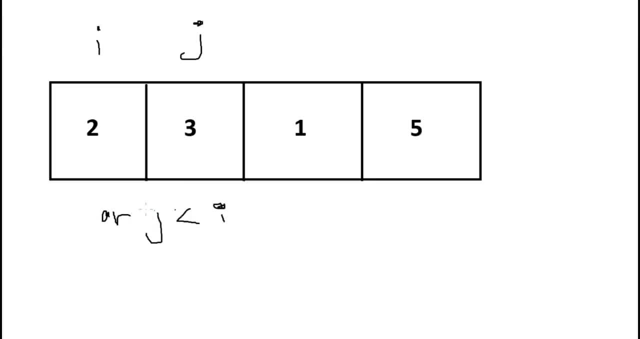 of that I Now that's what I meant by array sub J and less than array sub. So the value of J less than the I value. this is our condition. that's going to be inside of our nested for loop, the internal one, And this is the condition, if it's true, we're going to create a temporary. 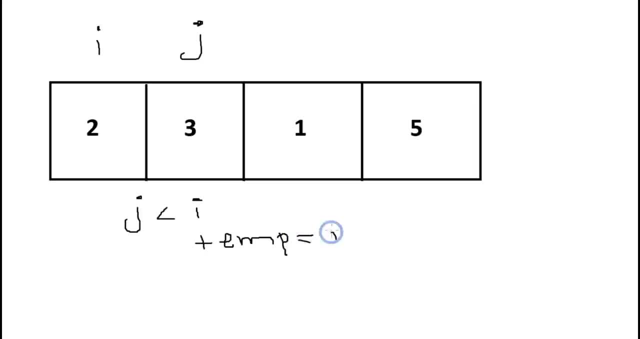 variable and we're going to store the value of I. So whatever is in I, so in this case, what two is in it? so two is going to be stored in temp. So then we're going to swap it using a Swift fame swapping methodology. I is equal. 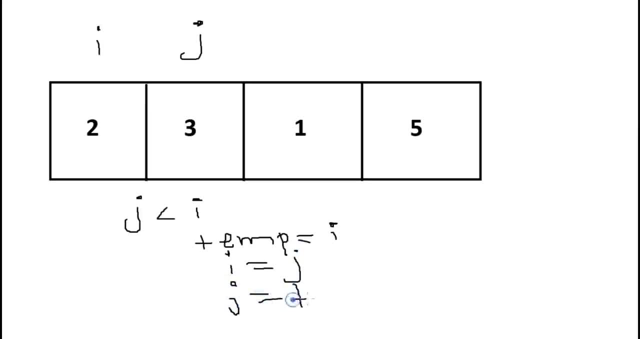 to J and j is equal to temp variable. So whatever the temp value was, it actually was I's value. I's value was two, though that's going to be in J. So actually we just implemented a swap methodology here. So right after that we're going to check in this condition. So 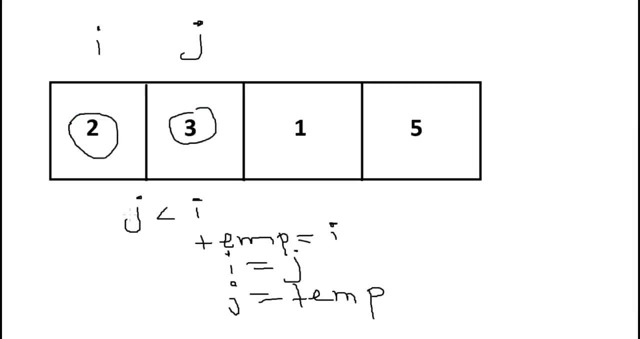 in this case we have two and three, So value of three is actually greater than the value of two and it won't execute. So this is just going to skip the value And we're just going to make our J now increment to the next portion, So we're going to skip this. So I just cross this out. 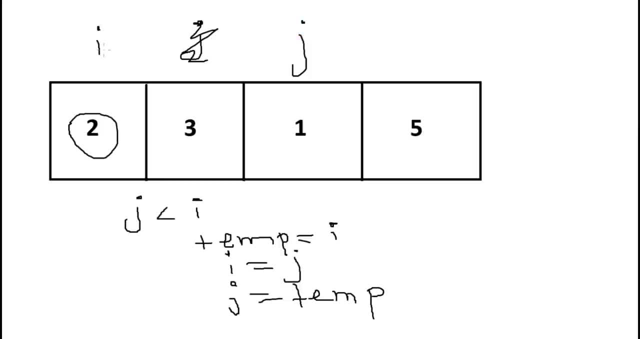 And now I go and put this next pointer over here in J. So now I and J, now you can see that J's value is less. Now we have one and we have comparing with two. So one is less than two. So this is condition is now true. you could see that one and two are going to be located. 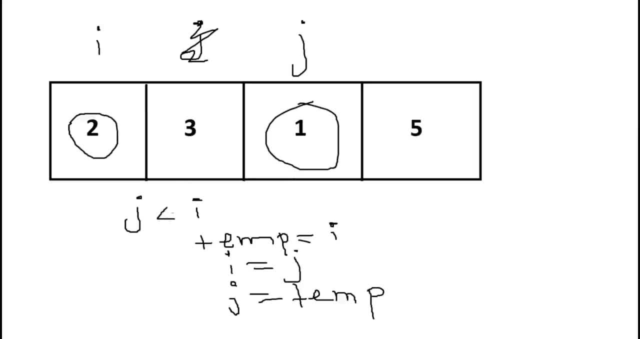 talking about the values And now that the condition is going to be satisfying here. So we're going to look over here that temp is equal to i, and then we have the value which is i. So what is i two? so that's going to be in that temp variable: i is equal to J. Now, J is actually. 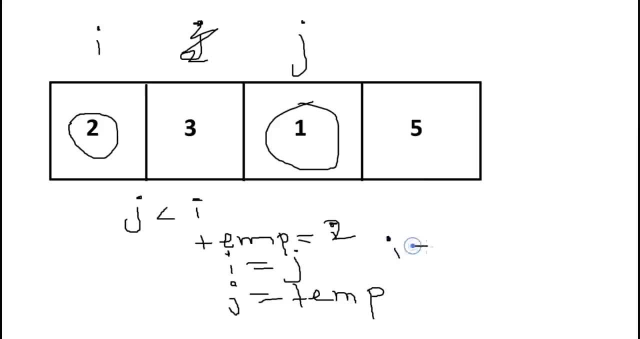 one, So i is equal to one. So we're going to have here: i is equal to the value one. Now, after this, we have J, So J is equal to now the value of temp. Now temp value was actually two, So now you can see that this swapped value. 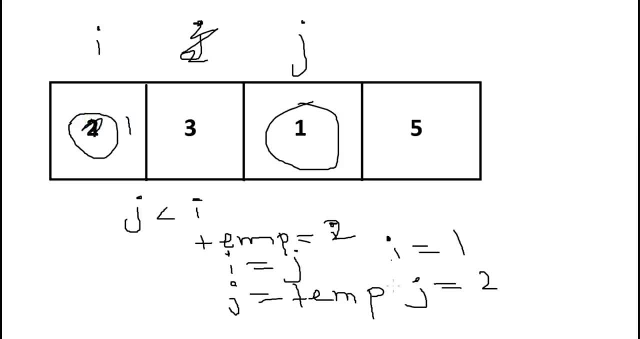 So we have i, which is now one, except for two, now two, And now over here in the J position instead of one. now we have the value of two. Now you can see that swapped out, And now J's value is going to be incremented, So you can see that the index is not no longer going to be here, And 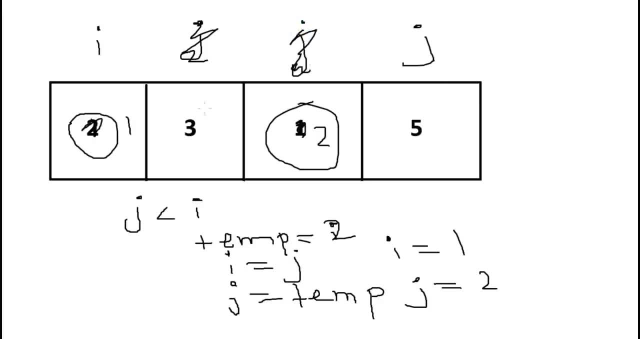 now it's going to be in the fifth, actually the last one, which is the, where the fifth value is, And we're going to be checking again. we're going to say i and J. we'll say J is less than i. Well, no, it's not, J is greater than i. So now this portion of that. 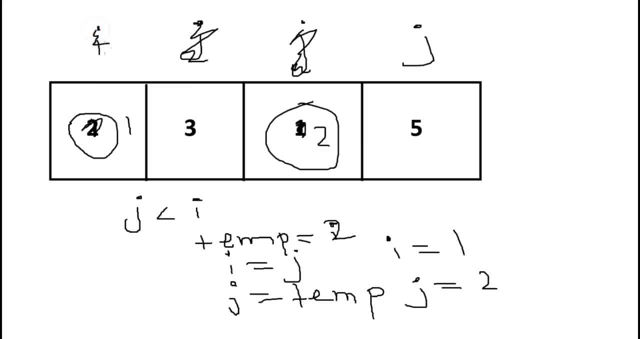 nested for loop will be terminated And what's going to happen now is that i is going to be incremented, So i plus plus, and we're going to have i now plus one, So originally where J was right. So now there, that's where i is going to be, And actually what we see here is that. 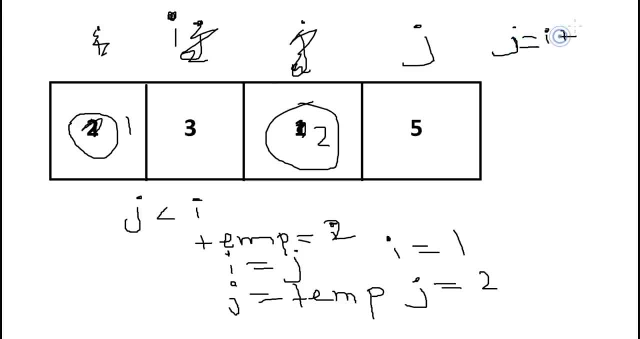 J is always going to be i plus one, like what we mentioned before. this is our sorting algorithm process that we do, So we're going to have i plus one and we're going to have i plus one, so it's just going to be side by side or they're going to be adjacent to each other. 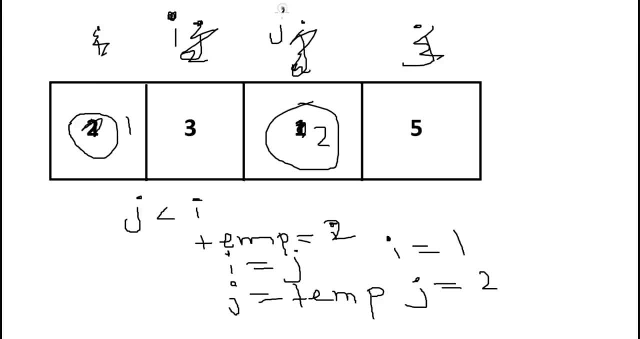 in initially And then after that they're just going to be incrementing. So like, just like J's position. So we have J over here and we have i and J. So if I look over here, we have i, which is: 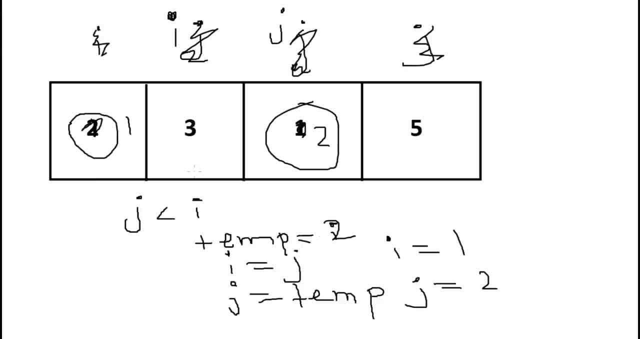 three and J, which is to check the condition. Now, that's true again. So what's going to happen is that J is less than i. that is true And we're going to process this. temp is temp is equal to- now. you could guess what's happening here. Now. temp is equal to the value of i, which is 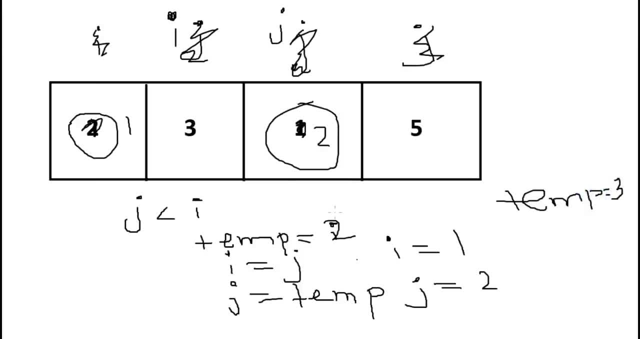 three now. So three is going to be placed here. So there you go, three. And then after that we have: i is equal to now the value of J. J is actually two, So we're just going to have two over here. i is equal to two. And then last one, which is J, is equal to the value of temp. 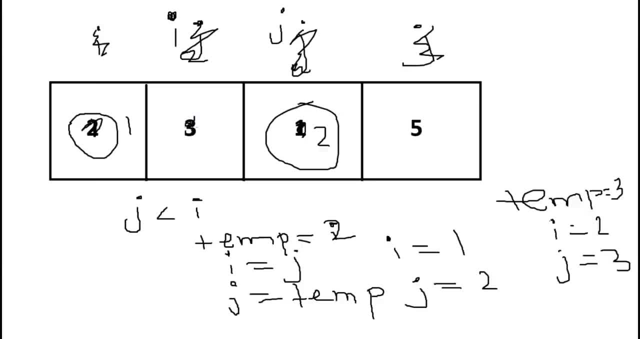 temp was three, So that places over here. So now we just basically swapped it again. So we have, instead of three, we have two over here, And instead of two we have three over here. So you could see now that J is now going to be incremented again to the last one And we 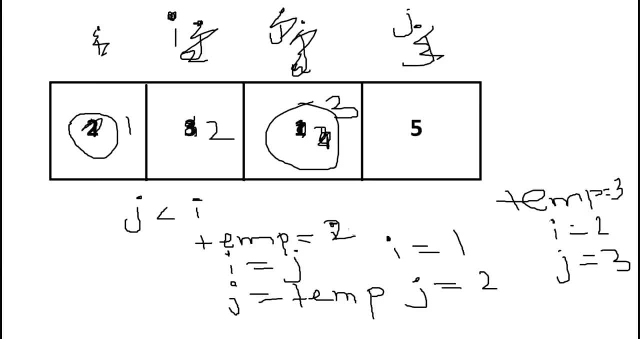 see, i is just in the same exact position And it's going to compare two and five. Well, that condition is not satisfied for this condition. So it's just going to increment that process again, i and J. Now it's going to compare and say three and five. Well, that condition is also not true. 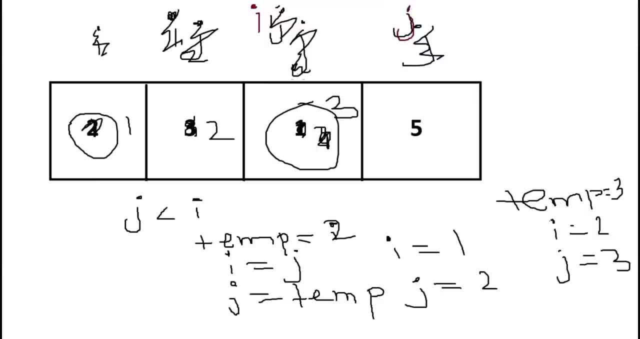 for that while loop to be executed. So now we have this i and J in red, So you see that there's nothing to be changed. So we have actually our algorithm is working And we see that one, two, three and five- you can see one. 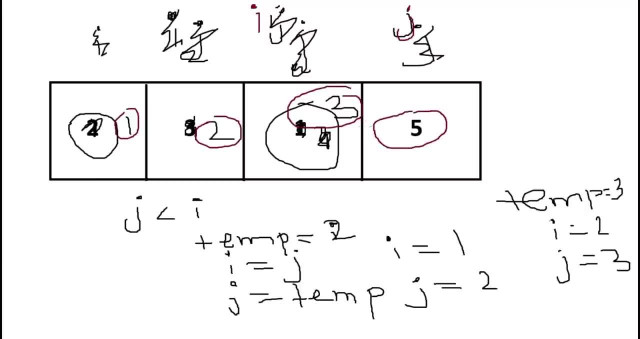 Two, three and five there are in ascending order, And that's how our algorithm was supposed to work. So this visual implementation of this algorithm helped us, And now we could map this into our code. So we're going to be right now typing, So I would encourage you to type along. 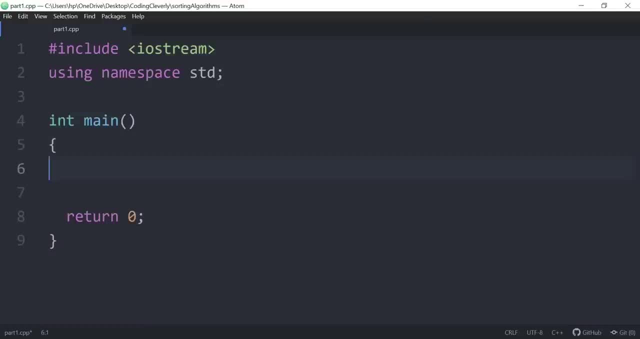 with me. So let's just get things started. Okay, so the thing here is that we're going to have to create an array, And I call it an array And I suppose we want to have a size, So I could define something over here on the top. So I say: 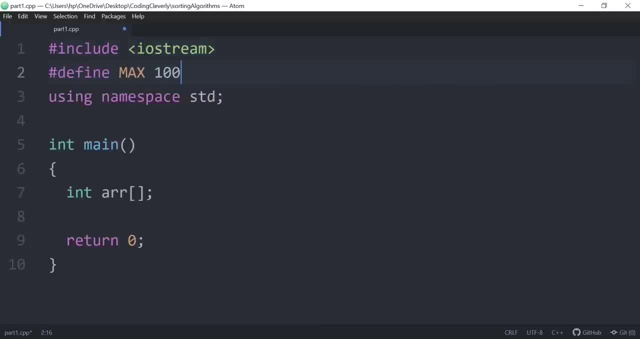 hash define and I say max and I say that's the 100.. Alright, so this is the maximum value. So we just put max here. And what I could say here is that I could ask the user to enter a number, n And. 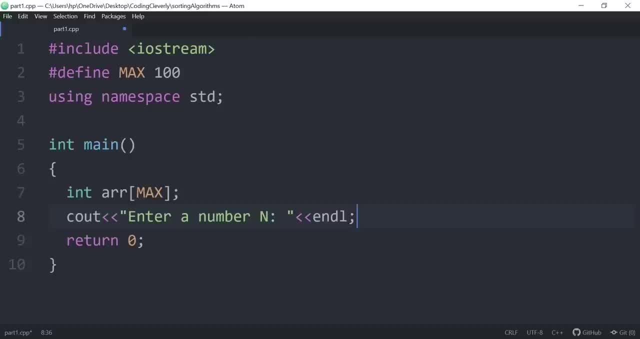 that will be the size, and it should be in between zero to 100.. So it's going to be input and then it's going to be n. now I need to define an n here, So I'm just gonna say integer, And so this is the. 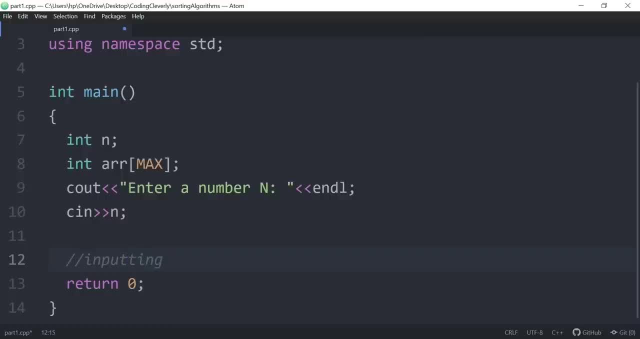 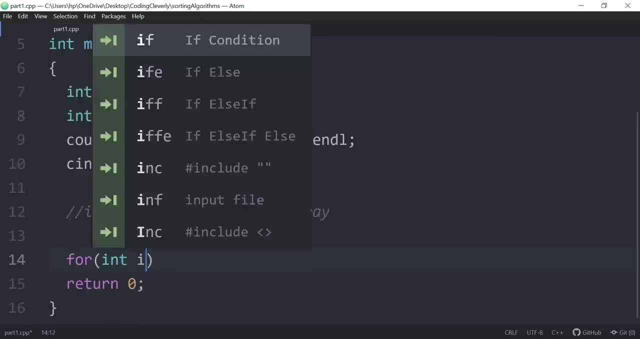 number n and now inputting values in an array. So, inputting values in an array, we're going to do four and we say int, i is equal to zero, i is less than n, and we say i plus plus. really simple, And 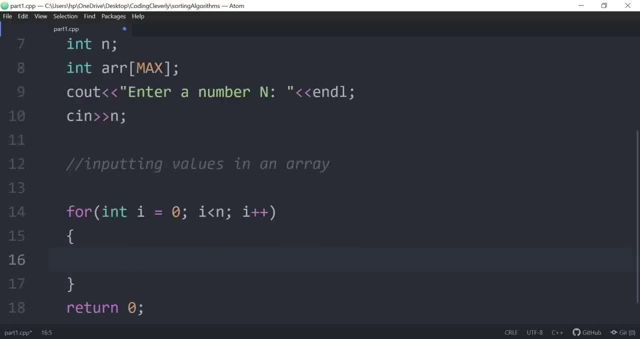 then we have the RAND function that's gonna put values randomly inside of the each indices. So we could say: array sub i and we can say: just the RAND function, and that's it. So this is going to give us an array. We can also say and we can say: and that's it. So this is going to give us an. 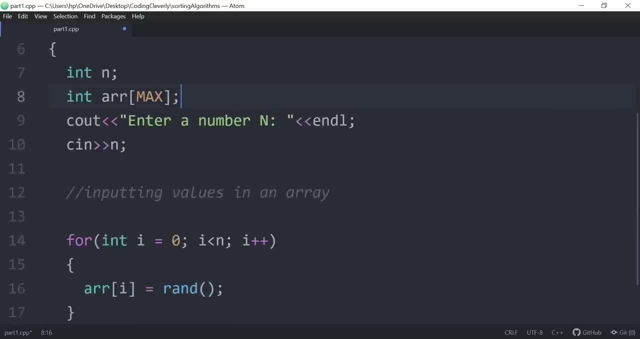 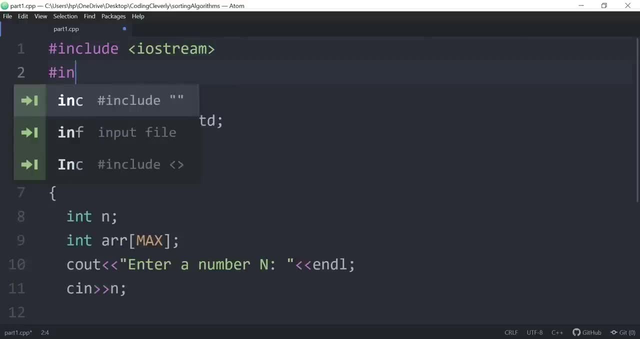 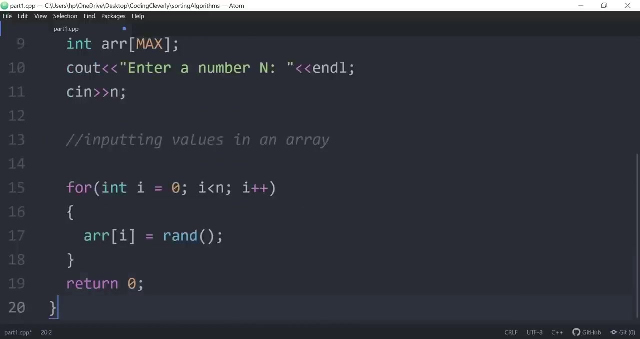 a number between zero to the Rand max, whatever the integer max is. So what we could put here is that we just have to include one more header file for the Rand function. So it's called C standard library. And there you go. So C standard library is done. Now we have values inside of this. 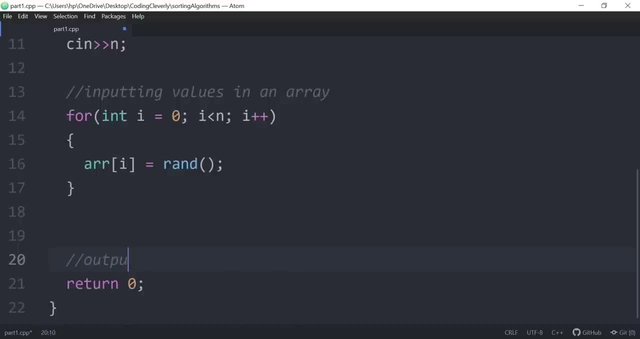 let's output our array, So outputting the unsorted array. so, unsorted array, we could just basically say: for int, I is equal to zero, I is less than n, and then we have I plus, plus, and then we say: 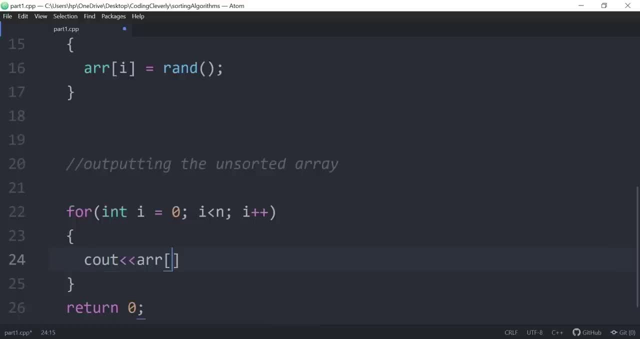 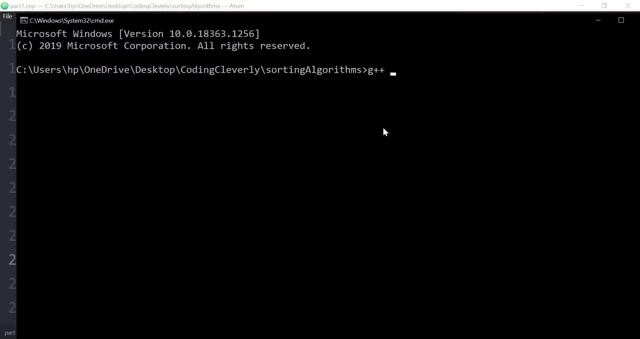 console output array, sub sub i, and we put this space And hopefully we'll get an array. just put an end line right here at the end. And now I save my code. So I'm going to run it using my G plus plus compiler. So over here I'm going to be writing G plus plus my name, which is part. 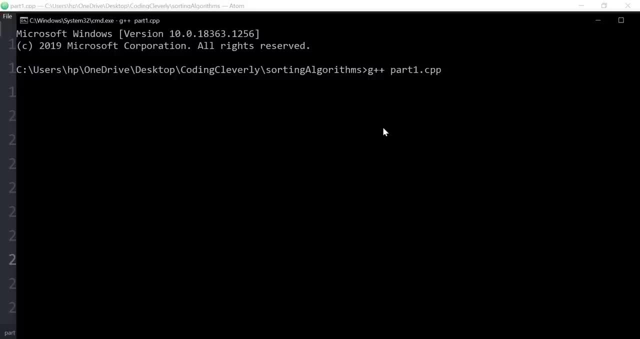 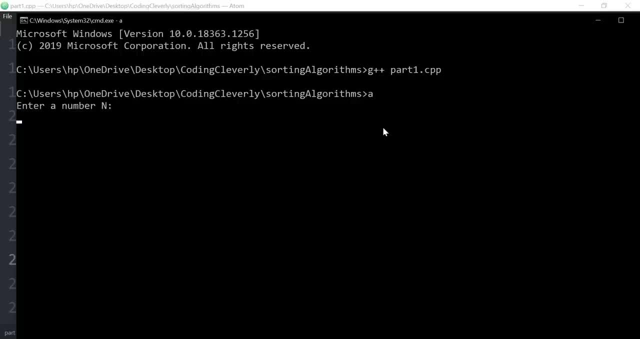 enter a number, n. So basically I could say 10.. Now it's going to give me 10 random numbers for my eight array. So it has 41, this, this and this and all the way to 10.. So you can see that these 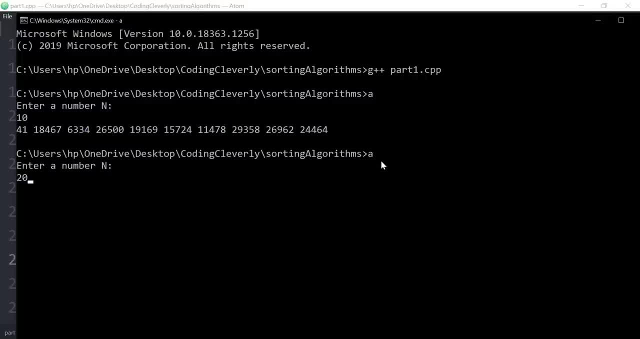 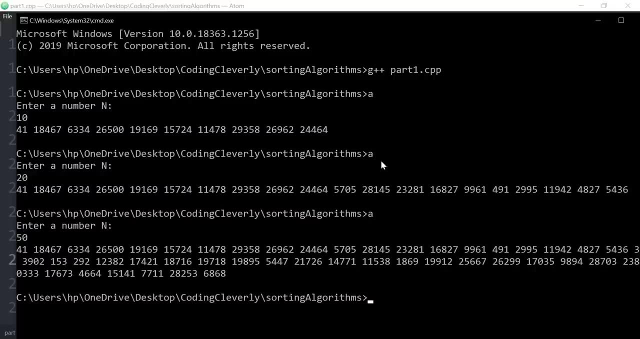 are 10.. Let's run this one more time. And now I'm going to input 20.. Now it's supposed to give me 20 random integers. So now, there you go. How about having 50? now, 50 random integers. Now you got my point over here. it's creating a randomized array. 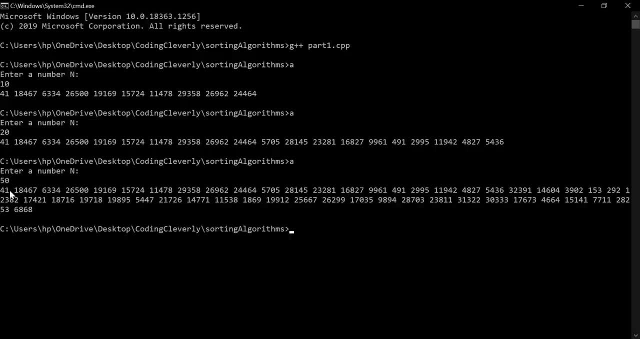 and it's putting some random values. But you could see over here that these are not sorted in any kind of order. They're not in ascending, no, they are in descending, And now that's our job to put that. So we could see 41. And you can see that this is a number that's greater. 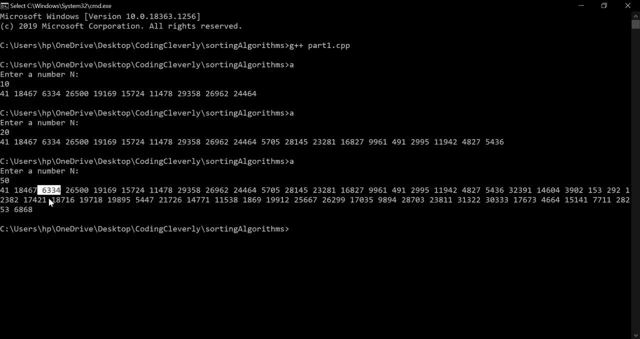 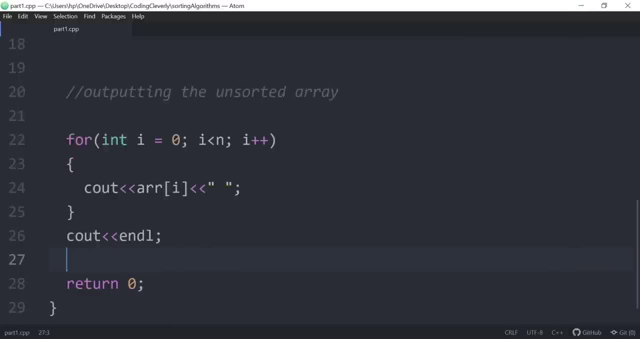 But then after that, you could see a smaller number, And what is this even meaning? So we need a properly managed array. So let's create a properly managed array. So what we can do here is, right after this, let's create a sorting algorithm. So sorting an array. 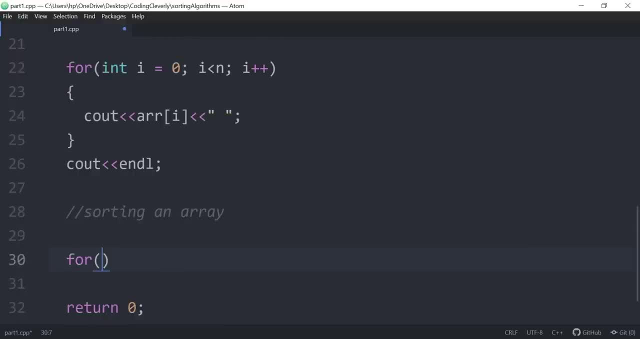 So how are we going to sort this array? First of all, let's go and open a for loop So we could say four into i is equal to zero, i is less than n, And then we say i plus, plus, And then right after, 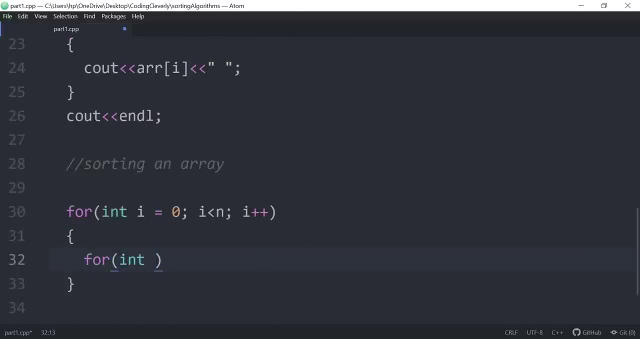 this. we can put another input array. So we could say this: another loop that's going to be nested inside of the beginning one, So it's going to be J. But this is careful, this is the next value after the array. So we're going to say, okay, this is the next value after the array. So we're going. 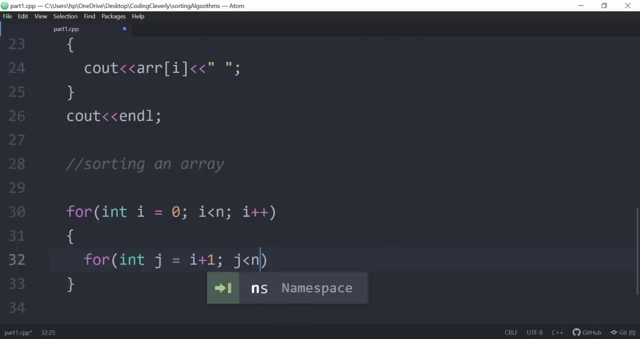 to say: okay, this is the next value after the array. And I'll tell you what's the reason behind this: say j less than n and we say j plus plus. And now inside of this is basically our concept that's going to be applying with array sub j is less than array sub i. Now, what does this mean? 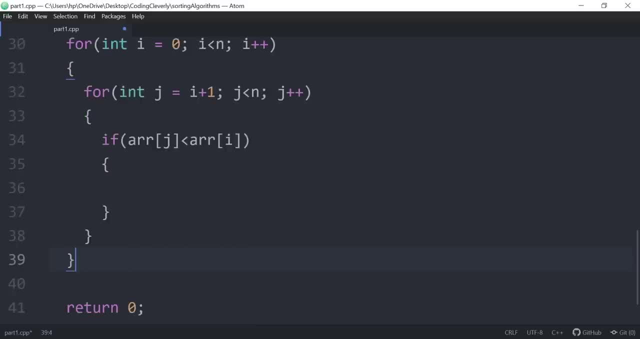 I'll tell you all of this. So suppose we have an array And this says that if a race of j is less than a race of, because, look at this. So this is an array And you will see that it's an order. So 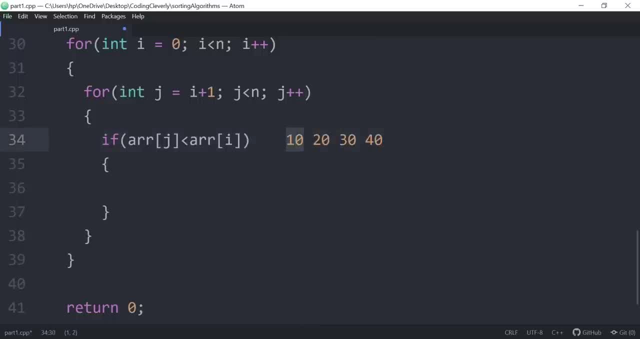 you can see that this is this i value, which is the array sub j. So this is an array sub j And you can see that this is the j which is starting from zero And this is the j which is starting, which is greater than i when one times. So you'd see that j is this and this is i. Now, if I had 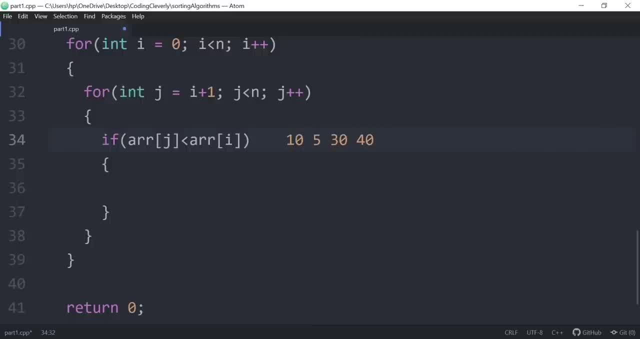 a randomized array. so let's say I had five over here, So you can see that this is not in ascending, it's basically 10.. And then it's five. why is five over here? something bigger should be appearing. So the condition here is that a race sub j is less than array sub i. So meaning if a race of j 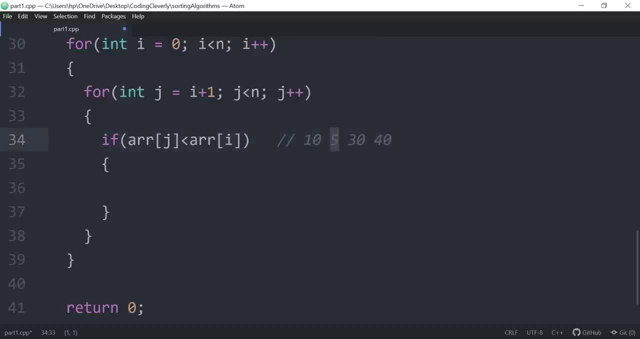 which is this is less than a race of i, And that is the case. Now, what we want to do, we want to swap the values. So what we could do by swapping the values, so five could be over here and the original value. 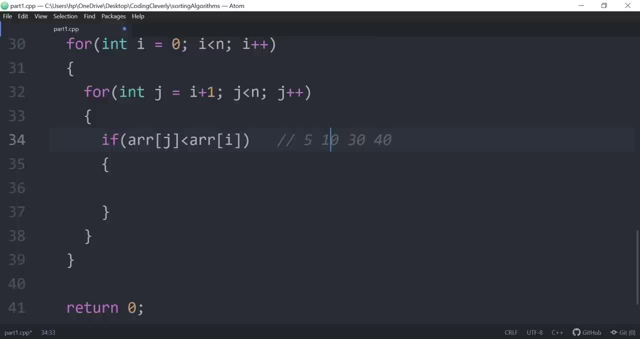 10 should be placed over here. How do we do this? Because 510, 30 and 40 will be then sorted And the thing is that we're going to have to create an input integer, temporary something. So we're going to put that and assign that with i. Now. once we have that assigned with i, now what we could do. 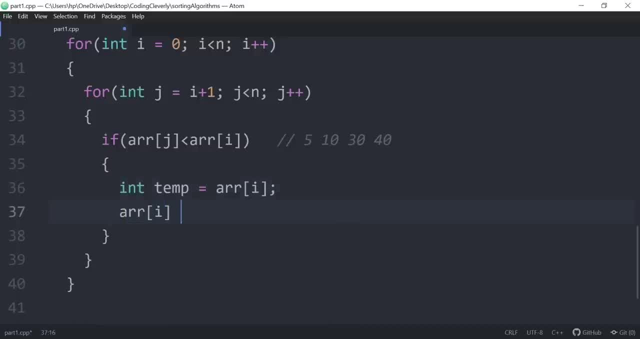 here is that we could change a race of i and we could say to that to erase a day. so we're assigning a race of eyes value with a race of j's value And then we can have a race of j's value And we could. 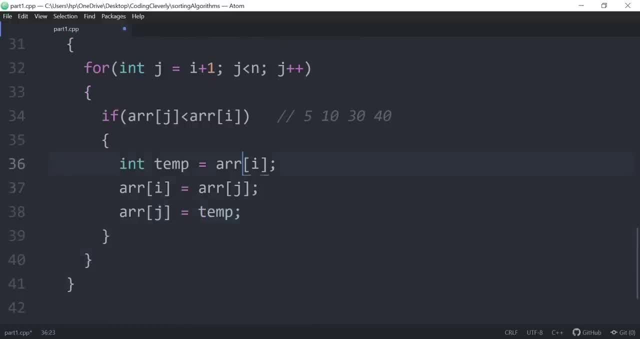 put that as temp value. So this is gonna improvise our array in a sorted fashion And it's going to be in ascending order: ASC, N, D, I, N, G or D? er. So this is going to be in ascending order, So it's. 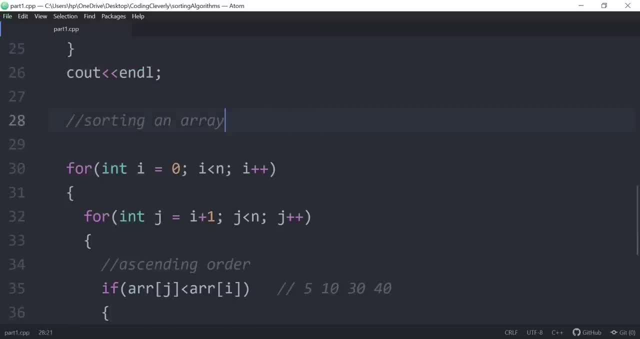 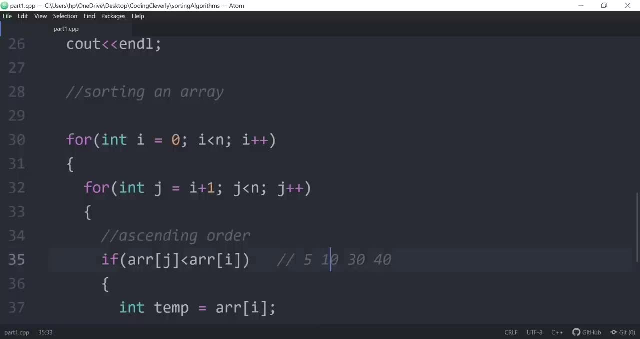 going to check that. it's going to do this. it's going to go into our next iteration, which is going to be: i is equal to one, So plus plus increments to this, so it's going to be this value And then it's going to be checking with this value And it's going to see if this is the case. 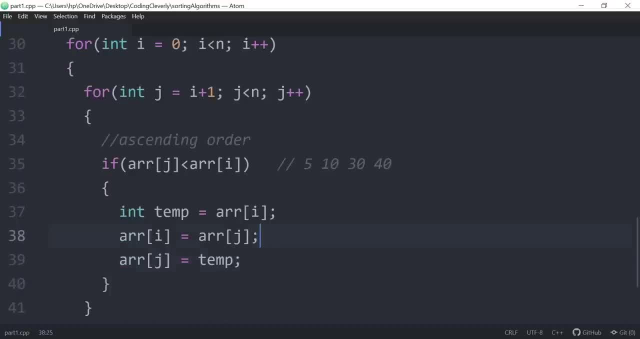 that it's not right. it's going to swap it out. it's just going to next do this next iteration until the array is done examining. So once it's done, you can just break out the loop, And once you're break like you're free. So what's? once you're free, you return. 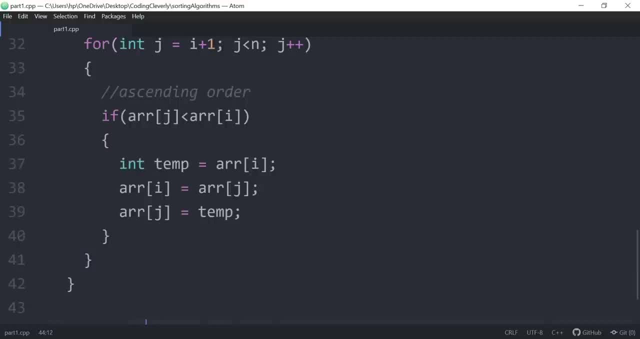 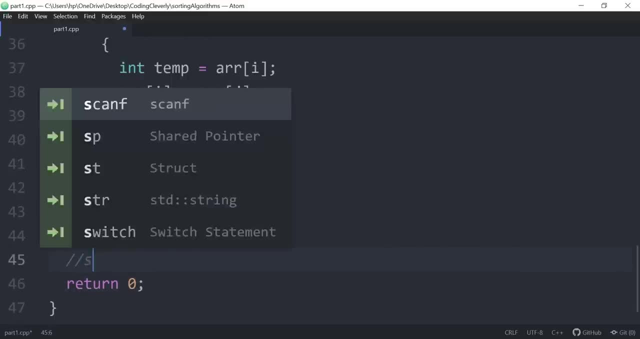 the zero. So this is going to give me my array in ascending order. But now we don't have anything displaying it, So let's display this array. So I'm just going to go right: comment sorting the array. Now we're going to display the, so let's just say the sorted array. So 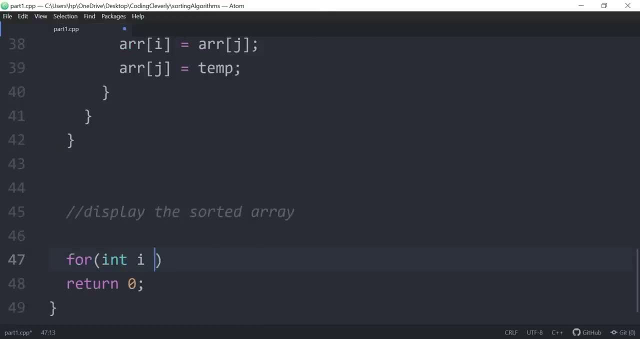 displaying the sorted array. we just do a basic for loop: i is equal to zero, I'm gonna say i less than n, and then we say i plus plus, And then over here which we could add is basically console output, and we say array sub i and 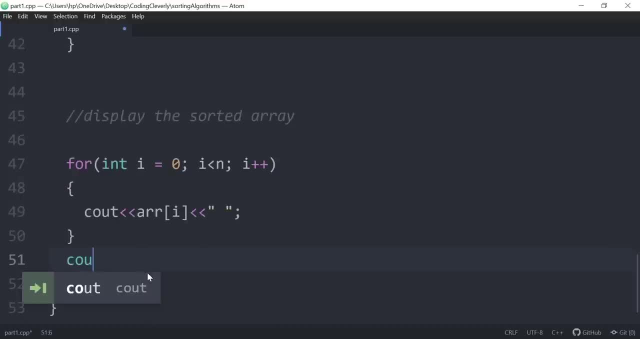 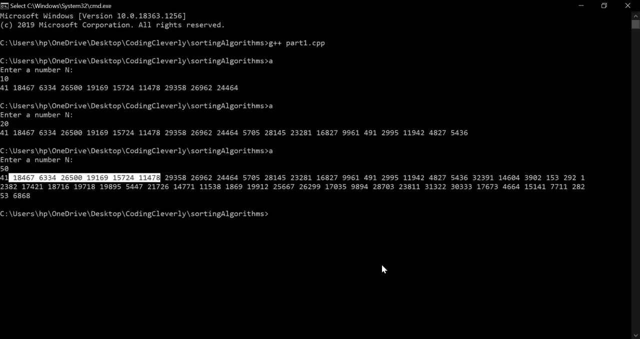 then we say this: And now let's just put an end line right here. Now let's run the code. So basically go back to our G plus plus compiler And we're going to be running our code, But first of all let's compile it. 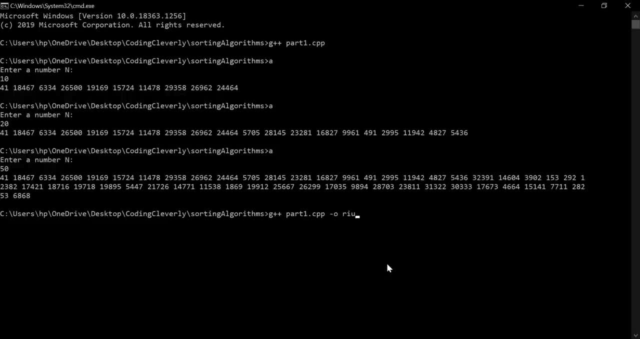 And I'm just going to give it a name. And I'm just going to give it a name, And I'm going to give it a hyphen o flag to indicate that this is a new executable, And I'm just going to call it run. So I'm going to hit the compiling button. compilation is successful. 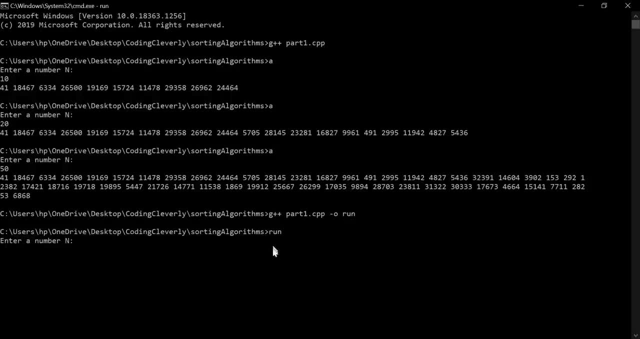 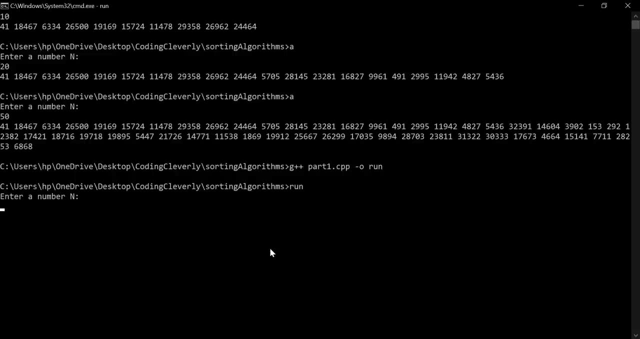 Now we're just going to run. So now you can see: enter a number n. So enter a number n, meaning that let's just enter some random number and it's going to create an array with some randomized values in each indices, So let's have 20.. Now these are 20 random numbers. 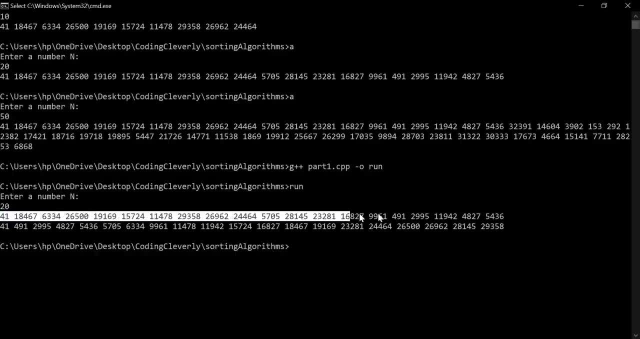 you will see over here For 2041.. And all of this which is unsorted. it just in random order And then after that it sorts it And you can see my sorting algorithm does the trick and sorts them in ascending. 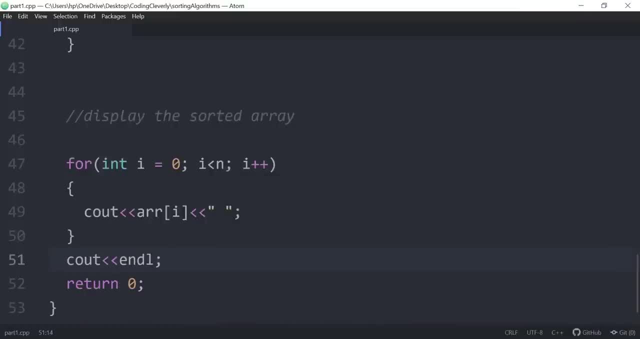 order. That's pretty amazing. Okay, now let's do one other thing: for us to have a descending order fashion. One other thing I want to do here is that I want to tell that this is going to be the sort of: so I could just write a console output and I'd say: sorted, So sorted. 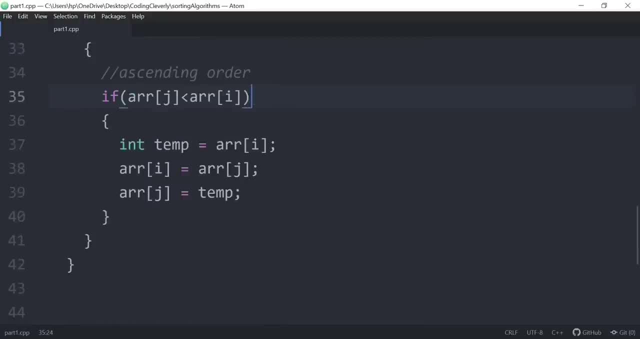 and right here, Right here, displaying the sorted array, And other thing that I want to do is I just want to show you how descending work. So this less than sign, which is a race of J less than a race of I, will just be turned into a race of J greater than a race of I. so if 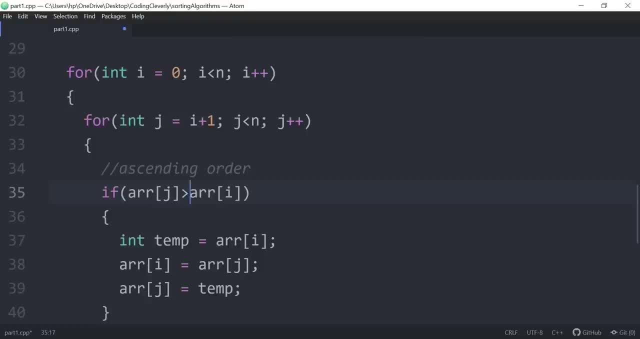 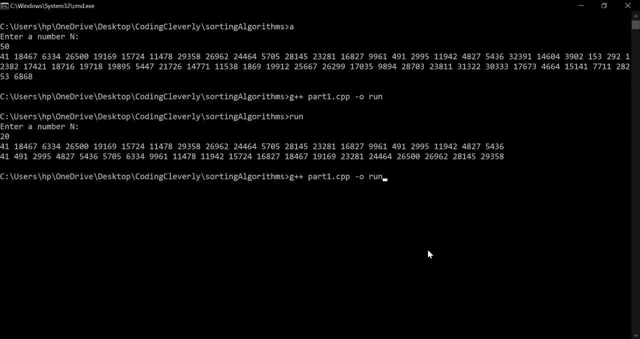 it's greater, then swap it. So that's basically descending order. So I'm just going to change this ascending to de, s, C and di ng. So this is now going to be in descending order. going to run again. So I'm just going to compile this basically And then we're going to run it. 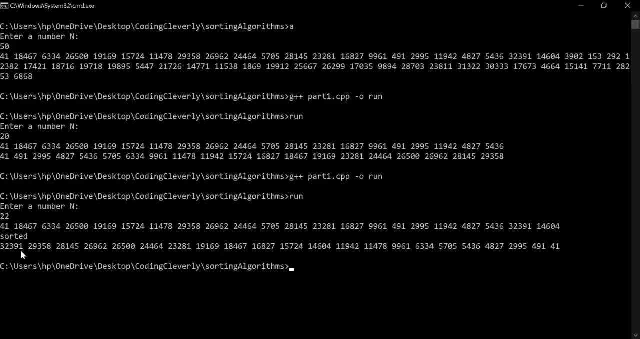 And now let's have a value like 22.. Now you have these values, which are 41,, and all of this in random order, And then after that you call the sorted, basically prompted out on the terminal screen, And then after that you sort them in descending order fashion And look how awesome. 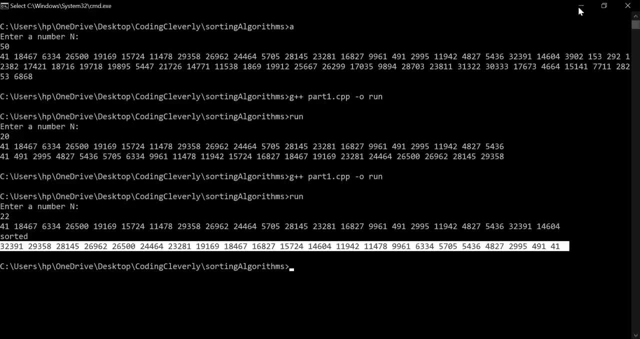 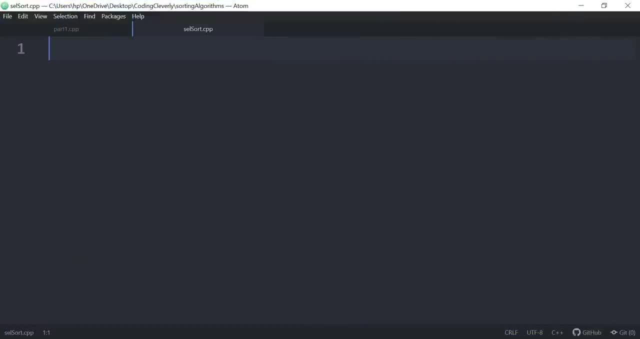 that took. So that's it with this one, And now let's continue with the other sorting algorithms. So the next sorting algorithm is called the selection sort, one of the most common and most famous, well known sorting algorithms in the world. So how we're going to implement this is basically: 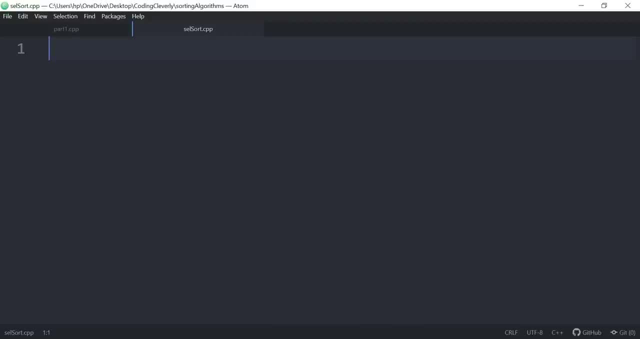 first type along And we're going to be explaining side by side as well as going to give a brief explanation at the end. So just keep on typing along with me. So hash include: we're going to have input output string, And then we're going to have input output string, And then we're going to. 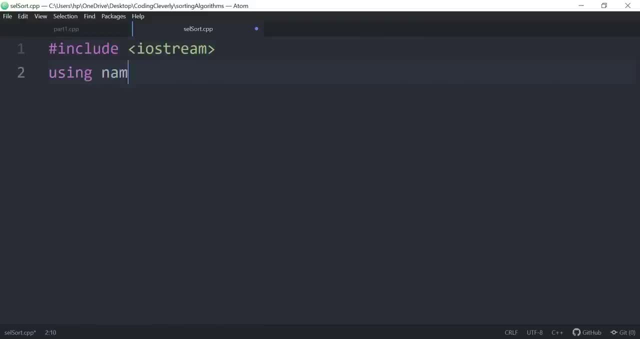 have using namespace standard, and then we also have integer main And we also have the return zero. Now what we're going to do here is basically: first we're going to create a swap function, So what I'm going to be implementing is basically a swap function, So void, and then we have swap. 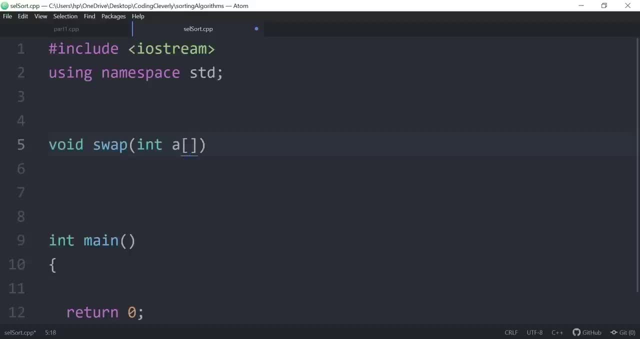 And then we have basically an array we're going to have and it's going to be swapping, So I'm going to show you that it's going to have an x, and then we're going to have an y, and then we're. 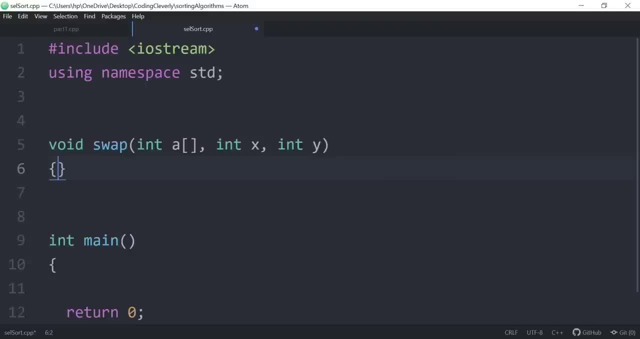 going to have an X value and it's going to have a y value. So it's going to be implementing that famous swap function process that we've been doing. So what's it going to be doing is basically, integer temp is going to be having a sub x as the first value. So A sub x. so A sub x is going to be. 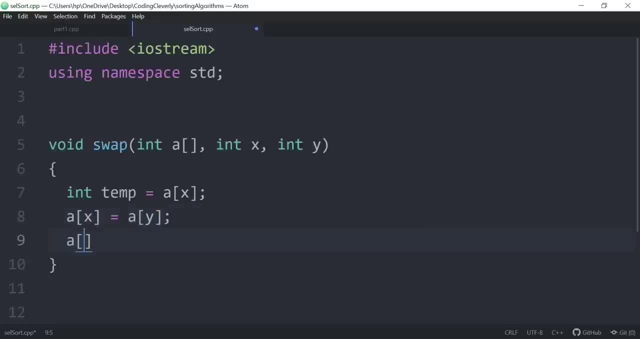 equal to a sub Y. And then when I have, is a sub y equals to the temp variables. So, and that's how we swap something. So suppose, have an array inside of it and we just call it an array And we're going to have some values to it. 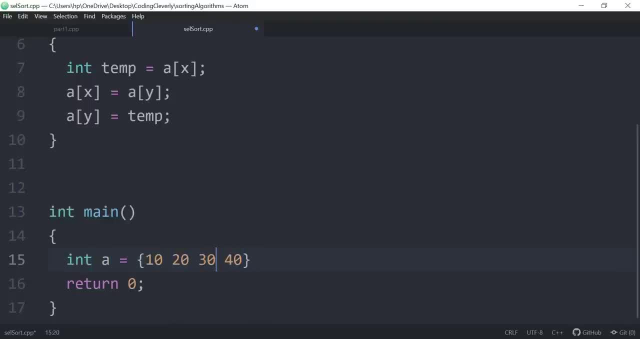 So let's say some random values And what we want to do is basically, we want to swap the process over here. If we have some random values, they're not matching and we want to swap them, we could use a swap function like just we did in the basic algorithm in the beginning. what we did ascending. 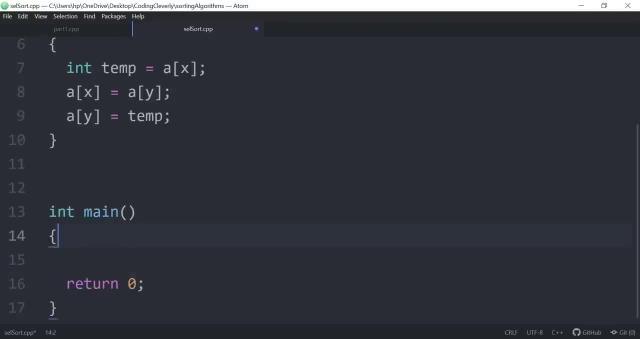 order. So basically we're implementing selection sort. So we created our first function, which is swap. The second function that we're going to be doing is basically the selection sort. So how this is going to go is basically we're going to have a void. 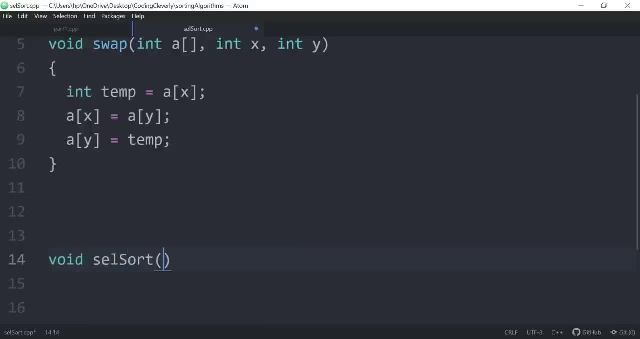 And we're going to call this as a selection sort, And it's going to have two input parameters. First one is going to be the array And the second one is basically going to be the size of the array. Now, inside of this is going to have the location index, which is zero. it's going to always start. 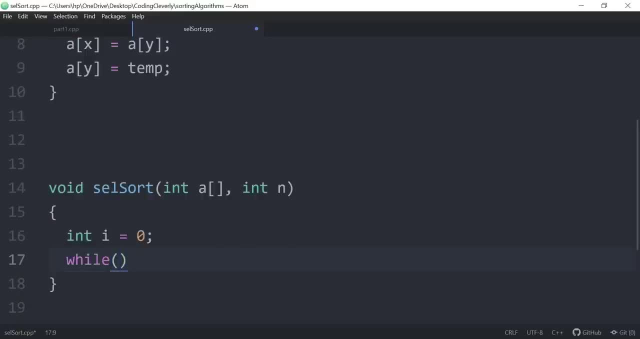 from zero array, start from zero, just that. And now, after that, it's going to loop through this. So it's going to be, I let's say, than n minus one. we're going to loop to the last set, the last element. So n minus one is the last. 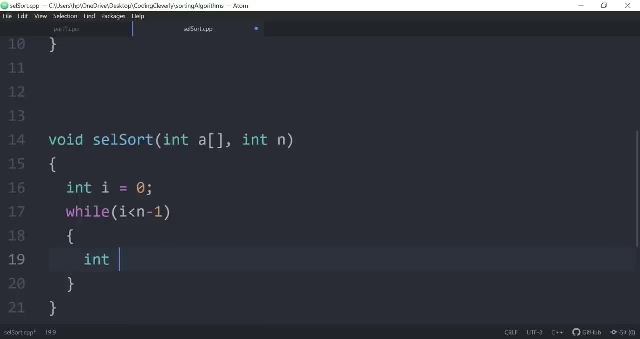 element, And then we're going to have to find the value that should be smaller than the value that we're specifying as i zero, and it should be like swapping the function. So we're going to have to indicate one j over here. So it's going to be called and we're going to use another function. 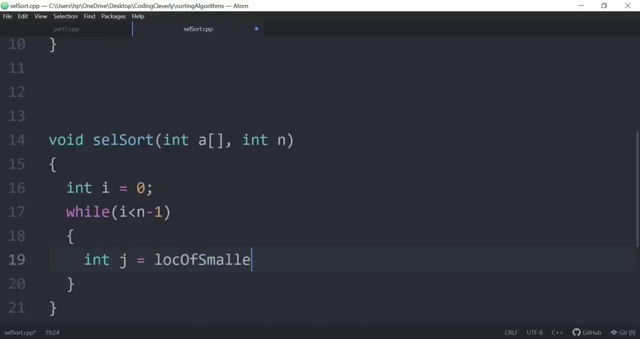 which is going to be called location of smallest. And don't worry, I'm going to be teaching what this is. So basically, we're gonna have a sub i and we're gonna have n minus one, So we're just gonna have three input parameters here. we're gonna have the array passed in. 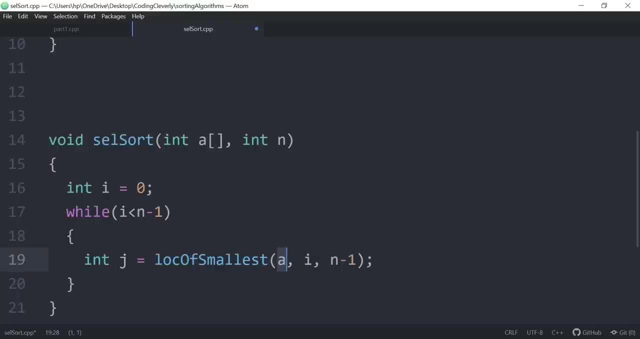 and you know this is passed by reference, So it's always going to be the same array, no matter where you're going. And then we have i, which is going to be the current location. it's always going to be incrementing And it's going to be zero over here. it's going to be 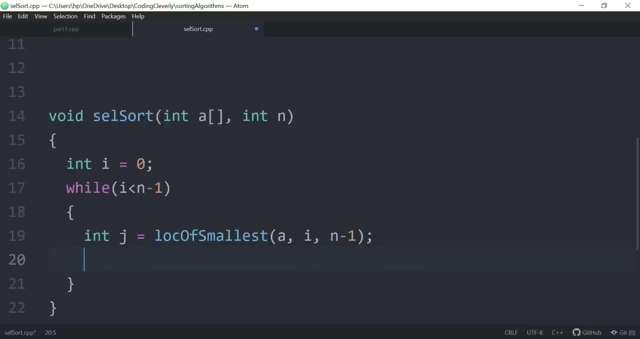 changing And over here is the ending point. So that's the last one And the last element. so swap is going to be implemented here and it's going to have three input parameters, just like we did before. So going to have the array, which is small a, and then it's going to have the size of the eye. 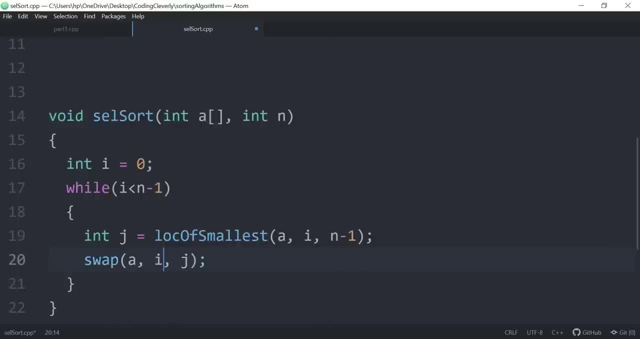 and it's going to have this J, So basically I, which is going to be the index, so it's going to be the first element and the second element- and wants to swap them. So it's going to be implementing this swap function and it's going to be incrementing I plus plus here. So this is how. 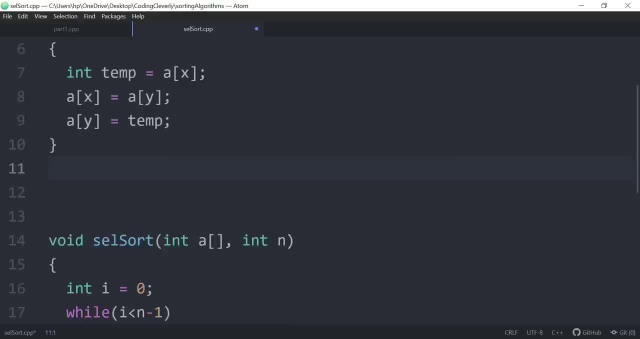 it's going to be doing now we need here is the location of smallest function. So let's just make it over right here. So what we're going to do here in the location of smallest is basically have a return type of int, because it's going to be returning a value of J, So you can see that j is. 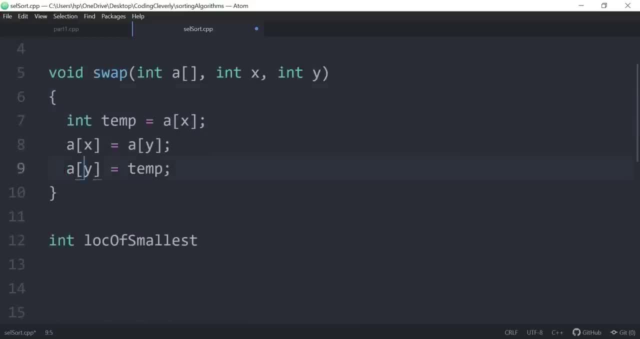 integer, so it needs a return type of int. So over here, location of smallest, let's have some input parameters. The first input parameter is the array And the second parameter is the s. And this third input parameter is the ending point, And you might be asking why I did this And you 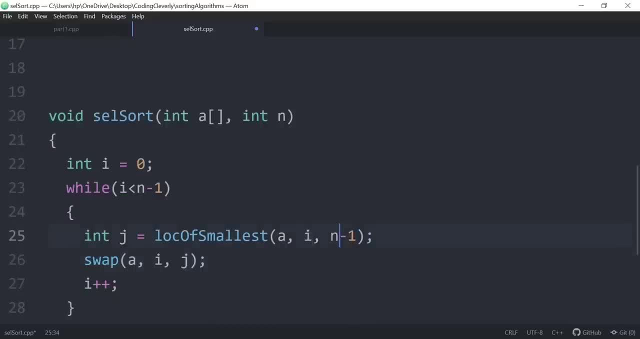 can see over here that the starting point is going to be I, the ending point is going to be n minus one. So it's always going to be checking at the end. So it's going to be looping through this hole array and trying to find the smallest and when it's, it finds the smallest from I and 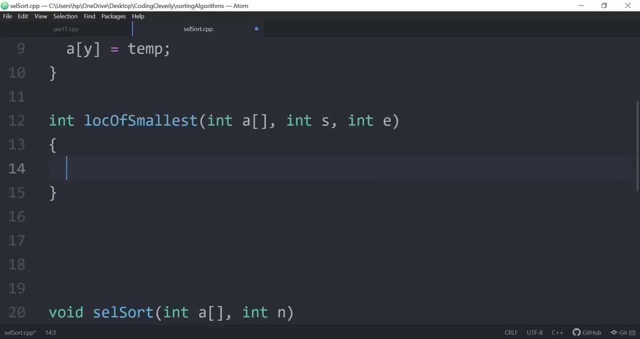 then it's going to swap the value using the swap function And that's how we're going to be implementing this selection sort algorithm. So if I'm going to create an eye over here, I'm just going to create intermediate or intermediary variables. one is going to be: is equal to: 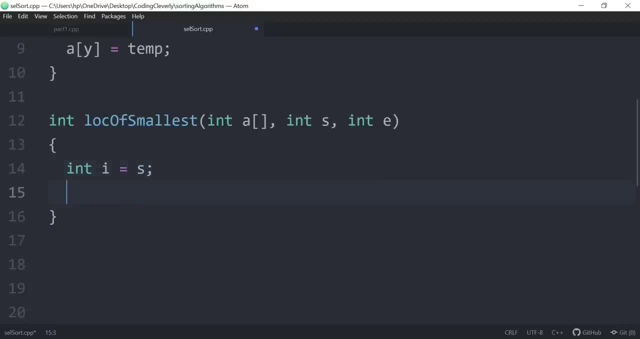 s so is. so I is going to be as the starting point, and then we're going to have j, which is going to equal to basically i, not s. So we're going to implement it and we're going to say: whatever I is, that's going to be one j and I over here is the starting point, And 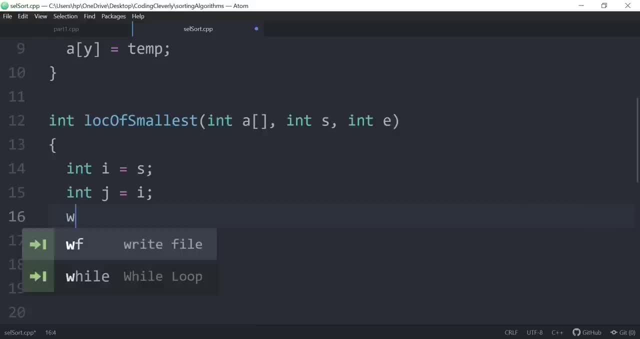 then what we'll do here is that basically, we're going to have a loop again. So, while we're going to have i less than equal to E, which is the ending point, Now if a s, and then we have a sub i, which is the first element, if that is less than a sub j, if we find some. 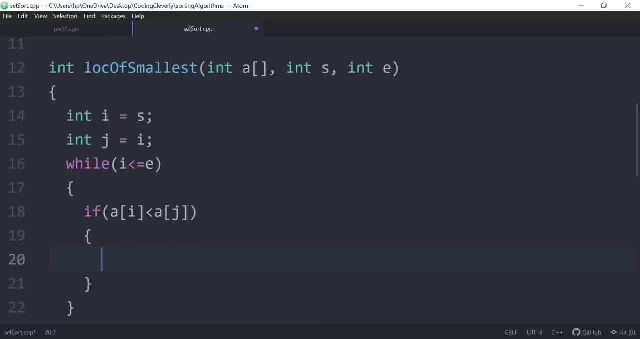 kind of thing that is greater, so a sub j is greater. So we would say: is j is equal to i just want to swap right, we want to locate it, And then after that what we want to do is basically increment it using i plus one right, so that's. 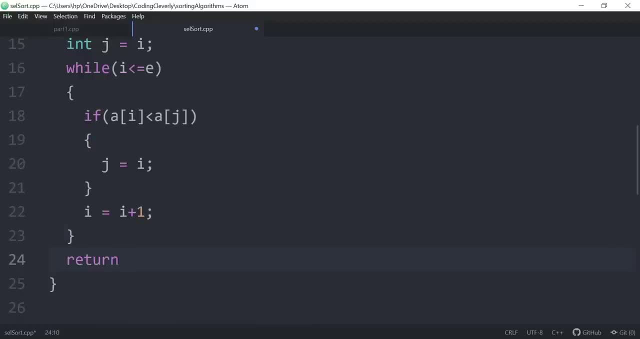 going to be incremented And then we're going to return the value of j And don't worry, I'm going to be explaining this through a graphical representation. So you know this is how it's done. So we have our three functions: we have a swap function And we have a location. 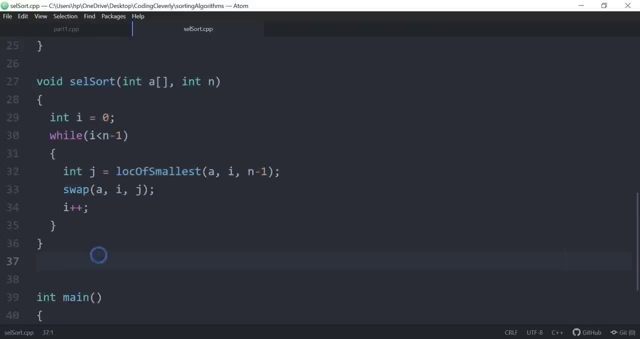 of smallest function And we also have a selection sort function. let's create a display function to display the contents of the array. So it's going to be called display, it's going to have an integer array And it's going to have a size of the array which is n And. 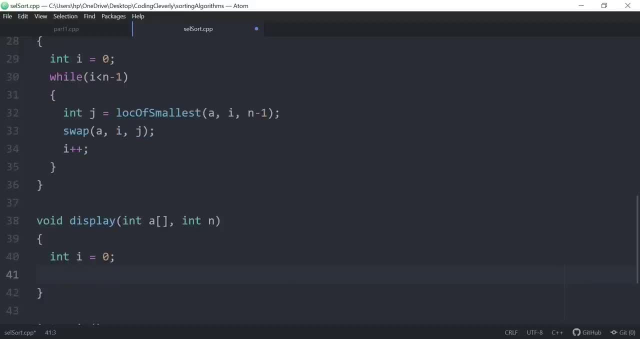 what's it going to do here is basically it's going to start from zero, And what's how it's going to be implementing is basically while the eye is less than n, and then we're going to be displaying the contents of the array by using a sub i And we're going to have 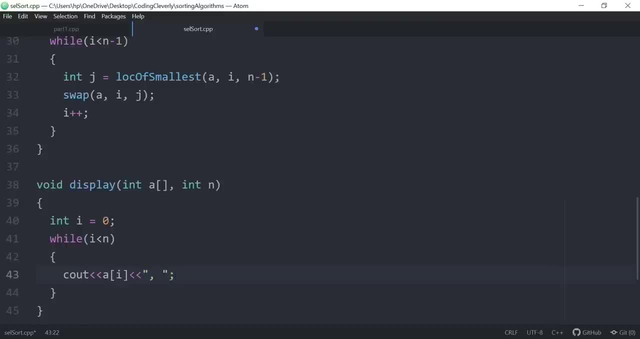 the double coach over here which is space and just going to. it's going to keep on listing them out And it's going to print an end line over here just to make the format a little more prettier. So right after that, what we'll do is basically have the array over here specified. let's. 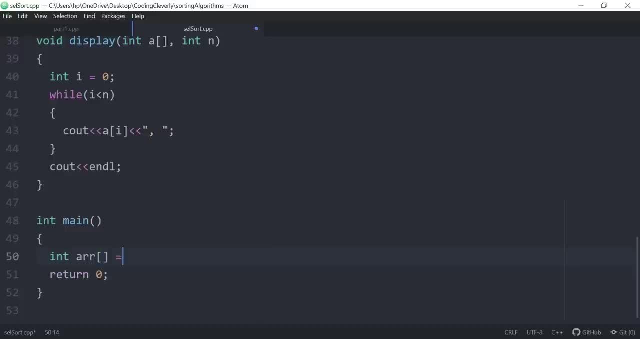 just create an array which is going to be called ARR And it's going to have some random values. So it's going to have 102, 12, I'm just giving random values over here. It's just in random format. needs to be sorted using my selection sort function. So I'm just going. 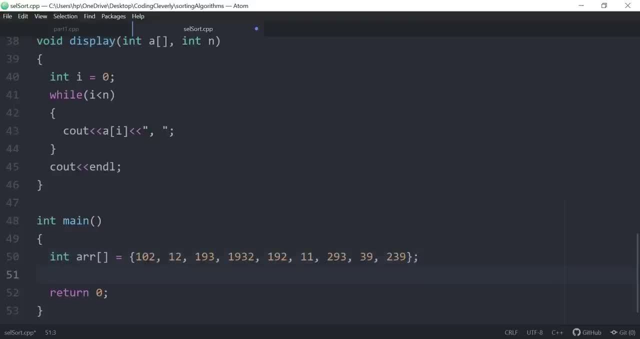 to pass this in. So you can see that this is random. And now what I'm going to do is basically calculate the size. How to calculate the size? one of the process I can do is basically the size of operator. size of operator is going to pass in and it's going to have the array and then it's going. 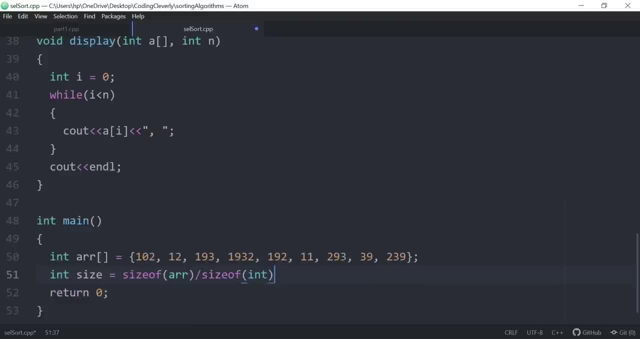 to have the size of basically the integer variable. So basically you will see that this is the data type and it's going to be, for the array is basically the whole thing. So we'll see 1234567 and eight and nine, nine multiplied by four, which is basically 36.. 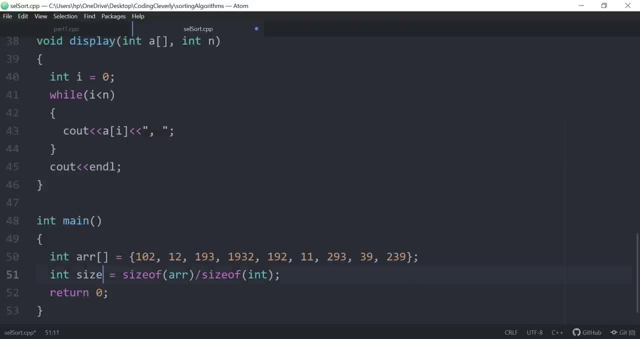 And now 36 will be basically divided by the integer, which is going to be four. So 36 divided by four is going to give you the value which is nine. So nine is going to be the answer right here. So once this is the size, I just comment over here and say: size equal to nine, What we want. 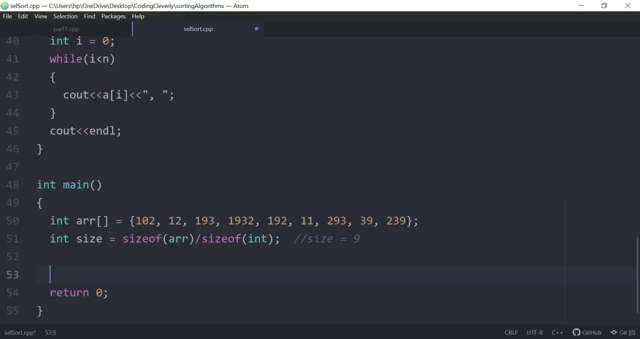 to do here is basically we want to implement our selection sort, But first of all let's just display it. So let's just display and we're just going to pass in the variable and the size And then we're going to automatically display, because it's a void function and its purpose 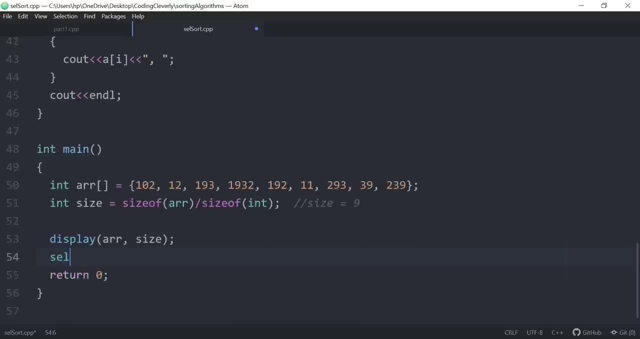 is to display it, And then right after that, let's just call our selection sort a function, and it's going to ask for array and also a size, And then after that, we'll just display our selection sorted array using array, and then we have size. So once I do this, I'll 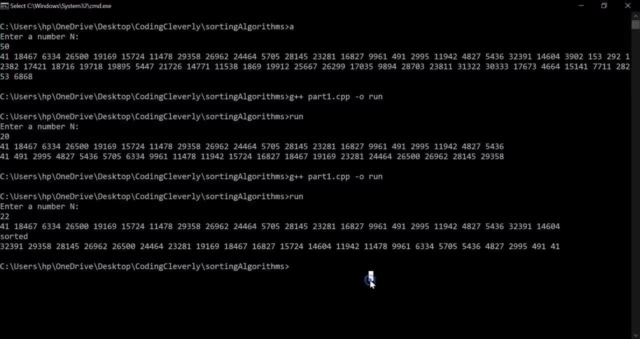 just execute and run. and so basically, let me go in my terminal screen over here. I'm going to write G plus plus I'm going to use the selection sort dot, cpp, And or. we know that by default it's going to be. 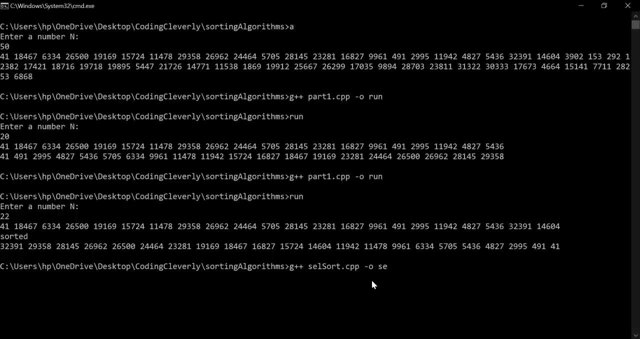 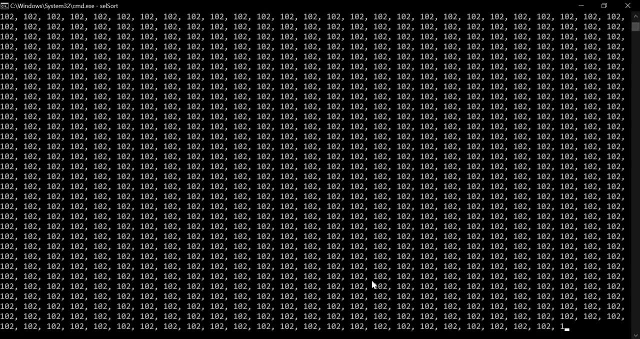 a. So I'm just going to run it and I'm going to say, oh, and I'm going to say selection sort. So now it's compiled, And now let's run it. So selection sort. Now you can see, over here we have some random stuff. what's going on? Okay, so something went wrong. Control. 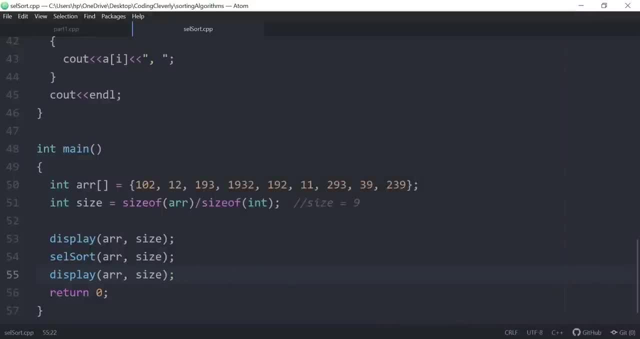 T to break the code. something went wrong in this code And let's just check what it's wrong. What's wrong in this? So we have i less than n and we have it's incrementing. So this is processes Okay and minus one is okay. 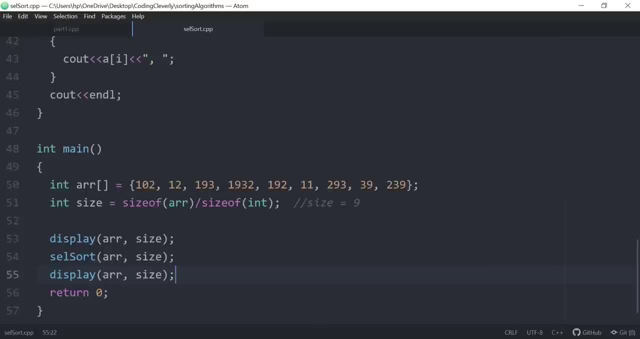 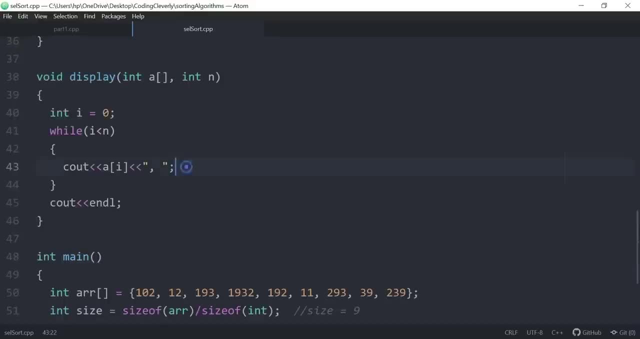 There's some infinite loop that's been created using selection, sort array and then size, And so let's just look over here. Okay, so I forgot to increment this. i plus plus. So just right here I had to increment, and now it's going to be working. So, basically, we're 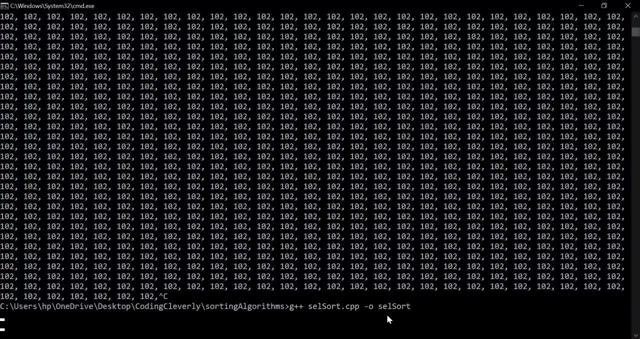 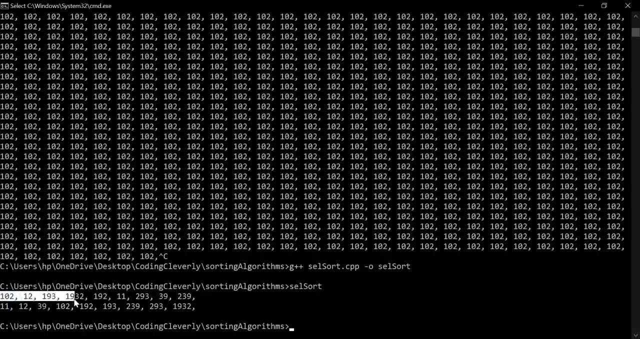 done that And let's just run this code once again: selection sort. And now let's call this and look at that. We had this array which was unsorted, which is 102, 12193, 19,, whatever, 32.. 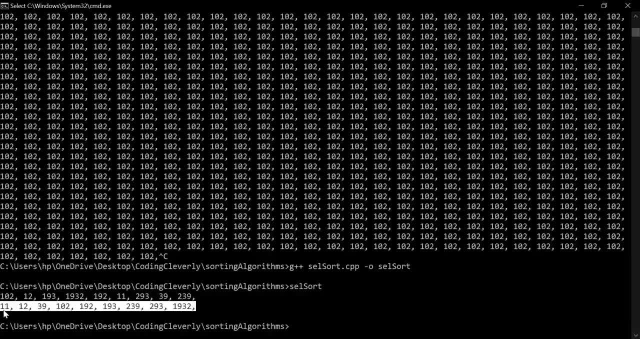 What we did is pass in the selection sort and it's sorted the array for us in 11, 1239 in ascending order. Now, ascending orders that like if you have the same value, it could be equal or it has to be greater. So, just in case, if I have a value like 11 and 11,- 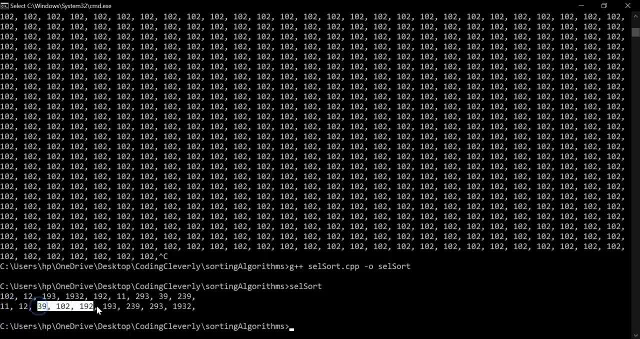 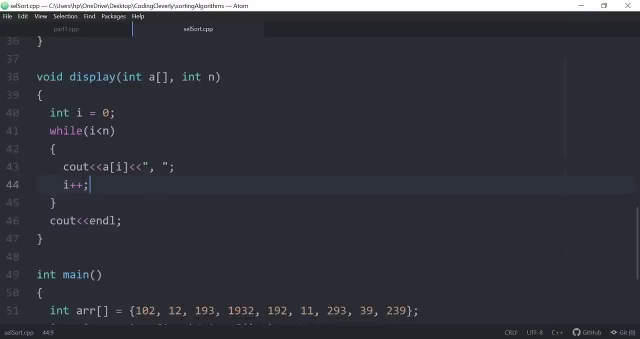 they're going to be in the same adjacent locations And then after that it could be a bigger value. So that's sorted in selection sort. I really hope you enjoyed and you understood. So what I want to do is one other thing is basically show you how the implementation 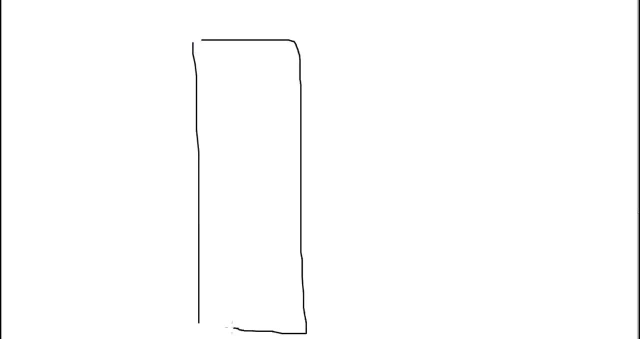 is done. So suppose that the arrays sorted like this in the memory, So we have some kind of indices, So we have like five and we have four, and we have three, we have seven, we have nine, So we want to sort this in ascending order. So what, we can do it by default with selection. 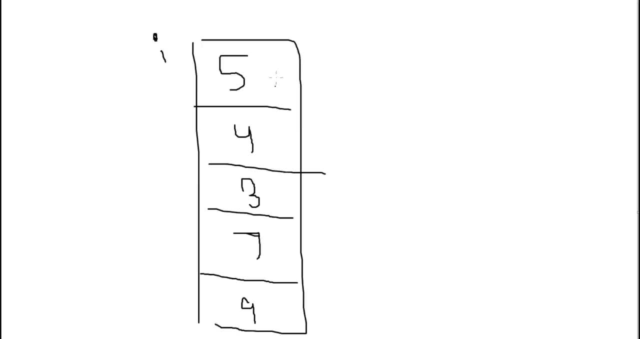 sort and does is that it's sort makes this I as the index of zero and it will check for J. So what my process here is like, that location of smallest will be called. So I'm going to do that And you can see in my code, which is basically in here. So I'm just going. 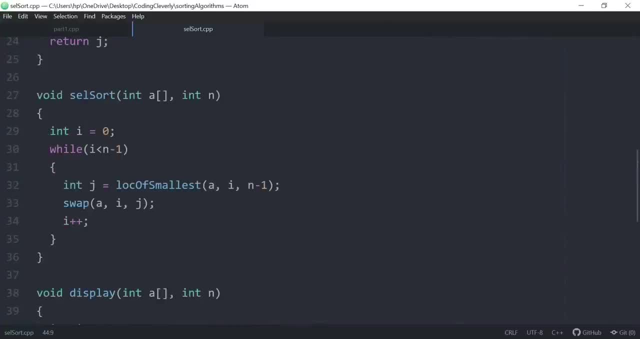 to show you over here. what I see here is that the location of i, zero, and then while is not less than n minus one, the last element. what we do is we get the J and we put that in the location of smallest passing a. we have the I variable, which is basically going: 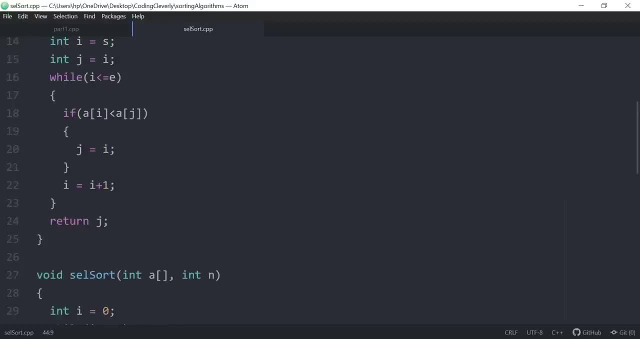 to be zero and n minus one, which is the last element, and it's going to be in the location of smallest. So location of smallest is going to locate for the variable which is going to be this smallest one, even I. less than equal to E. if it's less than or equal to. 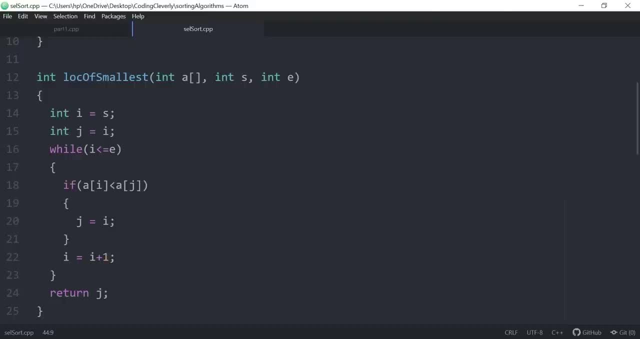 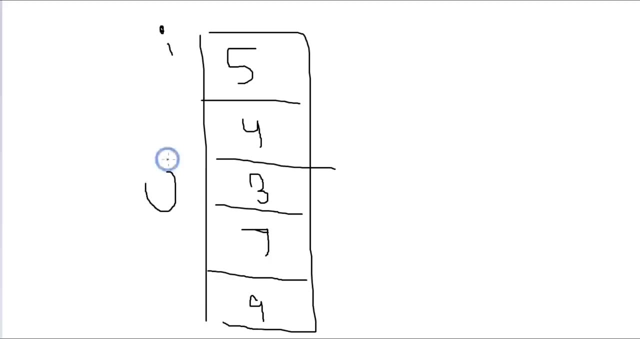 So if it finds it, it's going to sort that as J And it's going to return that value. So you can see: what is happening is that it finds the smallest. so you see that the smallest here is three. So J is going to be pointing here And then it's going to be applying that. 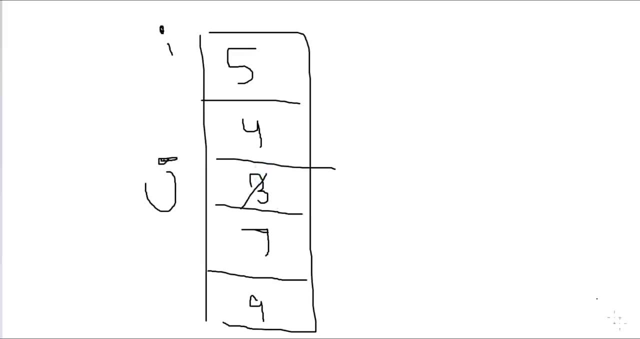 sorting algorithm which is going to cut, swap this. So you can see over here that it's going to be swapping. So we have three over here And then, initially, five is going to be over here. But what we want to see here is that in this text editor is that this is basically. 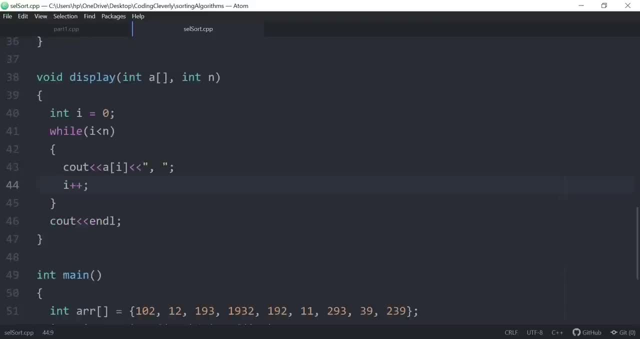 displaying. So we've had a selection sort And then, once we go back into our selection sort algorithm, we have a swap function. swap is going to get this value of i and a j that's returned from here and it's going to swap it. So basically, the simple swap app algorithm. 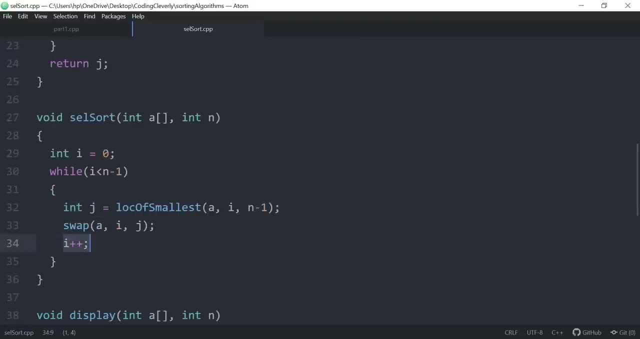 is going to swap the both values And then after that it's going to increment and it's going to go to our next location. So you could see in the place over here, it's going to now, not it's not going to be pointing. 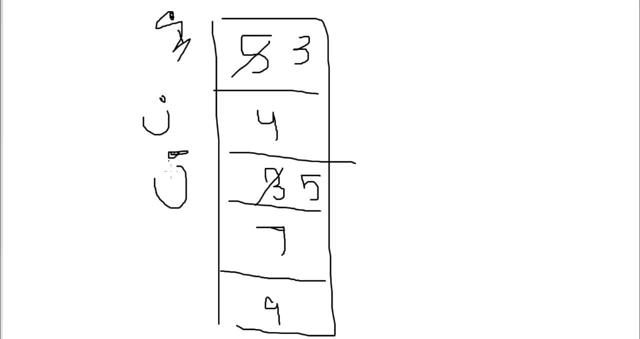 over here and anymore and it's going to be pointing over here, And now this J is not going to be over here. So just want to indicate that this J will now going to be pointing somewhere else. So we have this. I now incremented over here, So I is going to be incremented. 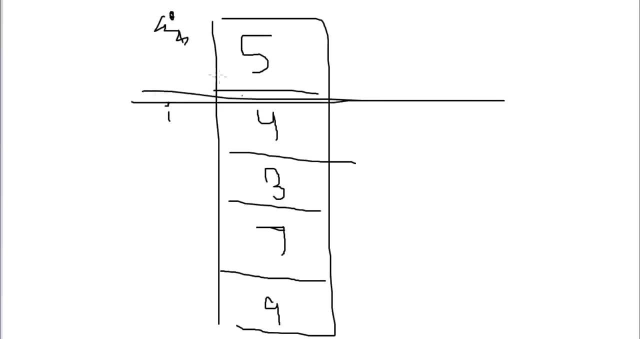 over here. Now this is going to be its base And what we're going to be checking now- because this is now going to be sorted with three. So now we're always basically over here, So now we're going to look for a value that is going to be smaller than four. So basically, 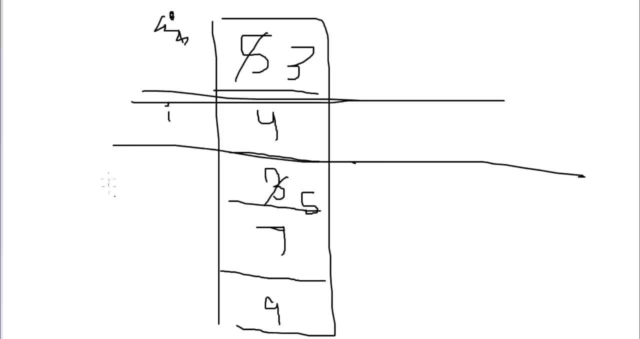 is there something for smaller than four? it's not so that we just increment And now we say I is going to be over here, Now it's five. if there's something, fine, it's okay. So it's going to be checking all and it's going to go throughout the loop until the 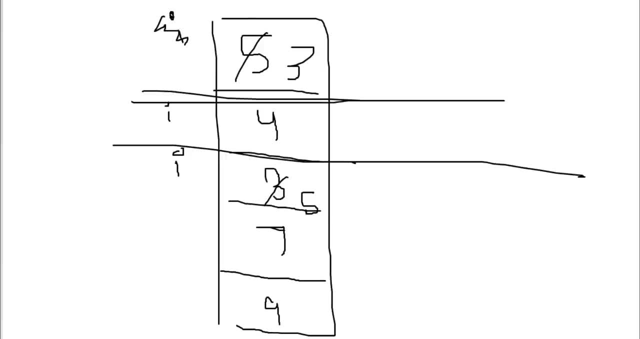 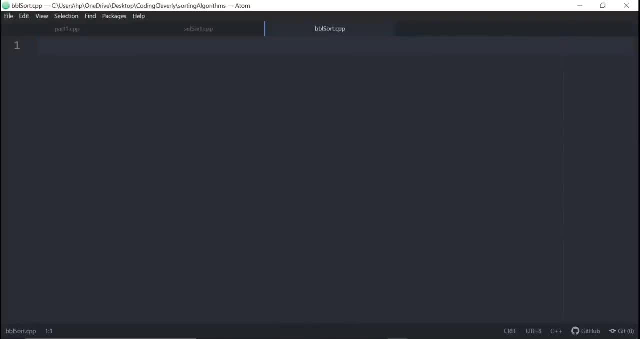 whole array sorted. So I hope you understood this concept of selection sorted through this graphical implementation. Now we're going to go to our next sorting algorithm And let's go towards it. Alright, so now let's look at another sorting algorithm. This is called. 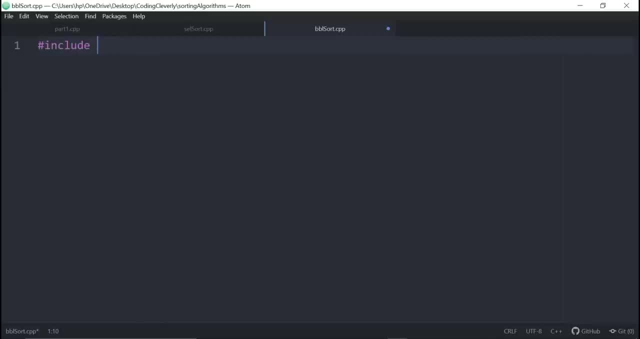 the bubble sort algorithm And it's going to go as followed. So, basically, you have to include your input output stream And you're going to have to do your namespace standard And let's just go simply write our boilerplate code. Okay, so, boy, this bubble sort is going. 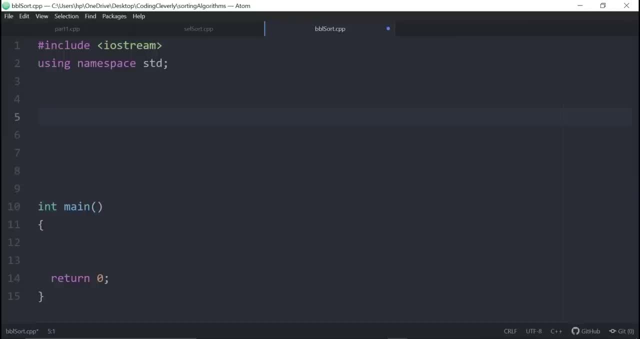 to also deal with swapping. So we're gonna have to include this swapping methodology, which is basically swap, And then we have an integer array, we have an x value, we have an y value And basically, when we go over here, we have actually a temporary which. 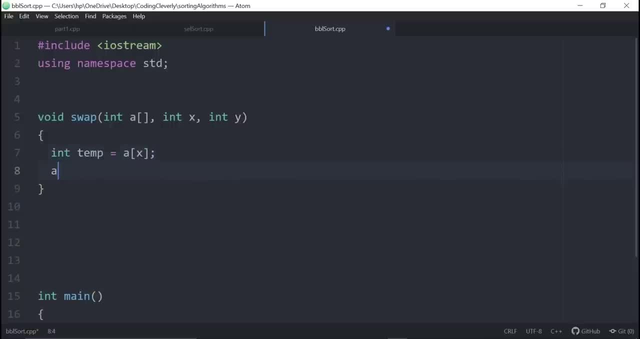 is going to be assigned to the first value. and then we have the first value, which is a sub x is going to be assigned to the a sub y value, and then the a sub y value will be equaling to the temp value. 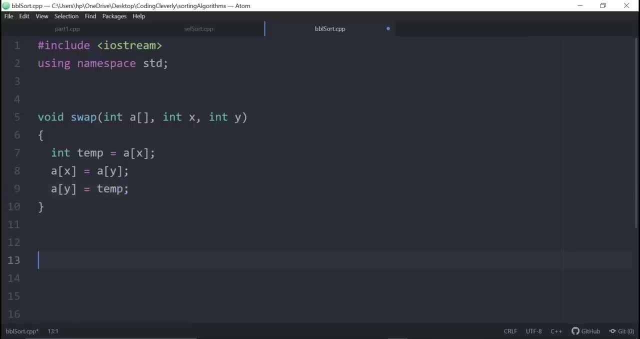 So this is how the swap works, And now let's have a bubble process. So the bubble process is a little bit different. How it's different is that, from selection sort that we already covered- we actually went from the top right, So we went from the top and then we went. 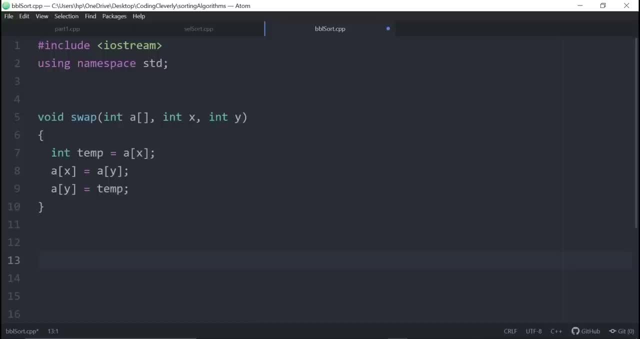 our way to the bottom. So in bubble sort we're gonna go Yeah, And then we're gonna 갦م bottom to the top. So I'll just explain it. So first just type along, So it's going to be bu. 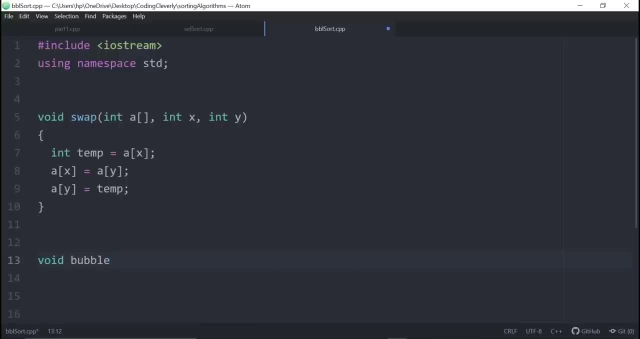 BB le bubble. And then what? what this process is going to do is it's going to do some specific process. it's going to get an array And it's also going to get the size of the array, And we're going to go back to this a little later. So let me just- I just wrote the signature right now And I'm 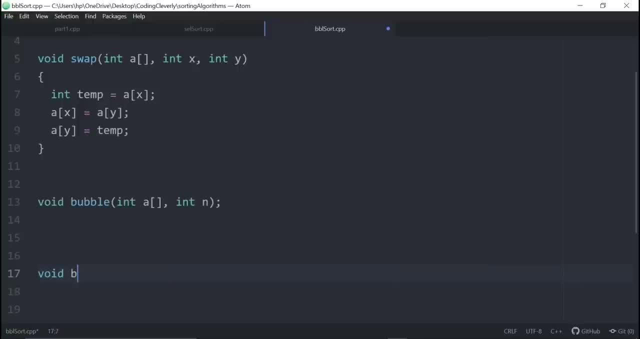 going to go and talk about the void bubble process, So the bubble sort actual functions. this is the actual bubble sort function And what we're going to do is basically, it's going to have that same integer array, which is right here, And then we have the size and n. So now, over here, what we 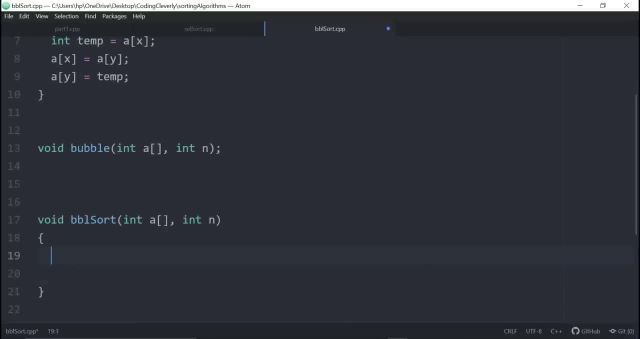 want to do is basically start from the portion what I was saying that the bubble sort is going to be adopting. So the bubble sort is going to say: integer i. integer i is equal to zero And what we need is, while we have, i is less than n minus one, the last element, we're going to have bubble process. So BB, BB, le bubble. 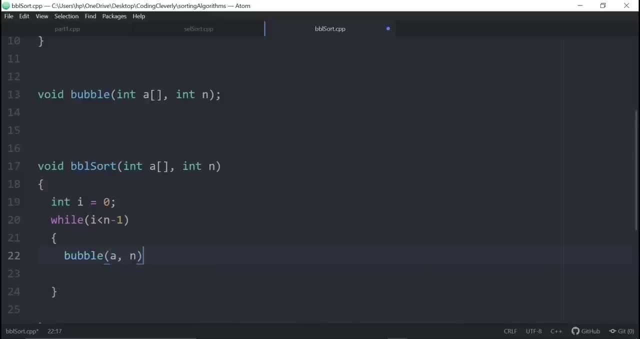 and it's going to have the array and the end value, which is n, is going to be the size, is going to be the array And it's going to increment it to the way. so it's just going to go and increment. So, in the bubble, what we're going to have is in here. now we're going to open it And 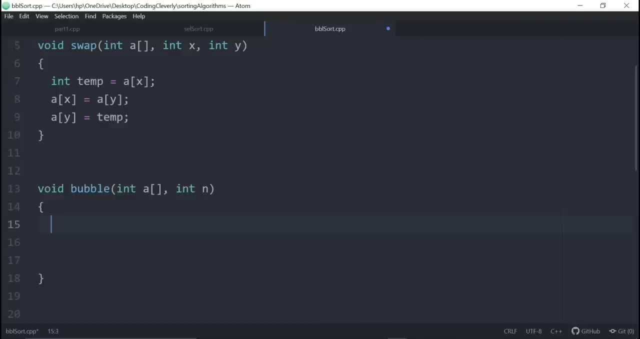 we want to start. so the bubble process is going to be from the I, so it's going to start from the last element. So that's what I was talking about, And minus one is the last element, And it's going to go like while and we have basically I greater than zero, so I 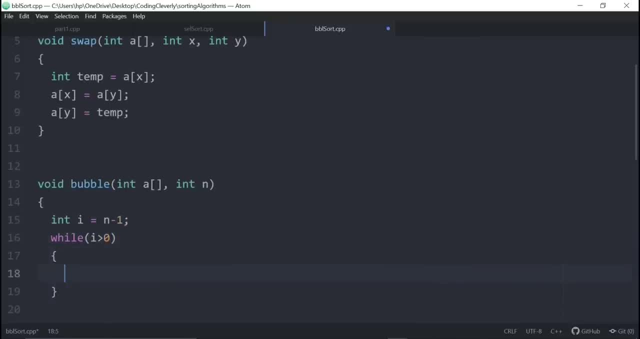 greater than zero. And now, inside of this is if we have a condition that if a sub i now a sub i should be less than a sub i minus one. Now this means that sub i, if it's the top portion, is greater. So what you want to do is that if a sub i is less than the 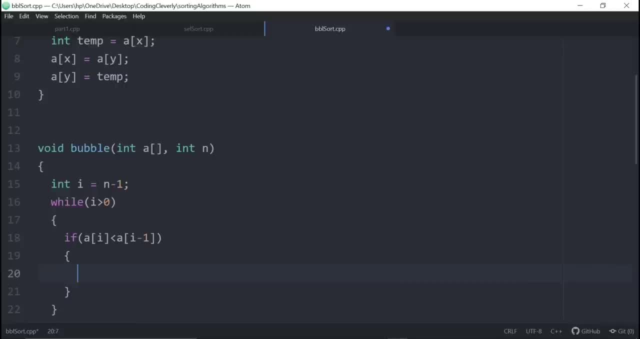 ace of i minus one. what you want to do is swap it. So we're going to swap it using this swap function that we already have. it's going to take a, it's going to take the i element and it's going to take i minus one. So that's how it's going to swap it And we're going to have a. generically. 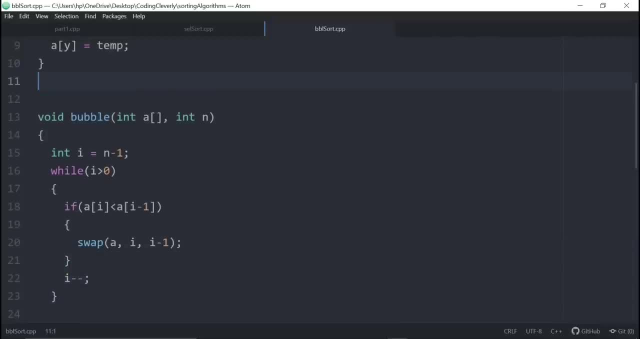 having going minus minus because we're starting from n minus one. it's going to go all the way to zero. So this process should work. So now, after that, we should have our display function And we're ready to go. So, basically, display over here, have an array And we also have the size of. 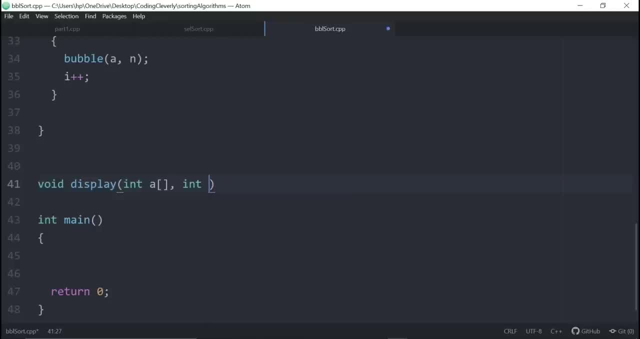 the array, which is some kind of size- I would just call it as that- And inside of it we need an input, So I would just say some kind of i is equal to zero integer. And then we have the loop process which is going to start from i less than n And then soon as go. 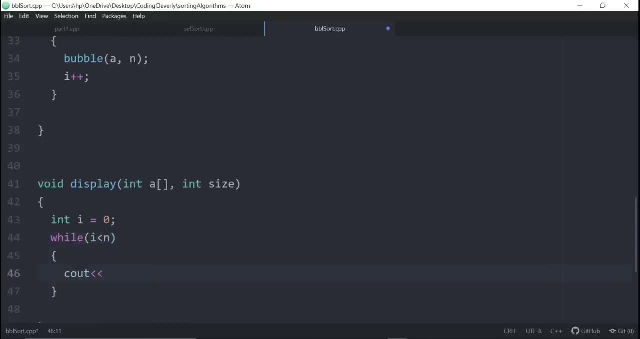 so basically, i is less than n and you want to process it, So array, and then we have the i's value And we're just going to keep on going like that until we reach our ending point. So we just console output over here, Yeah, and just to make it a little more similar to the previous one, 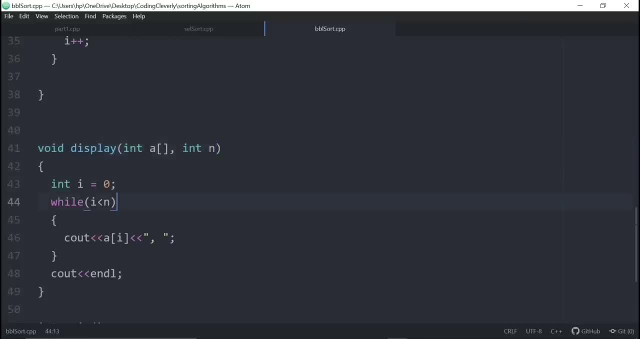 I'll just change this to just n, Because this one's matching here. So now let's create an array over here, And I'm just going to go ahead and create an array over here, And I'm just going to call it as integer array And I'm just going to give some random elements to it. So let's just say: 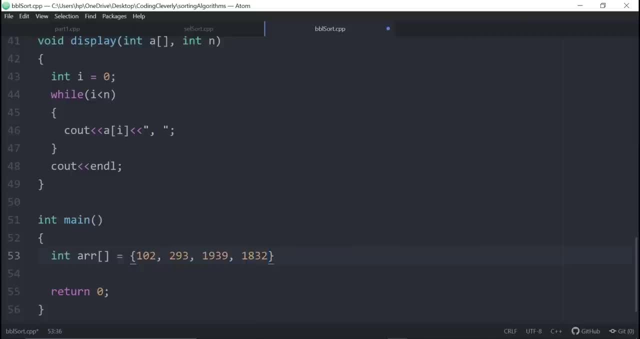 this and then this and then something like that: this, this and 33.. Okay, this is just random stuff. Now I want to sort this, So I'm just going to first display it. So I'm going to display, I'm going to say array and also need my size data type, So actually my size variable. So 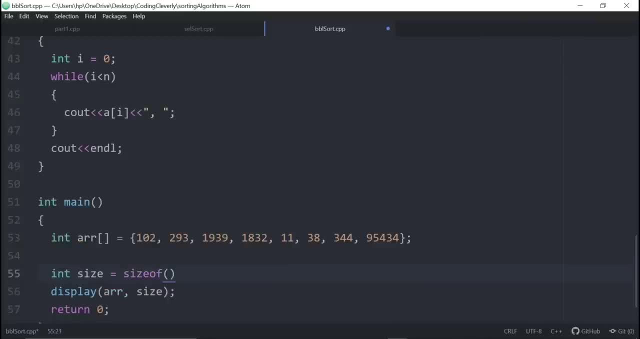 I'm going to have size And over here I'm going to say size of and I'm going to have the array and I'm going to say size of and I'm going to have the int. it's going to give me the 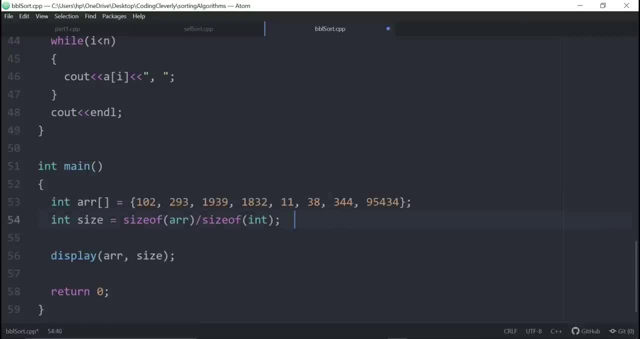 size. Now, what I could do here is basically have the display function called and then the sorted function. So it's called bubble sort. So I'm just going to name it bubble sort. I'm going to pass in my array, I'm going to pass in my size, I'm going to display once again. so I'm going to display. 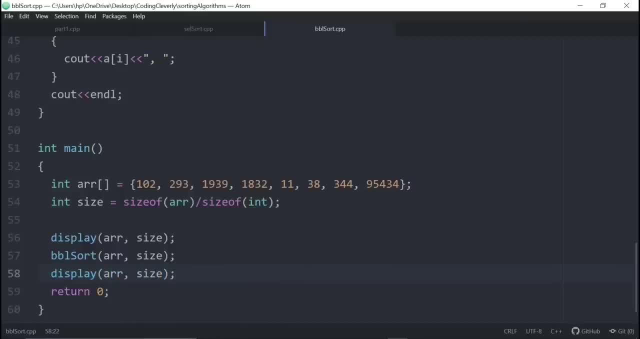 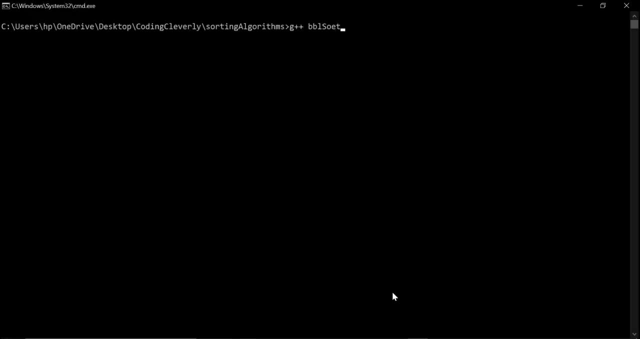 array and then I'm going to pass in the size. Now I supposed to work. So let's just go to our G plus plus compiler over here. let's just type bubble sort, bbl s o r t And we say dot, cpp, And let's just name it something like hyphen o, bbl s o r t. 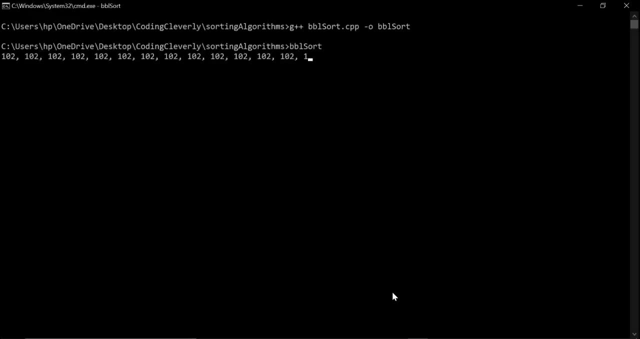 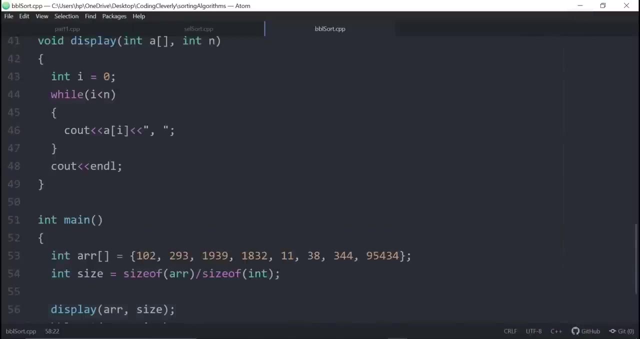 And there you go right, compiled, And there you go- Iran. whoa, what happened over here? I think we did the same exact mistake, So let's just go back over here and see where we went wrong. Okay, so we just forgot to increment on while loops, to remember to do this. this is really 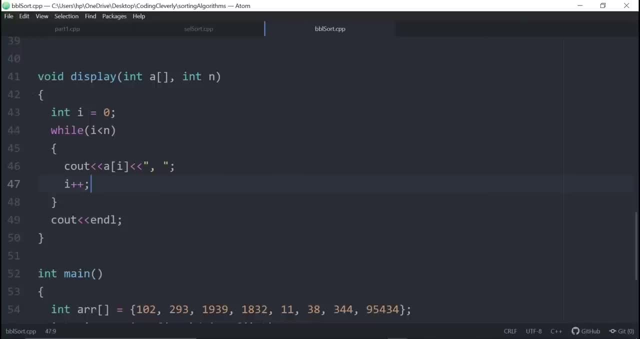 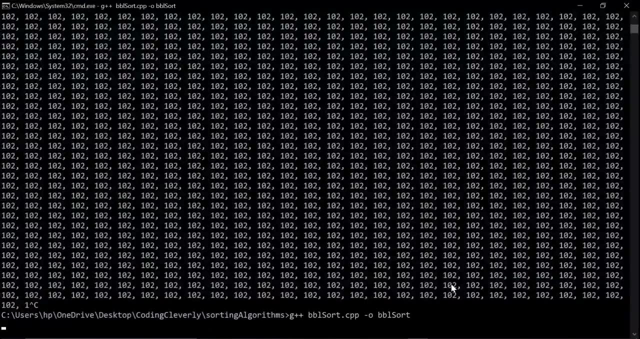 important. Okay, so I plus plus over here, so that is just loops out and doesn't cause an infinite loop. So over here and let's just go back over here to compile it, recompiling it and running it again. 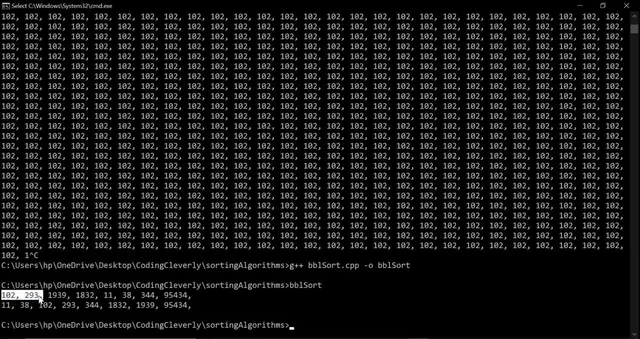 you can see that my original array was 102, and then 293, and then 1939, and all of that, And then, once we passed in our bubble sort, it actually sorted out some from 1138, 102, and all the way to the last element. So that was pretty cool. assorting an array in ascending order. 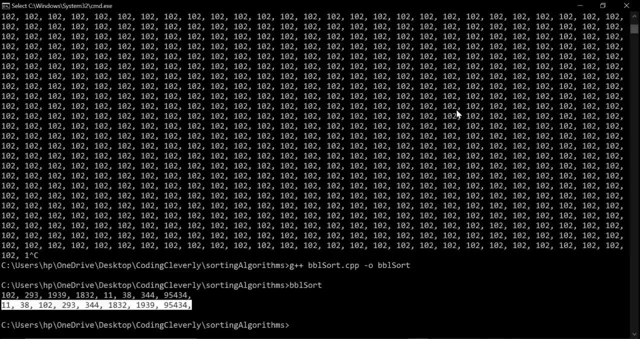 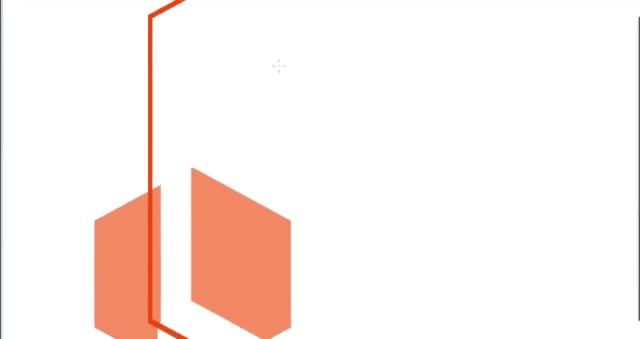 using bubble sort, collection sort- because the the methodology was basically a little bit different. I just want to show you how this is implemented in a graphical way. So so the implementation of the bubble process is basically similar to what we did with selection sort, but in actually reverse. 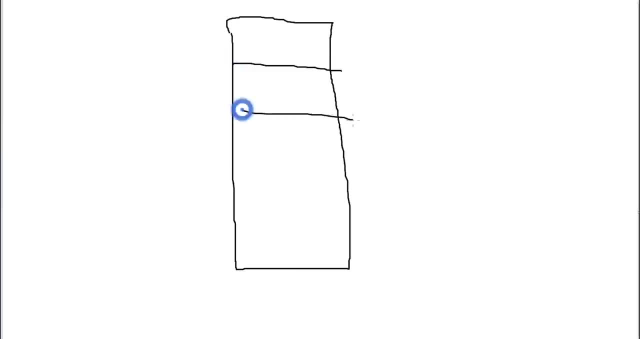 order. we have a swap function that's going on, But we have this visualization that could help us understand how this process is working. So suppose we have some random values here. we have three, we have five, we have one, we have four and we have, let's say, three. 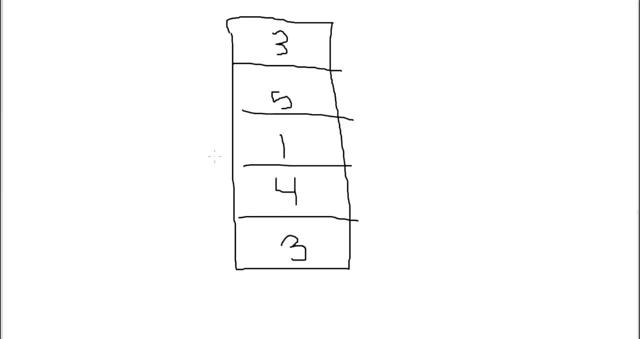 Now the bubble process is going to work like this. So let me just go over here And now let's see. So it's going to start from the bottom and it's going to compare these two values. Now it sees that three and four. now what you mean? that is basically bubbling, meaning it's liquid portion. 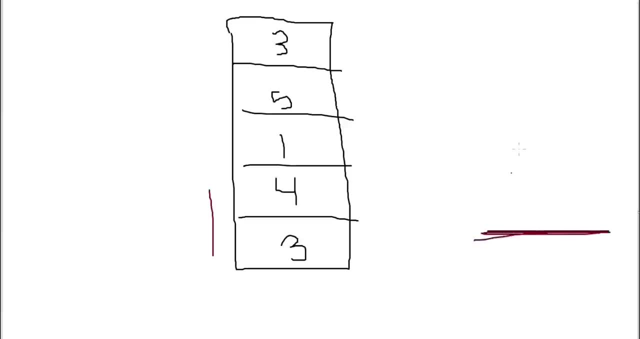 is on the bottom and liquid portion is basically heavier than the bubble. bubble is lighter. bubble makes it flow on the top. So when you compare a liquid and a bubble, bubble is lighter So bubbles should be on the top. So this is exactly the same thing. They're talking about the weights. So four: 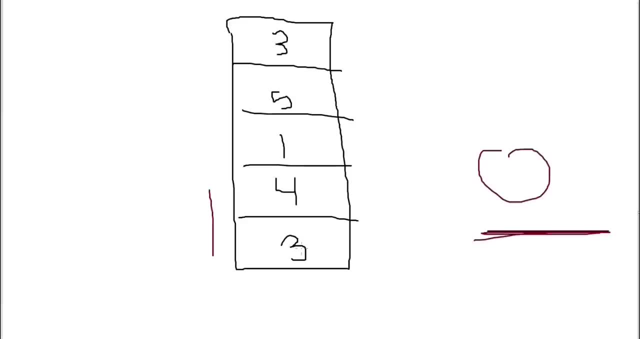 weight is heavier than three weight, So four should be on the bottom and three should be on the top. So this is the actual process. What's happening here is that the swap function will be called and this is going to be changed to three, and this is going to be changed to four, And then, after that bubble. 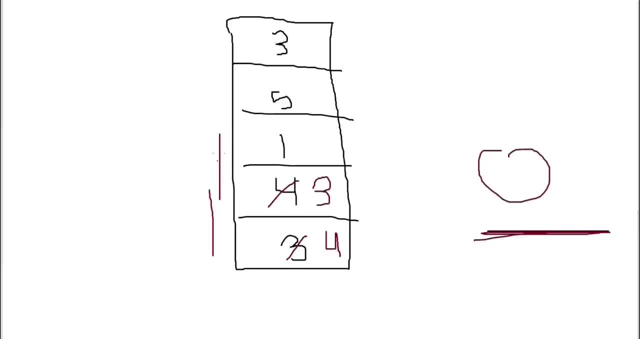 will go up over here one step level. So it's going to go from here Now. it's going to go over here. So now it's going to compare three and one, So three and one. actually. what's different now So you have over here, is basically you say one and three, So actually it's okay. So three is heavier. 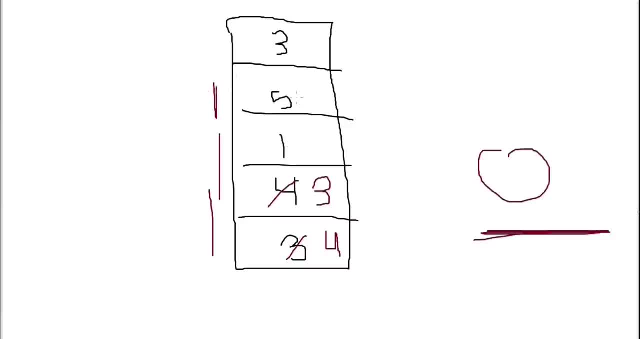 than one. So one, it's okay. So go again over here. one and five, So five is heavier. So basically five will go on the bottom and one will go on the top Now now over here. now. one and three, So basically three is heavier. So three will go on the bottom right here. So just three. 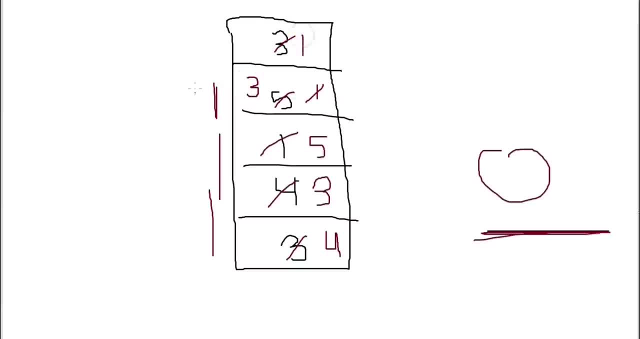 is on the bottom right here And then one is will be on the top. So this is one actual bubble process And you can see one, three, five, three and four Right now. we basically did our one process here and we sorted till this portion. There is more processes and you'll need to do. 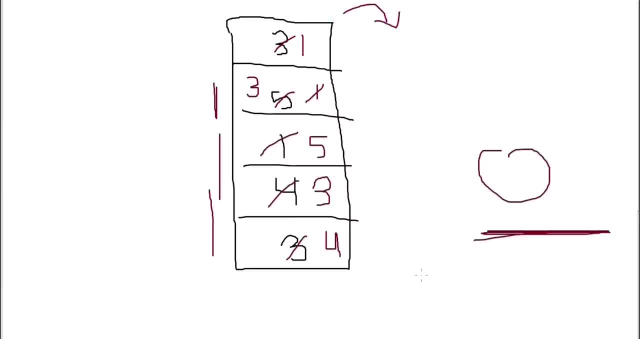 one more bubble process. So again you're going to have to go from the bottom, So you're going to check like this. So basically we're going to start again And we're going to see the values once more. So forgive my writing, So four and then we have three, and we have five. 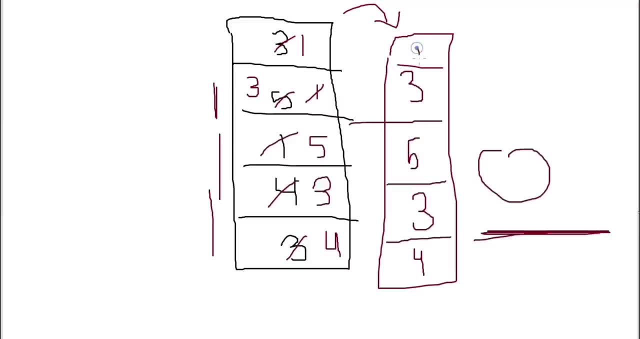 then we have three again over here and we have one, So now four and three, which is heavier. it's okay, go up here, compare these two values. Now three and five, So three and five. actually five is heavier, So five will go on the bottom, So five is over here. 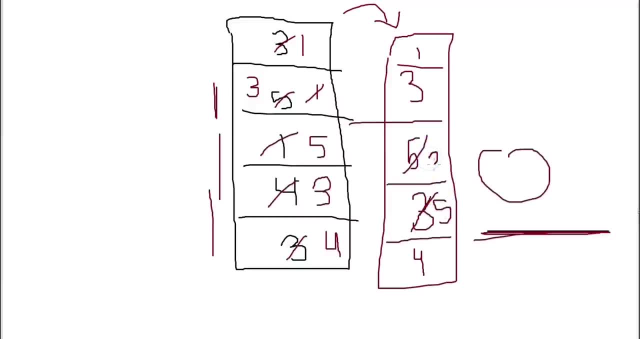 just cross this one out And this portion will be having three now, Now three and three. Well, actually it's the same, equal, So it's going to be okay, So one and okay, so it's okay, So one. 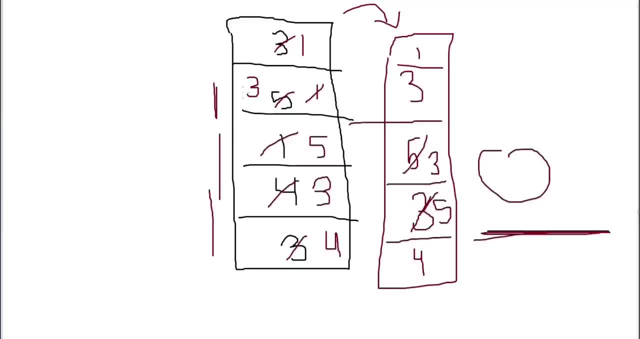 three, three, five, four. Now one more process. So after one more process. so we're going to have one more process. So let me just erase all of this. we're going to have an even one more process, And now this should be our final bubble process. So let's just look at the values again over here. 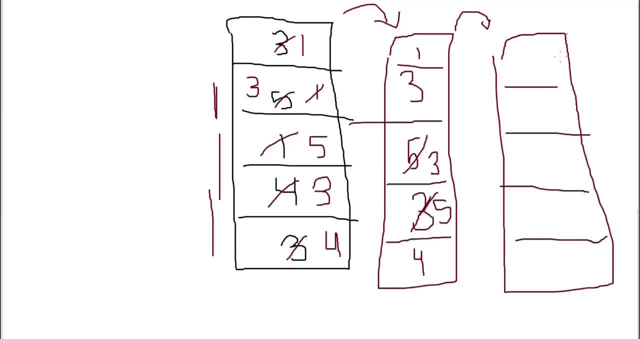 and then over here, and then over here, and then over here. So this is one, and then this is three, and now this is three as well, And now this is five, and this is four. So it's going to start. 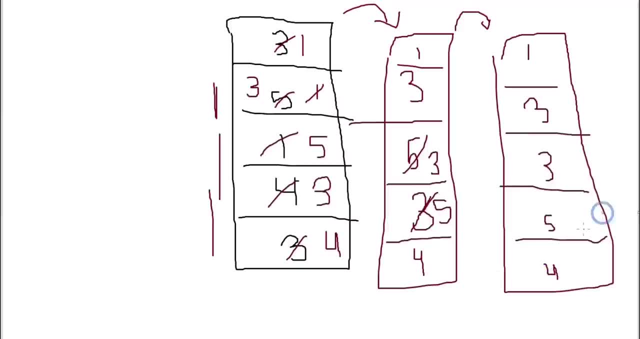 from the bottom And you see that five and four. well, five and four. this is different, this is heavier. So the heavier portion should be on the bottom and the lighter portion should be on the top. So four is going to be over here And then five should be over here. So five, four and then. 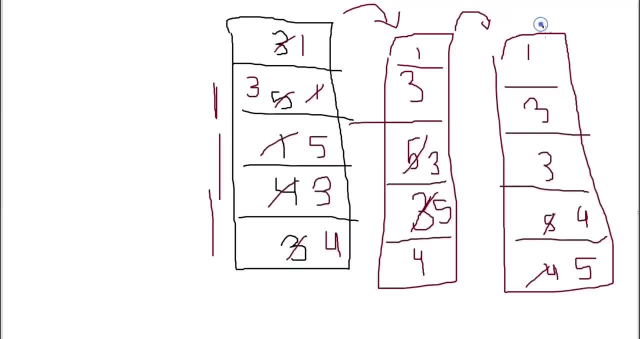 three, three, one one. it's okay. So this is our exact sorted array And this is how we're going to be sorting our array. in bubble sort a slower and it depends on the number of inputs, So it could vary and exponentially grow as the inputs increase. So that was bubble process. 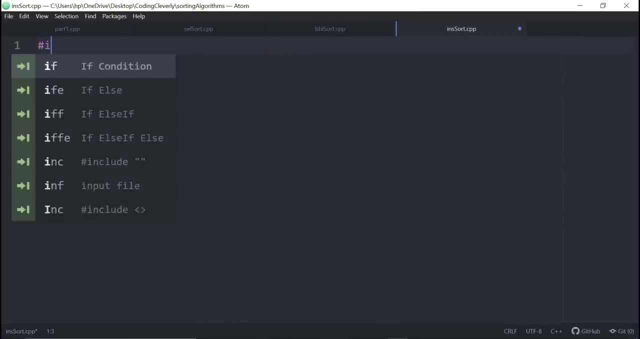 Alright, so now let's jump into insertion sort. So this is pretty much different from the other two that we've included right now, which one was selection sort of. no other was bubble sort. So I would just encourage to type along with me, and the explanation will be doing side by side. 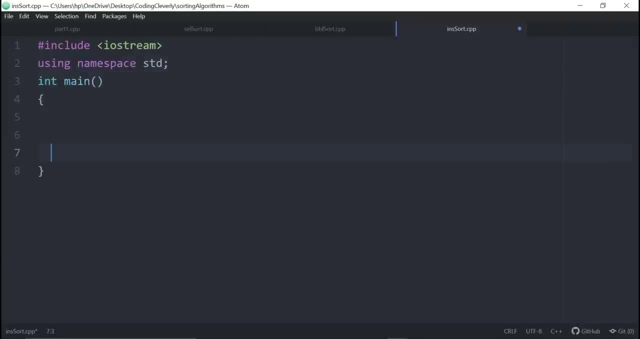 So let's just go and include this main and then let's just go over here and then return the zero, Okay, okay, now what's gonna happen here is that we're not going to have a swap function like we did with the other ones. what we're gonna have is basically some differences And now the 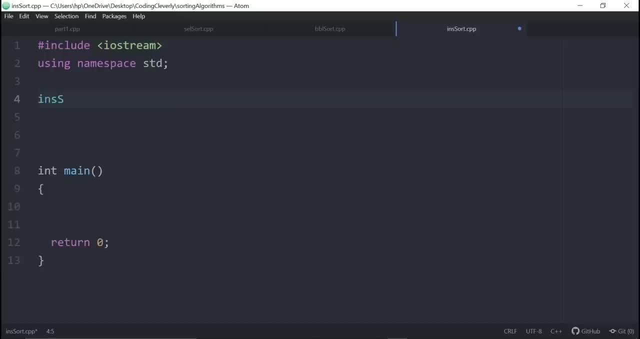 differences is that we're going to have an insertion sort function And the insertion sort is going to basically have an array. it's going to have one more thing that is going to be inside of it, So the first thing that's going to have is going to be the size. This is pretty much the. 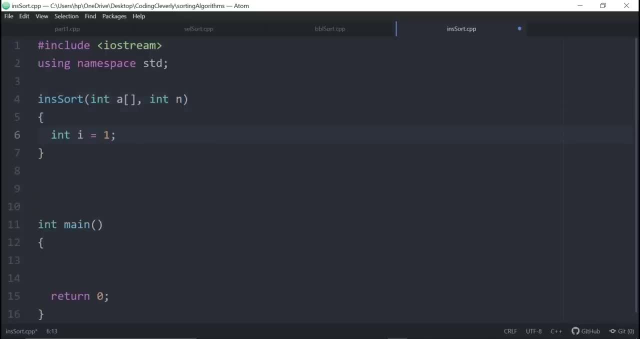 similar, And one thing here is that it's going to start from one, not from zero, like others that do, because we're assuming something, and assuming is that the assumption is basically that some portion of the rate is already sorted, And then the other thing is that the assumption is basically 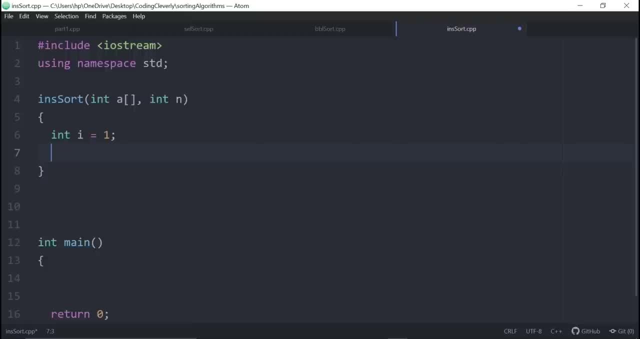 already sorted beforehand And we just have to, like, insert elements, be into that sorted array, And that's how our process is going to be done. So we're going to go and we're going to have a while loop so that I could tell you that it's going to go in a while loop. it's going to go to n. 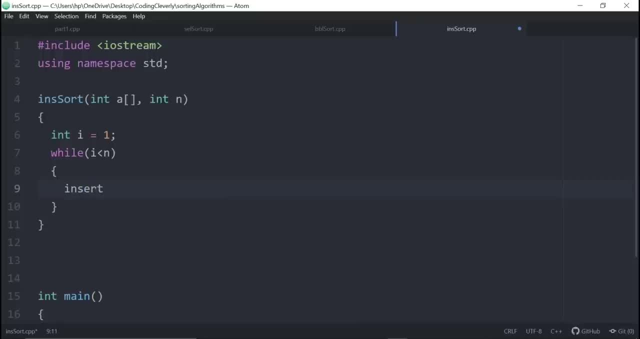 and it's going to say: insert, insert it. this is going to be the function that's going to be called, and this function is going to take in an array. it's going to take in the size, is going to take in the element, which is going to be the portion that I'm going to be talking about. And then this: 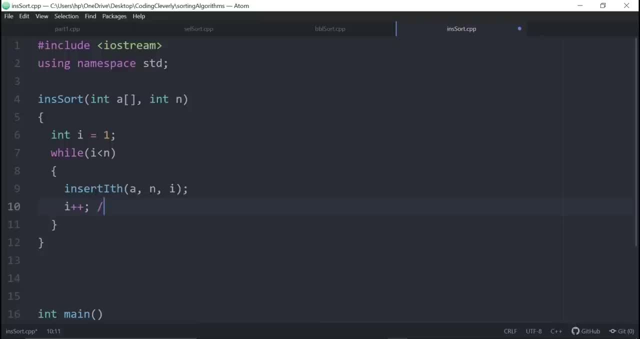 is going to keep on incrementing: I plus plus right, Like in other languages. like I is equal to i plus one, whatever it is. man, I can't get the plus right, Okay, so just like that. So I plus plus whatever. it is like that. So now let's have the insert ith element. how do we do? 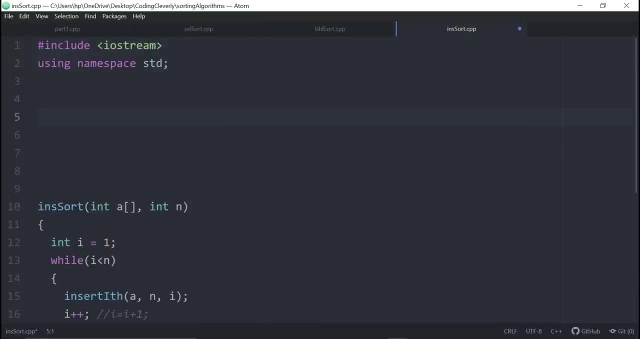 this insert, I think. so let's go over here And after this let's just talk about the insert ith. So this is actually something that's also void And it's going to have the insert ith element. So just ith over here And now inside of it, we're going to have the array, we're going to have 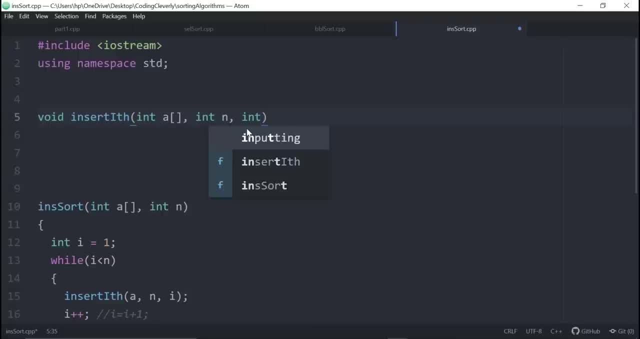 basically, we're going to have the integer n size, we're going to have the integer i size, which is specified over here. we're going to have this key variable, a mid intermediary variable that's going to store our ith location, or basically the value of our eye. And now it's 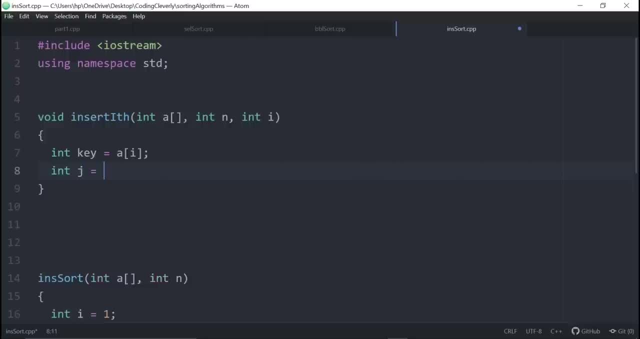 going to say int j And this is, j is going to be the last element of that sorted array. So last element of that sorted way was going to be i minus one, because I is actually after the sorted rate, and I minus one will be the one last element. So we're gonna have a loop again and we're gonna 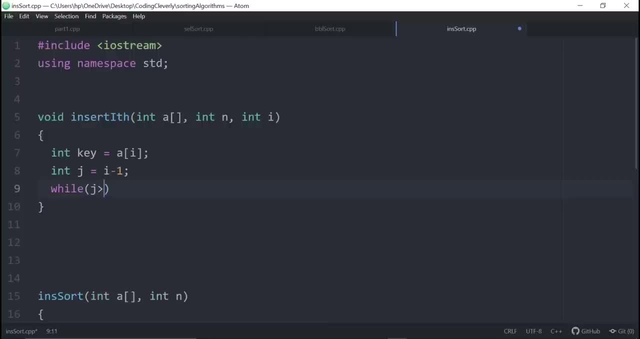 have two conditions For this case. we have j is greater than equal to, we have j is greater than equal to zero. And we also have one more condition: that j should be actually greater than the key. So if j is greater than the key, we're just going to keep on looping this. So not a, g, j or whatever. 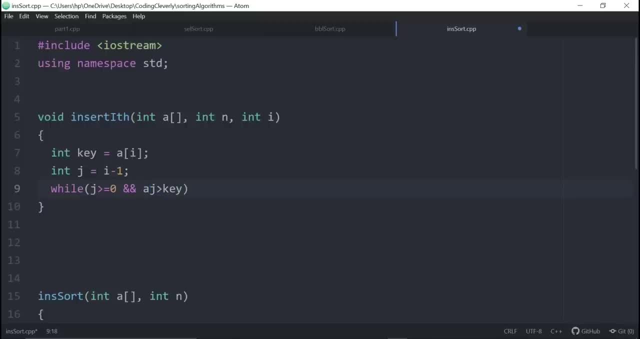 it is a key. So a sub j. So let me just have this a and then a j over here, not just plain j. Okay, so a sub j should be greater and then the j should be greater than equal. So what's going to happen here is that a sub j plus one. this is going to be. 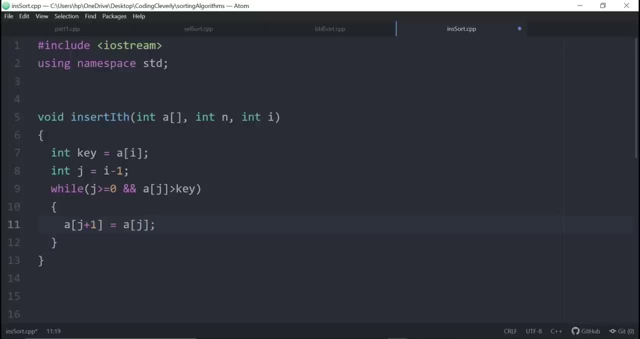 implementing and it's going to equal to j. and I hold on, I'm just going to teach you this, Don't worry. So now we're gonna have j is equal to j minus one. Now it's just going to keep on decrementing, going to the top like a bubble sort. it's going to go up and up and up until you reach. 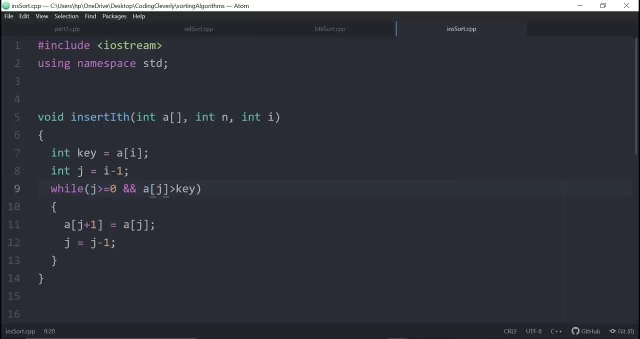 that less than equal to zero, or if a sub j is great, basically greater, or if it's less than, something like: if it's less than, then it's going to just break out the key And naturally, what's going to happen here is, if this condition is false, we're going to 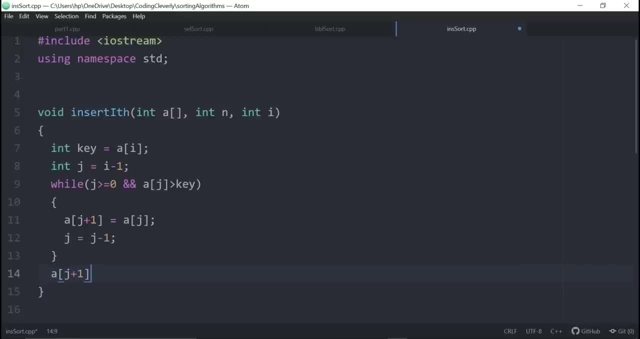 have a sub j plus one, whether we're trying to implement and we're going to put that key thing inside of it, that lost value. And now we just have this display function which is going to be over here. let's just have it over here, So void, let's have a display And let's have an integer array. 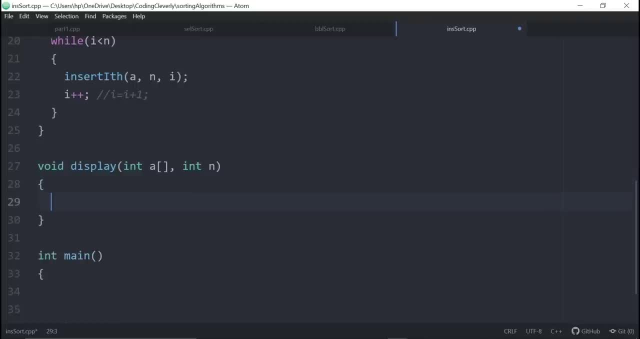 And then let's have the size of it And then let's have something which is going to be the I. it's going to start from zero, it's going to go basically from while and it's going to just check that I is less than n And 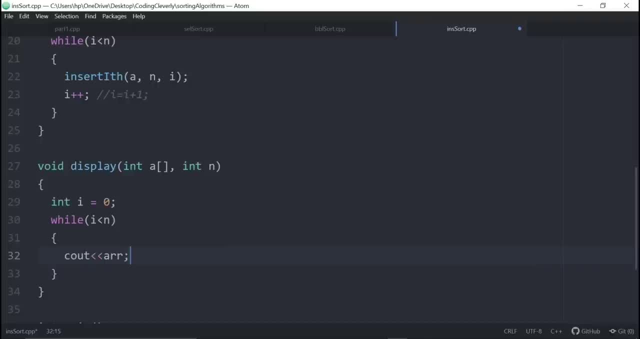 then it's going to go and say our console output is going to say ARR. Actually it's not ARR, it's going to be a sub i and it's going to be I, and then it's going to be that over here. 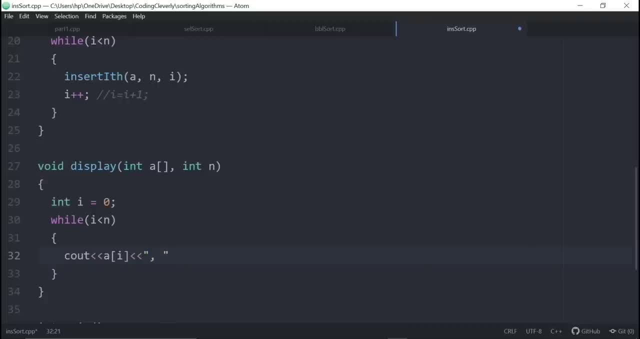 there's going to be a comma right there And then there's going to be an endline semicolon right here, And actually not this. I don't want that, I just want a semicolon. And this is going to be incrementing, so i plus, plus, and then we're going to have a comp N line over here. There you. 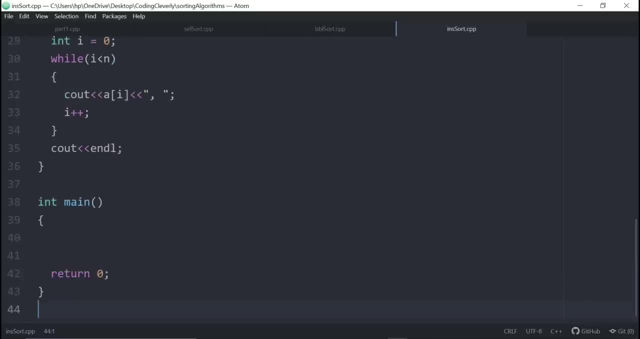 go And let's just get some data from our previous sorting algorithm. So like a bubble sort, let's just get some of the data, just the array portion, not anything else. So just get this portion over here. Let's just copy this and just come here and just paste it. So I'm just going to go here And 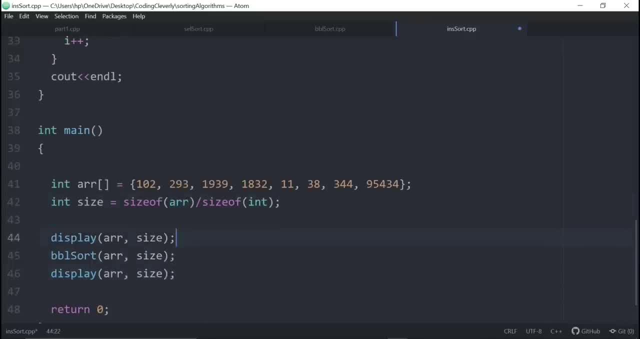 we're just going to paste it right here. So the only thing I'm going to be changing here: everything is okay. I just want to sort it using my function. So I'm just going to call it with my insertion actually. yeah, so insertion sort is going to be called. Okay, so the insertion sort should be over. 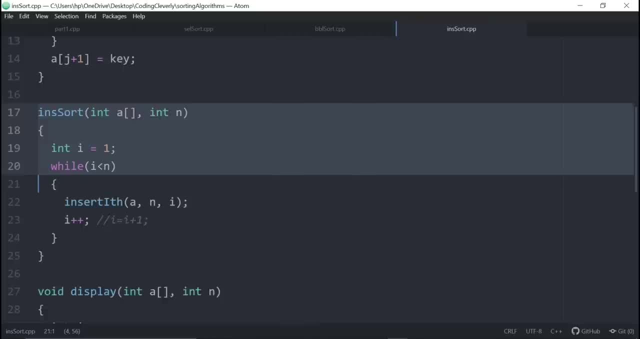 here. Let's see, Yeah, the insertion sort is right here. it's going to go and it's going to call this one insert it. it's going to, it's going to perform some operation and then it's going to go back. 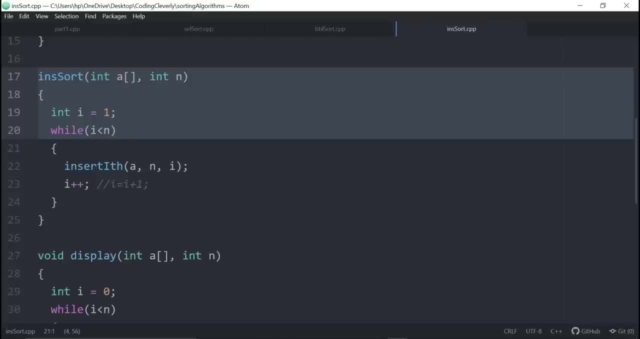 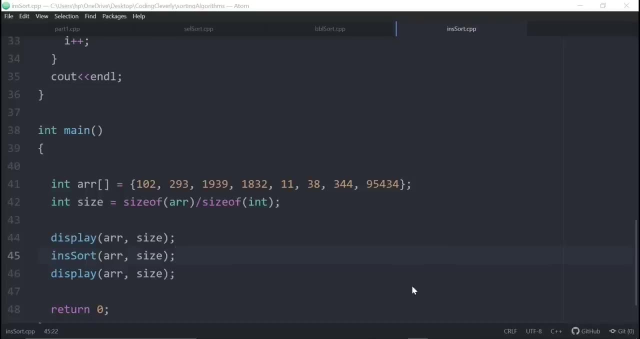 plus plus. it's going to keep on doing and it's going to keep on calling this, insert it so many times until the thing is sorted, And then after that we just display it. So let's just run this code- I'm going to go over here my G plus plus and let's just clear this screen And let's just 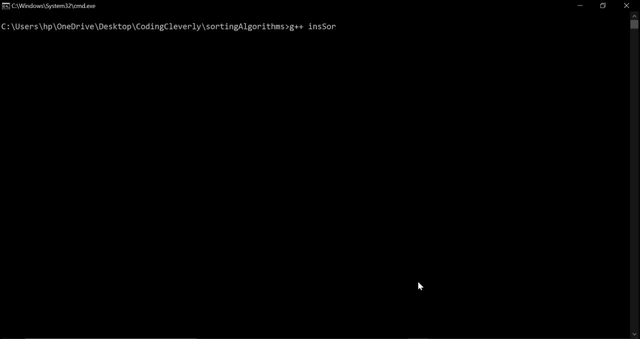 compile. So basically G plus plus ins sort, insertion, sortcpp, And then we can say hyphen O flag and then say ins sort. Okay, it should be working. compiling Okay. so there's a warning over here and 25.. No return statement in your function. returning non void 25.. Let's see. 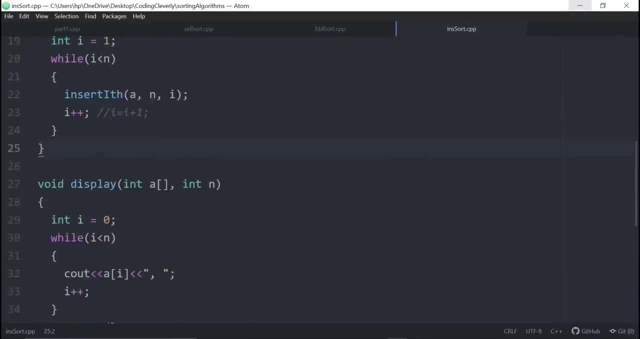 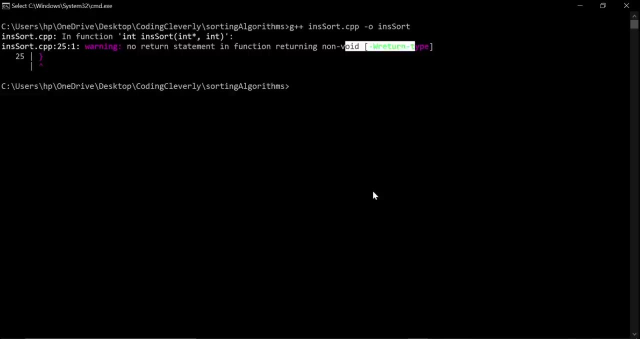 25.. Where are you? 25 is over here And there is should be something over here- insertion sort, And it doesn't have a return type. Wow, should we have a void? So let's just have a void over here And let's just go back here And now let's just compile a recompile it. 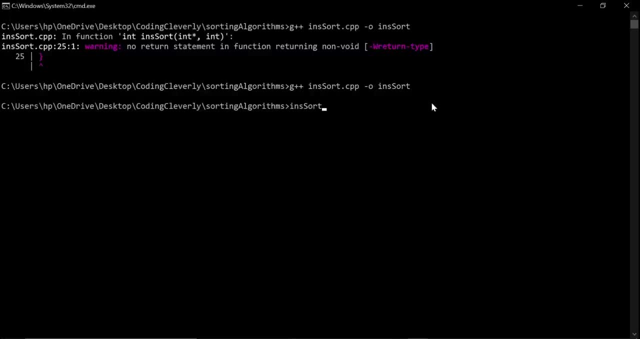 And there you go. Now we have ins sort, So insertion sort, And if I run this you're going to have this sorted. So 192, 293, 1939, 1832, yo, yo yo, 1138, 102, 293, 311.. And this: 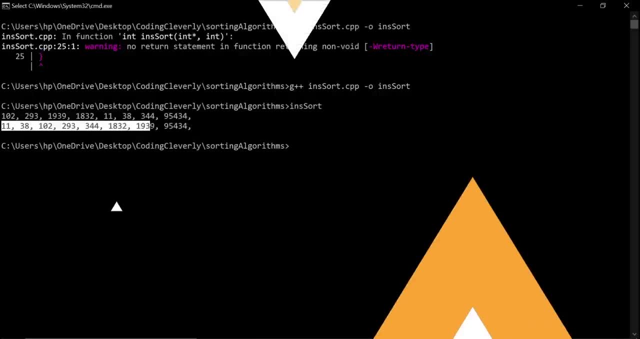 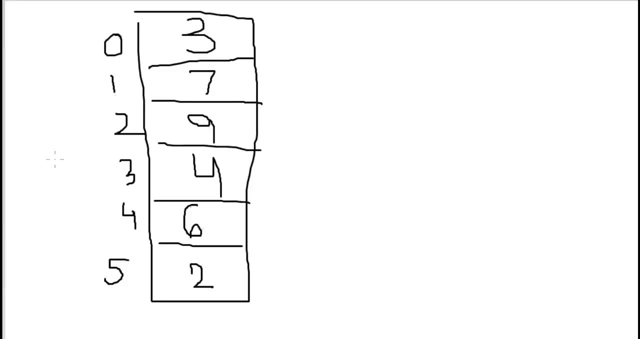 is also sorted in ascending order. Now let's have the implementation. So this is the basically an array, just random sample, And we have 379.. And somehow this is basically sorted from here How that happened: just randomly, it just sorted beforehand And now our eye is going. 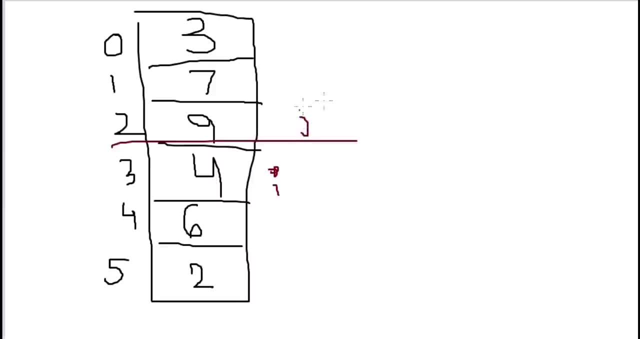 to be over here. So it's going to be after that sorted And then J is going to actually be going to be over here. But remember I said that it's going to be I minus one. So this is J And the. 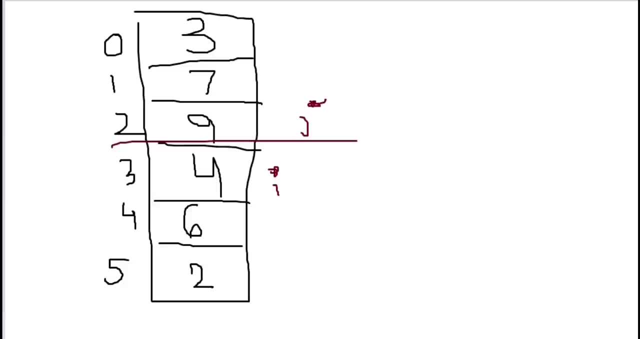 first process is going to happen. So if I go over here and back in my code, so my code is over here- And if I see over here that this is going to be the process insert, it has an array, it has the inside. 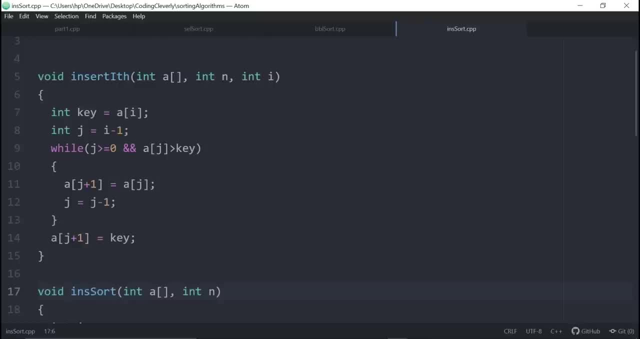 It has the element i And it says that key is equal to a sub i. So there's going to be a variable that's going to be stored and j is equal to minus one, And it's going to say that j is going to equal. 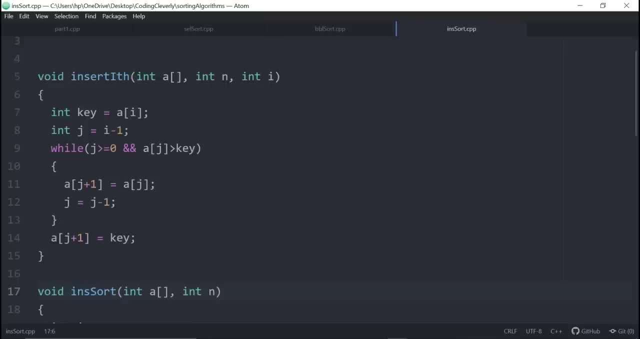 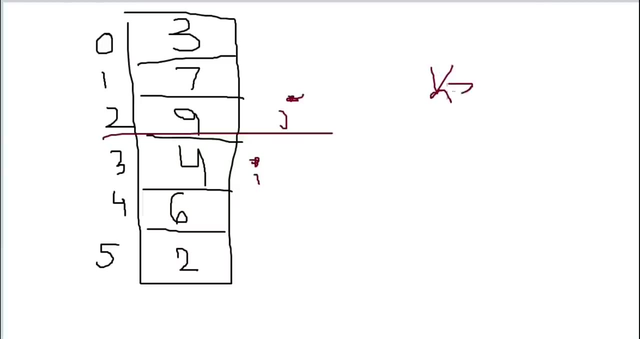 to zero and a sub j is greater than the key. So it should be working like that And let's see if I could implement here here. So we have a key variable, So there's a, have a key over here, So key k, e, y store that value inside of it, which is going to be something inside. So what's it going? 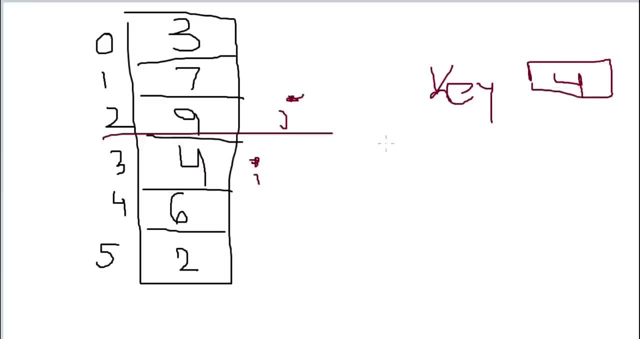 to be. it's going to be the value of i, it's going to be a sub i. So that's four. So four is here. Now ignore that. Now, what you're going to do is basically, you're going to check the condition. 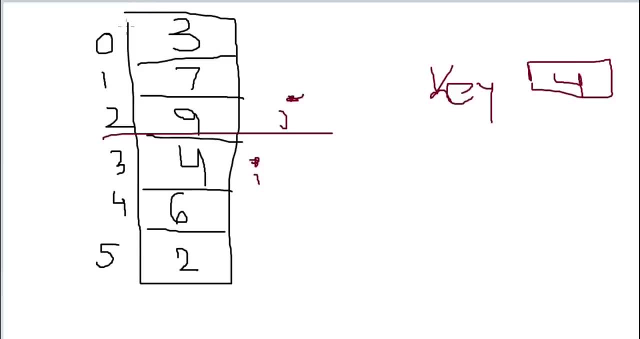 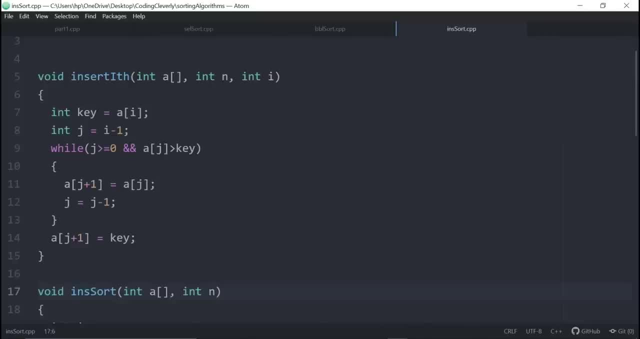 and the condition is true. Why? Because a sub j is not. it's not, it's a greater than equal to zero, actually. That's why, if I go back over here, where am I? Okay, so you could see that it's. 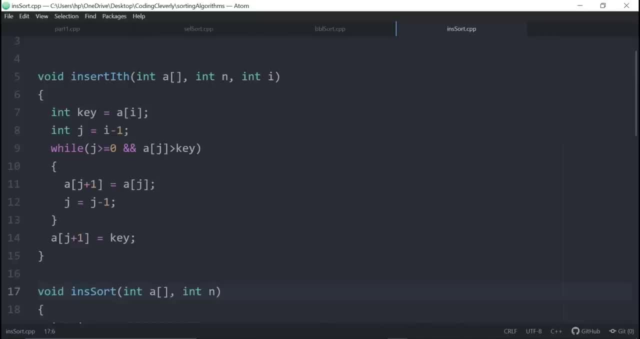 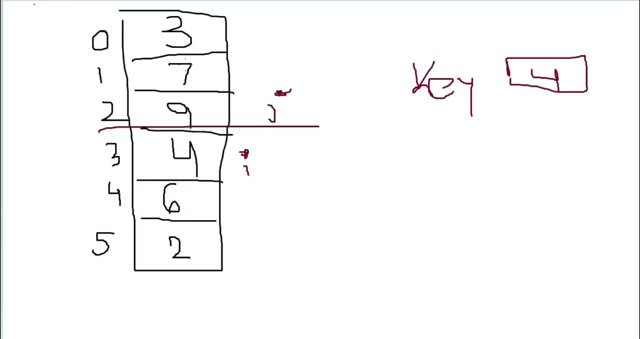 j is greater than equal to zero, it's perfect. And then a sub j is greater than key. Now, if I talk about the a sub j, Now if I talk about that, let me just see: A sub j is basically this nine right now, And we have a key which is four. So 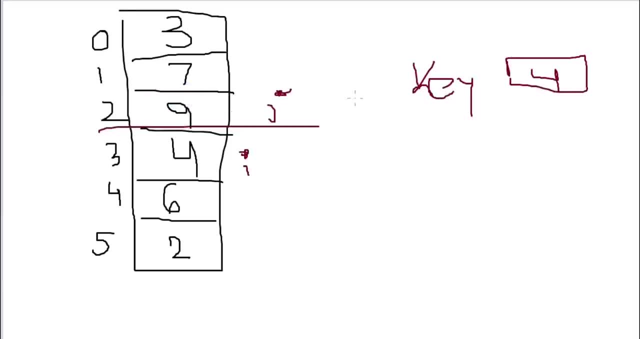 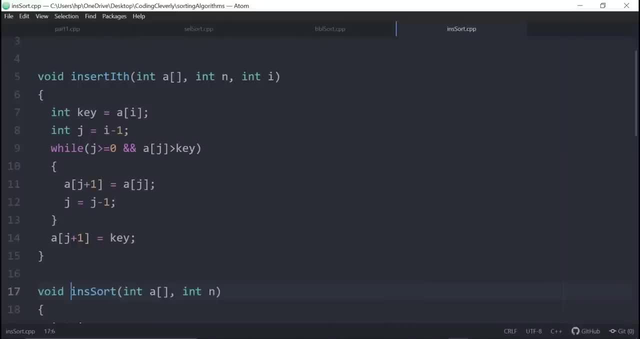 that a sub j is greater. So, no, no, fans, we're, we're still working. Okay, so the work, the thing is going to still work. If I go back over here, we're going to have a sub j plus one is equal to. 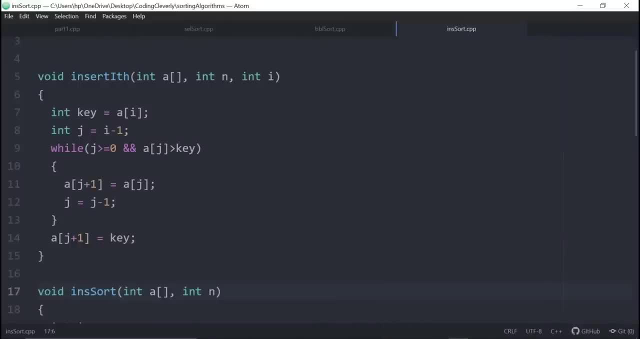 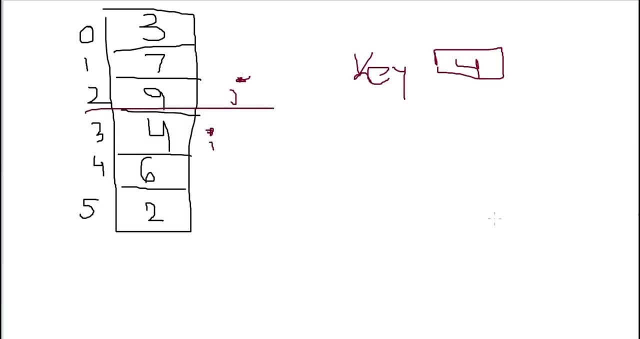 a sub j, So that means that we're going to have something that we're going to be implementing. So a sub j is going to be over here, So we're going to go over here. So this is going to mean that j plus one is this portion is going to equal it. it's going to sign this nine over here. 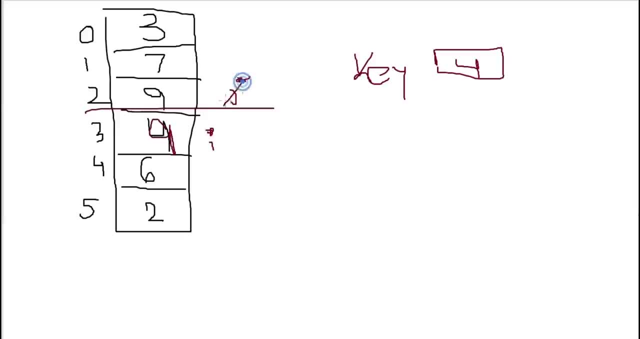 And what's going to happen is that is going to go minus one, So j is not going to be here anymore, And now it's going to go over here, Okay, so that was now. that's one process of that loop. So that's one process of it, And 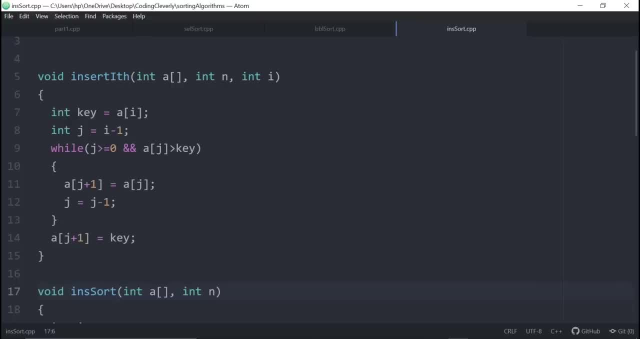 let's go again. So a sub j greater than this is greater, j is greater than equal to zero, and a sub j is greater than the key, because the key is four and j is seven. So that's perfect. Now let's go back over here And we see that a sub j plus one is equal to a sub j, And we have 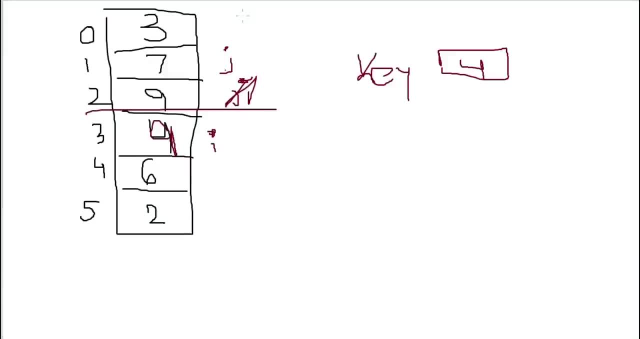 j minus one process again. So whatever that value was, so we have seven over here. that seven is going to be now over here. Okay, So the j is going to go up here now And it's going to move it. You can see that the I still 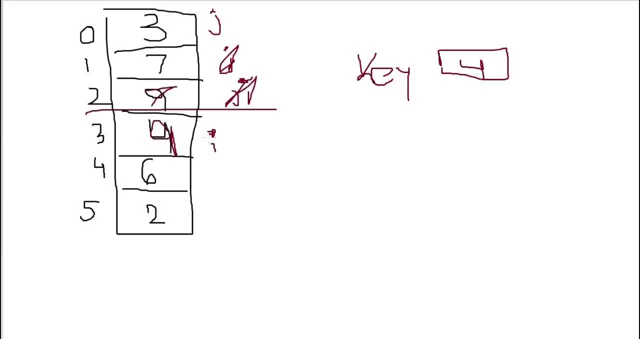 over here, in this location, and you can see that the four was removed, So we don't have that value anymore, that it just changed to nine. see over here, this is nine. And where does nine come from? it came from here, So, with a seven came from. it came from here. So this is happening, So we have. 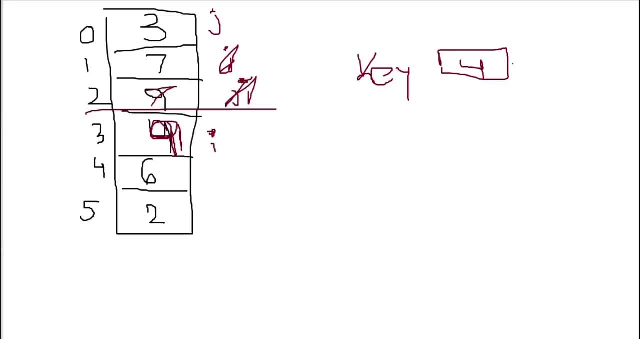 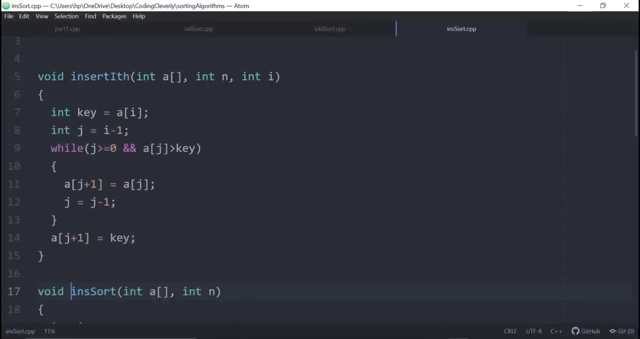 this lost value over here, stored in our key. So that was the purpose of the key. Wow, nice key. So now we're going to do is basically go over here And we're going to see a sub j plus one, and it's gonna, it's gonna see. 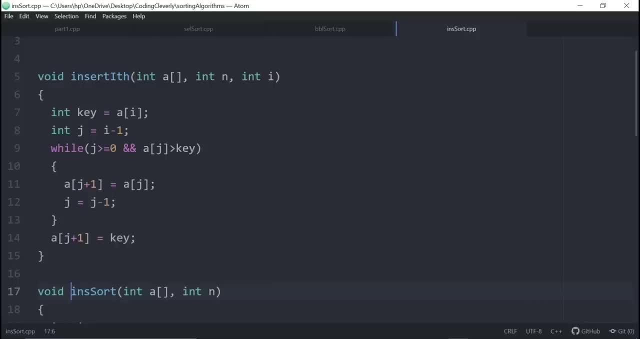 this condition: is j greater than equal to zero? Well, that's true. If I look at that position over here, it's over here. it's greater than equal to zero, but it is equal to zero. So it's true. But the second condition is not true: Why a sub j is greater than key? And actually it's not. 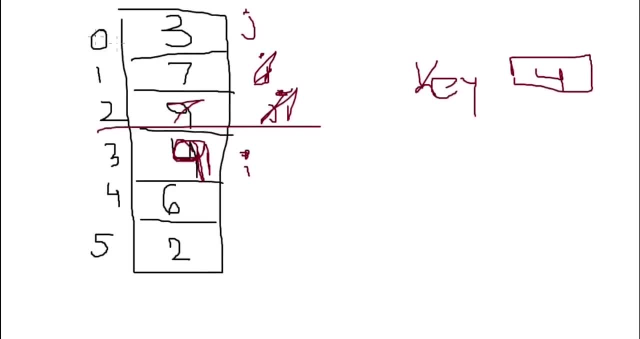 greater. How is it not greater? It's less than because it's three down. this key is greater. So this just terminates that loop, And what's going to happen now is that the key is going to be sorted inside of this, this portion over here, which is j plus one, So that key value, which is 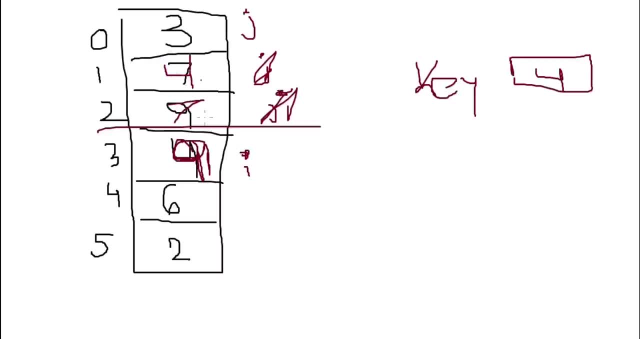 four is going to be over here. Now, this four is going to be over here. 3479.. Well, this is sorted, And now it's gonna it's gonna move on, And this is I, now new position of I, and this is going to. 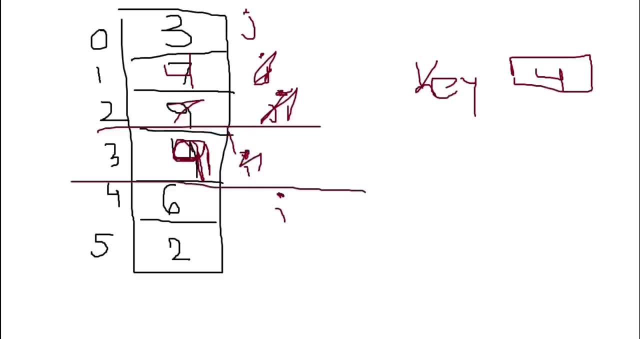 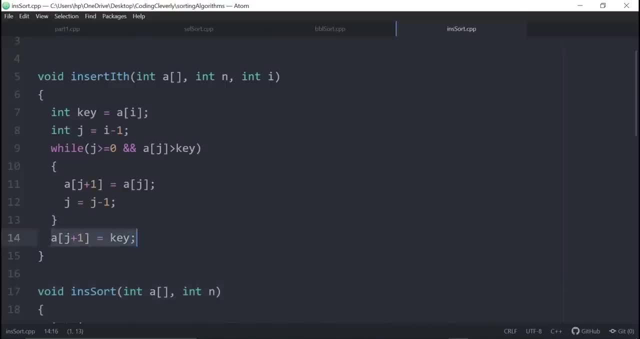 be a new process, So that's how it's going to be starting. If I look back over here, So you can see a sub j plus one is the key, and then the process starts again if you want to do it. And that's how. 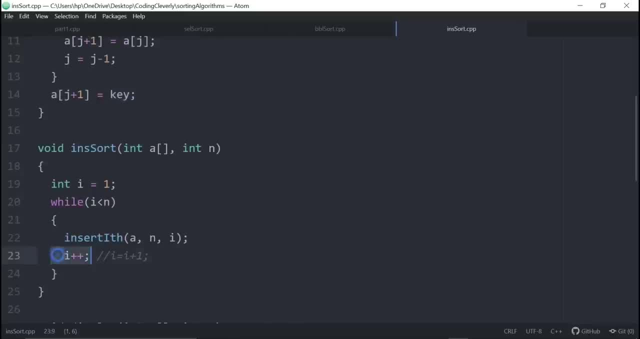 basically, we're going to sort it, insert, sort it's going to increment its eye value again, it's going to go in new playstation, And then after that position, and then after that we have insert. i then the process starts again and again, and again, until the whole damn array is sorted. And then we 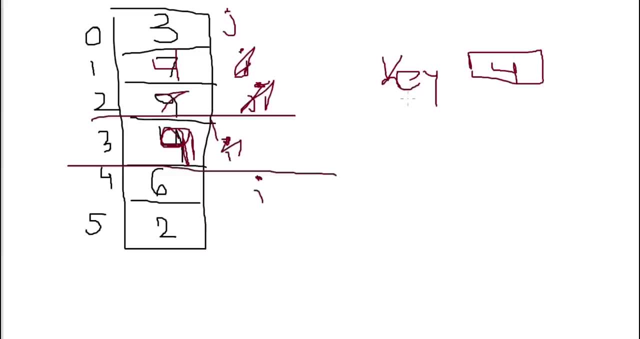 get this ascending order of it. So I hope you understood this concept of insertion sort Really. if you took this concept and overall like, take a practice of it, I definitely know that you can do it. So next off, we're going to be diving into another algorithm. Let's dive into the. 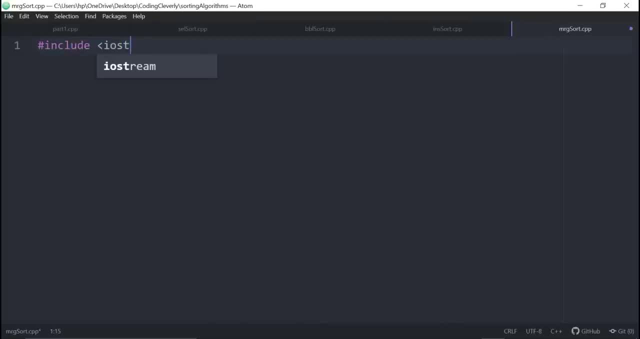 merge sort algorithm. So let's just type along IO, stream, Namespace, standard, main and the return zero semicolon. Okay, so let's create some functions here And let's just explain it the way we do it. So first of all, let's just find our way for the merge sort. So we're going to initially 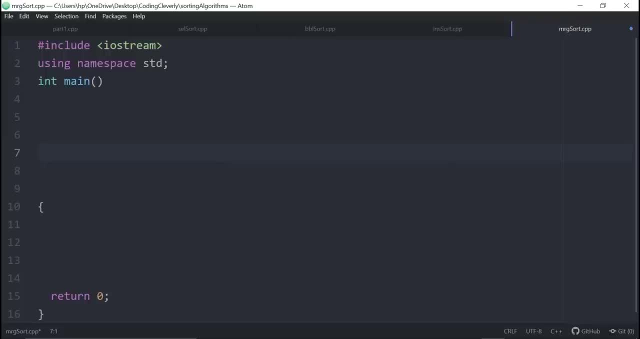 have a merge sort function, And then we're going to have a merge sort function, And then we're going to have a merge sort function. So how this is going to work is basically we're going to say, void, mr g s o r t, And we're going to say we're going to have an array inside of it And we're 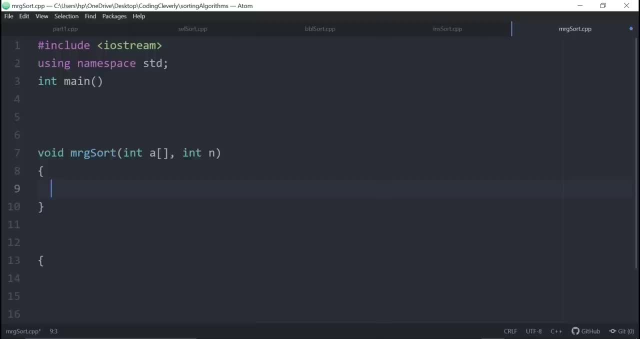 going to have the size of that, Alright, so this is going to have another function inside of it. it's going to call another function And what this process is called is called. actually, this is called a wrapper function And it's going to pass into an auxiliary function. So this is a wrapper. 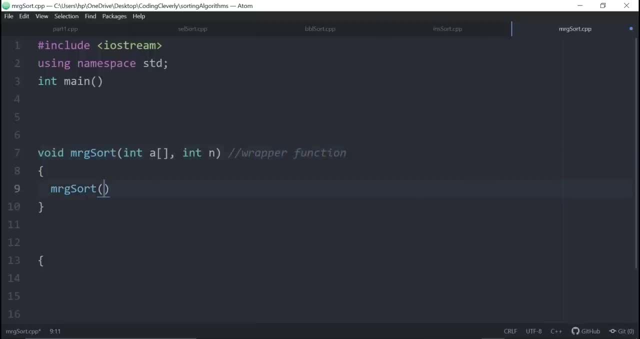 function Alright. so what we say is: this is merge sort and it's going to have the array inside of it, it's going to have the size of that array And it's also going to have one other additional parameter. So additional thing is that it's going to have the size, but before that it's going to 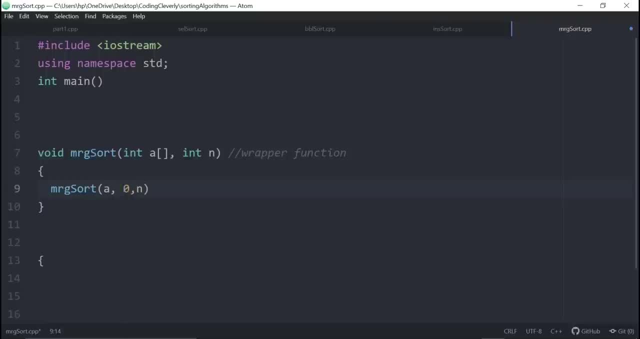 have one other thing: it should have the index of the first element. So it's going to be the array, the index of the first element and then the size of that, basically size minus one, And this is how the merge sort is going to be. 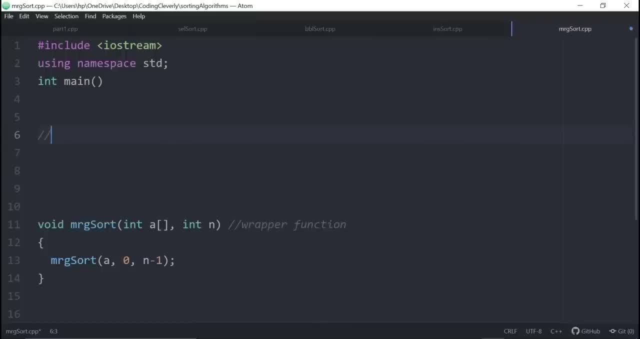 Over here we're going to have that auxiliary function called, So on the top we could just specify our auxiliary function So a u, x, i, l, i, a r y function, And what we could say over here is: we use the same void, Mr G s o r t, And now the same input parameters. 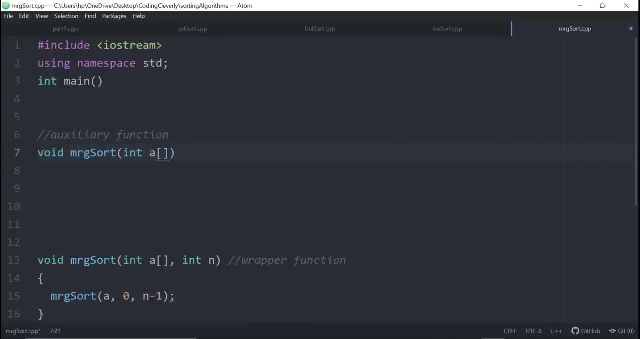 where we have an array. So we have this input array, we have basically the start value and we have the end value. Okay, these are the basically the indexes, And we call this as the auxiliary function or we also known as a, say, helper function. These are some of the names we're going to use. 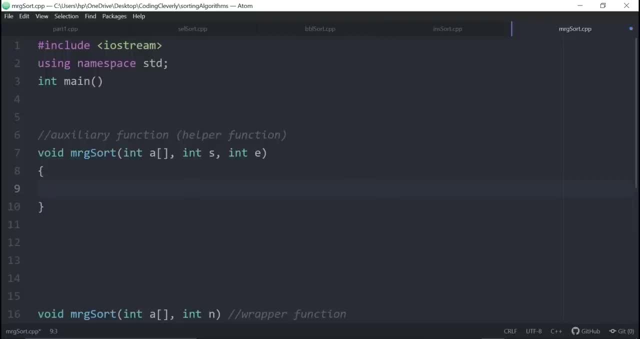 So let's have a base case to this. Now, Yeah, I don't know what a merge sort is right now. we just basically drew out the thing over here. So we have this function and calls to another function. Another scenario here we have is basically a same array And somehow 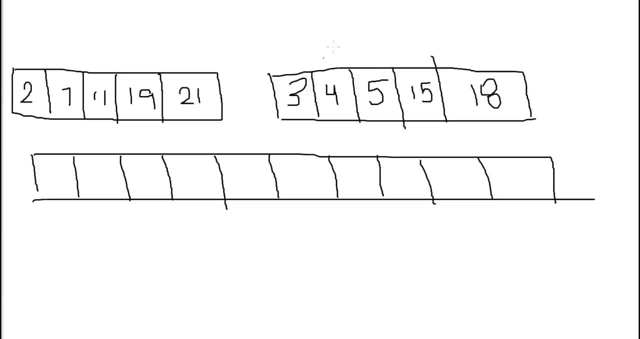 we can do this is we have this first part of the array sorted in sections, So you have a first part which is sorted and the second part is sorted, And what we, our job here is don't think of this as just two arrays. this is one single array And somehow we have this first part sorted. 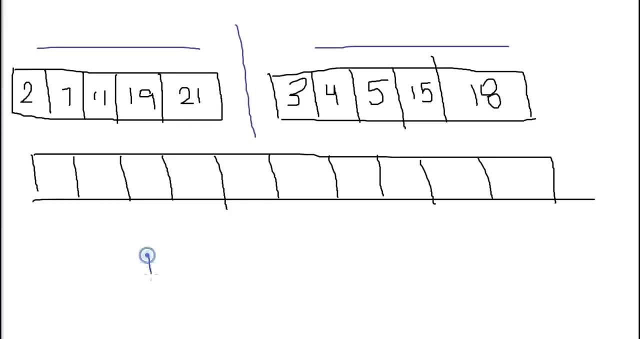 and we have the second part sorted, And our job is to make this sorted in one hole, And how we can do this is the process of merge. So we're going to use merge sort algorithm to do this. So what we can do is: 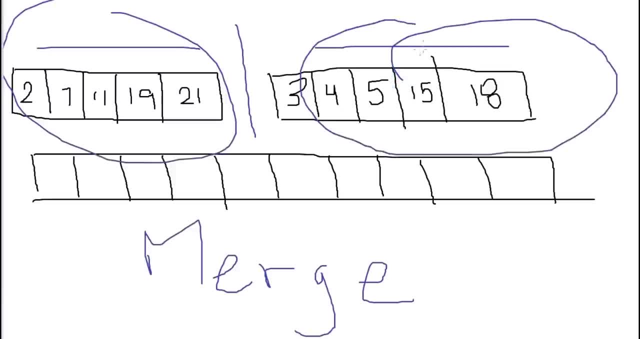 how the first part is sorted or the second part sorted. And we have to put a trust, We have to put faith in one process, And that famous process is called recursion. And now that's what we're gonna be applying. So you're gonna check. 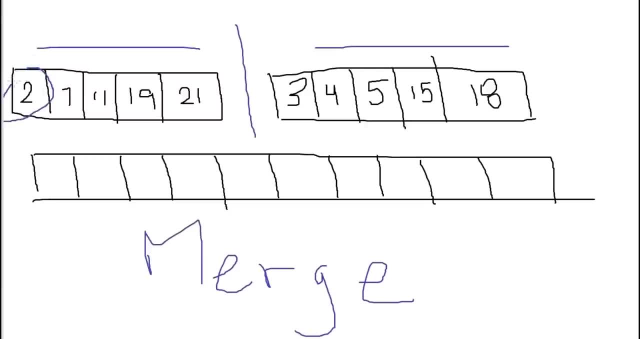 and the process is gonna go like this. So we're gonna have this first, element two, and we're gonna check this third up this part over here. So first, first of these two sub arrays- and I'm gonna say two and three, which one is greater? 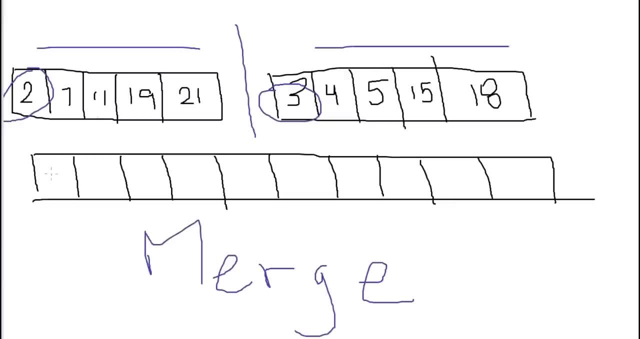 I mean, which one is smaller? So basically, two is smaller, So a two is gonna be planted here, And then this is gonna be incremented, So this sub array index is gonna be incremented, So it's gonna be plus one, which is gonna be seven now. 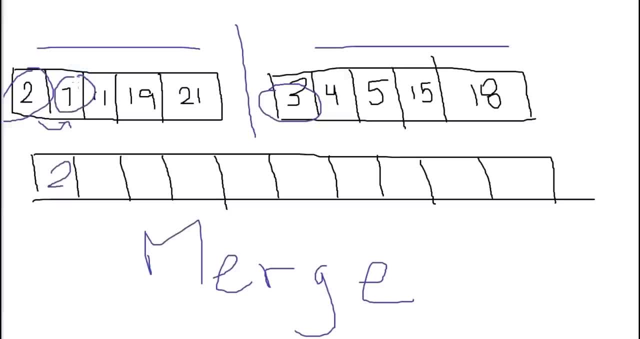 And this part is gonna remain the same. Now three and seven will be compared And we could see that three is lower. So three is gonna be placed in here, And now this is gonna be incremented to four. So you could see that four and seven will be compared. 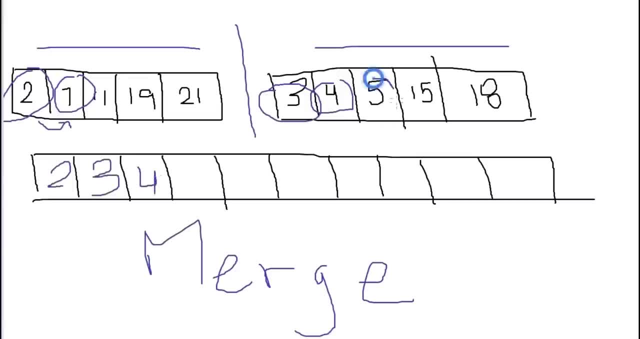 and we have four over here. So four is gonna be, and now this is gonna be incremented to five. So five and seven, and five is now gonna be added, So five is gonna be here. Now it's gonna be 15 and seven. 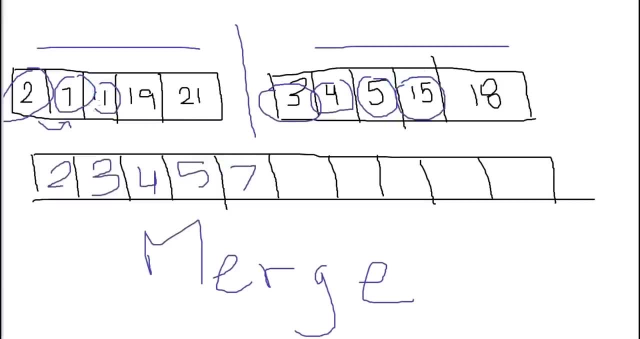 So seven is gonna be here, So seven is gonna be here. Now 11 and 15, you can see 11 is smaller, So 11 is gonna be in here, So it's gonna be incremented to 19.. So we have 15 and 19.. 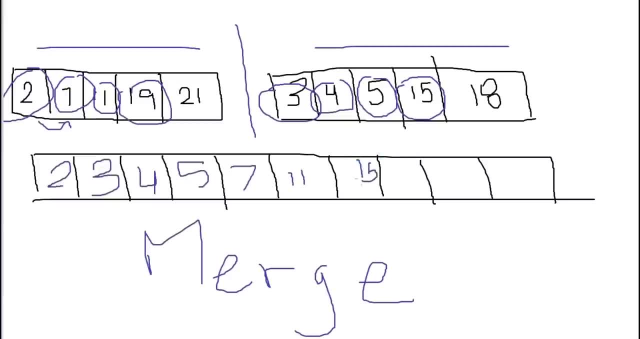 So now we have 15 over here, So 15 is gonna be over here. And then we have this compared to: 15 is gonna be incremented to plus, plus, So we have 18 and 19.. So what is it? 18.. 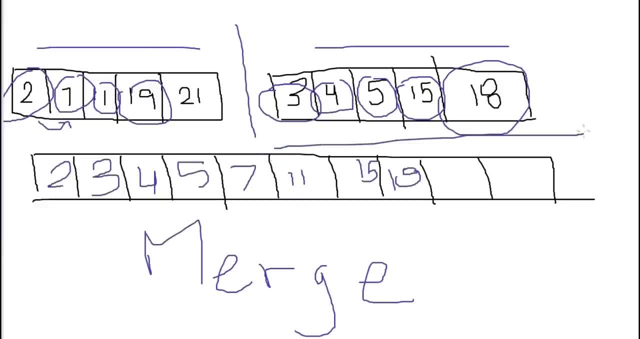 So now you could see over here, we assumed that this part is already full. Now, what do we do? Well, now, what we're gonna do is basically this last part we're just gonna append to the end. So that's our process here. 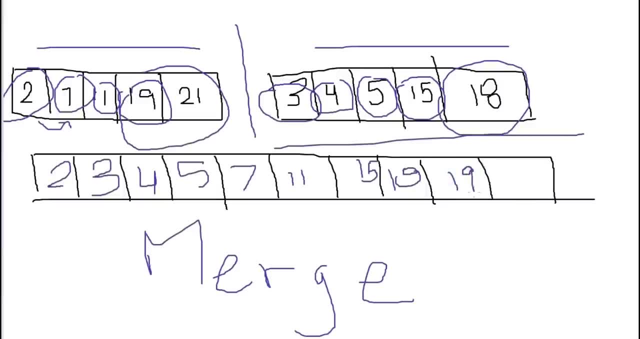 What we're gonna do is append these 19 and 21 to the end. How are we gonna do this? And you could see by: this is just sorted in our ascending order fashion And that's what we required. And how do we do this. 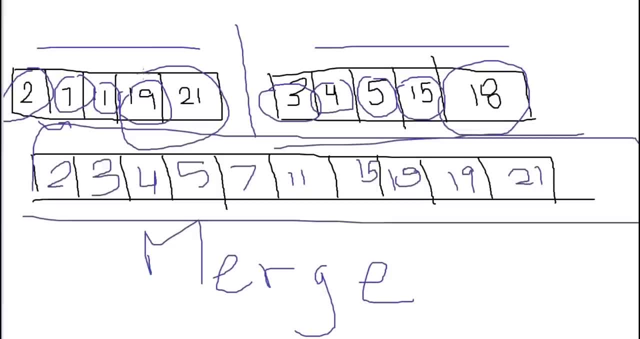 And you would ask me now, if it was sorted like this, why not just put like a pre-existing sorting algorithm, like a merge, like something like insertion sort or selection sort? Well, that process is gonna take longer And this process is fairly shorter. 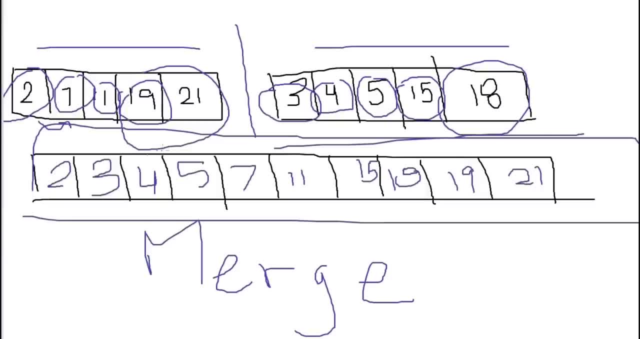 That's the crux of merging. It's a merge sort And that's why it makes it faster. It's much more faster as compared to any of the sorting algorithms we've discussed so far. So now let's go back into our code. 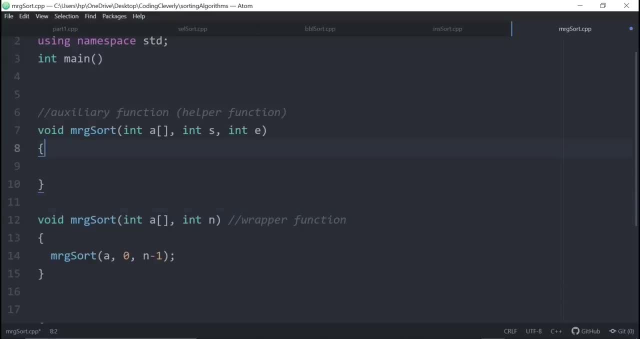 and now let's start typing along. So first of all, let's have this merge sort And inside of this we have an array, We have this int s, we have this int e, We have a helper function out in the condition. 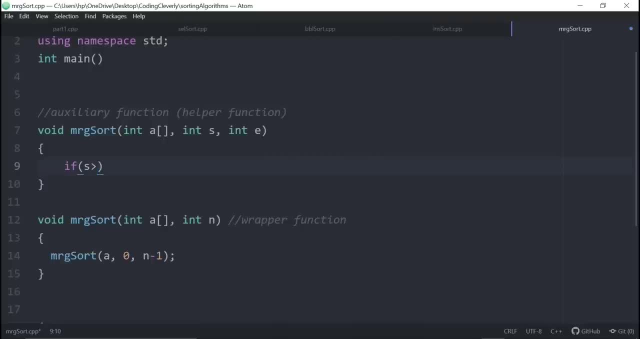 We have a base case Now. we have this s greater than equal to e. This is some case. that's not true, It can never be true, And in this case it will just return. So this is our base case And that after that you could say: 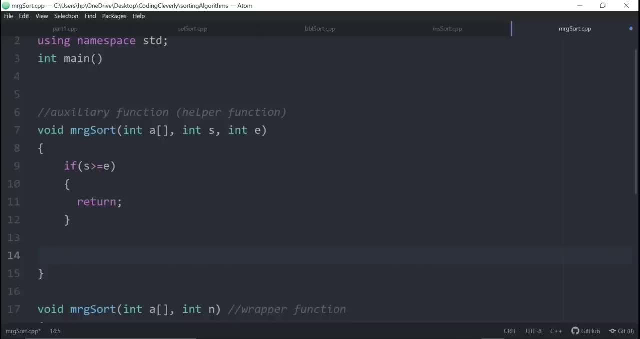 that this is not gonna be true, because start is never gonna be greater than or equal to e. That means that it's just illogical. Always you have a start which is less than equal to e, And I'm talking about the indices over here. 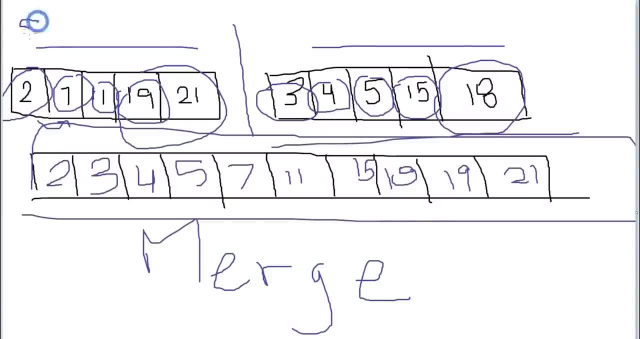 and not the value. So you have a start like, for instance: we have a start here and we have an end over here. Obviously, these are indexes and indices are. start from zero all the way to n. right Indices start from n minus one. 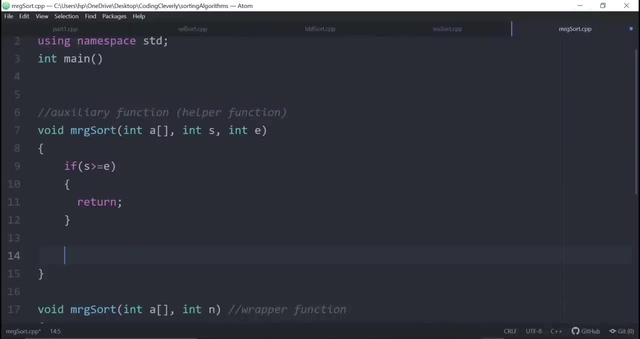 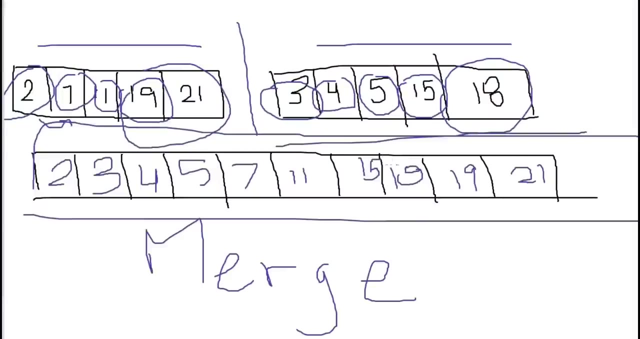 It never does the other way around. So that's just illogical. And now we're gonna have the implementation array. We're gonna find the midpoint value of that array. So this is our function here. So what we have to do here is basically manage this. 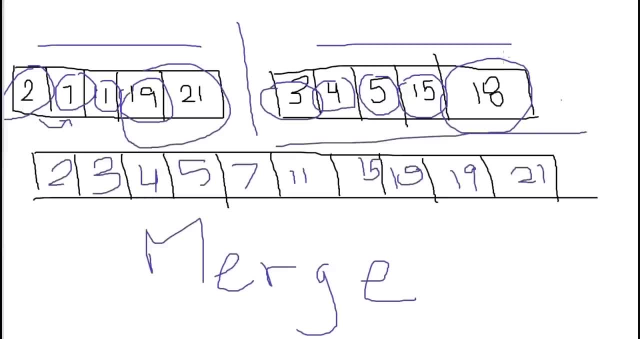 Let me just put these plots back, okay. So our process here is: we have to find the midpoint value which is right here. So you can see over here if I observe here that I have one, two, three, four, five, six, seven. 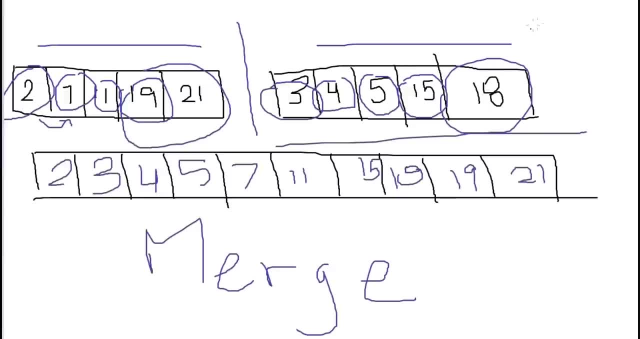 eight, nine, 10,, 10 elements, And if I go from here, like the start value, which is zero index, and the last value, which is nine, And if I divide this by two, I'm gonna get a 4.5, right. 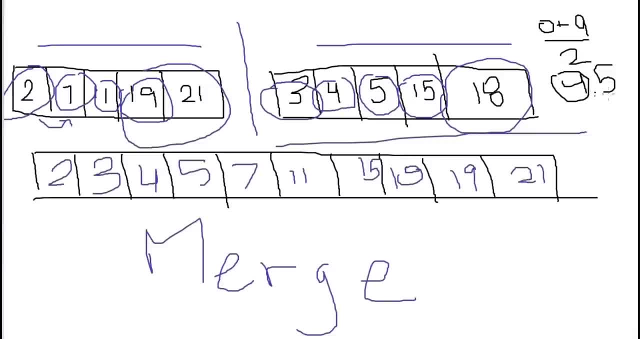 And I'm gonna get the integer division of it. So I'm just gonna get the four part. The decimal part is just gonna be excluded. So we're gonna have zero, one, two, three, four. This is our fourth index. 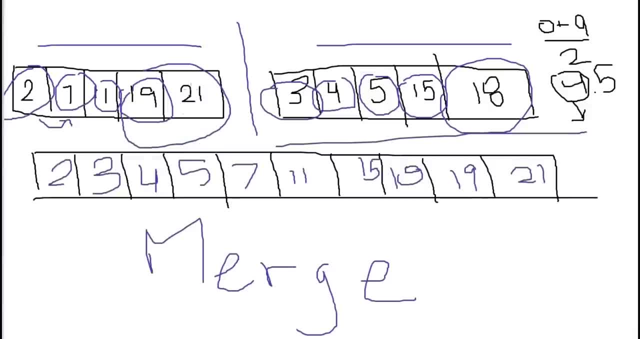 So this is our fourth index right here, And what I'm gonna do here is I'm gonna place that value. So, basically, this is our four index and we're gonna split this here, And this is now. you could see that this is our mid M. 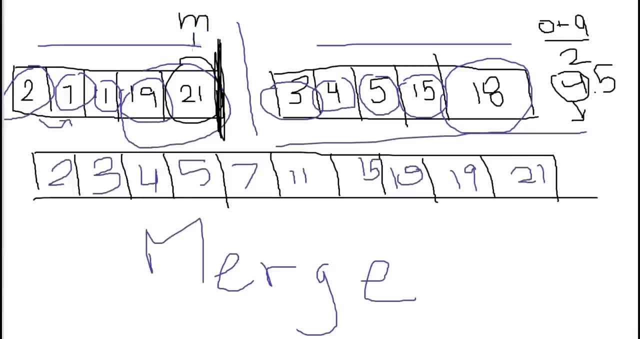 and I would say this is our M and the stuff that is before is gonna be the things. so zero one, two, three is gonna be four, And then after this is zero one, two, three, four. So this is five over here and this is four. 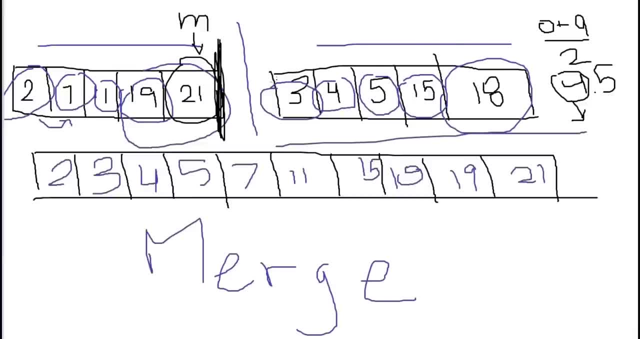 And this is our midpoint. Now suppose if we added something like had an odd number, then we'd have even cases here, But in this case we don't have. But this still is our process. This is how it's gonna be implemented. 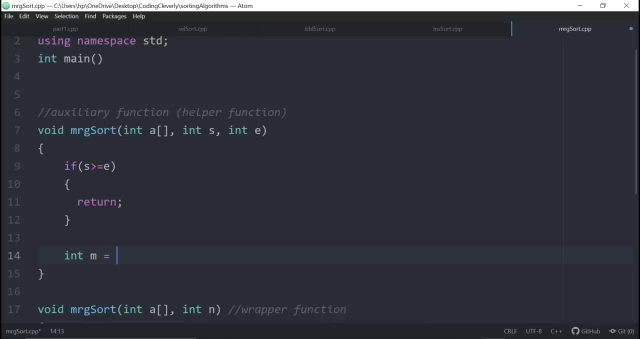 Go back here and we have this mid And this is gonna be a simple function where we're gonna do It's gonna be S plus E. Now this is gonna be the start index and the last index and we divide it by two. 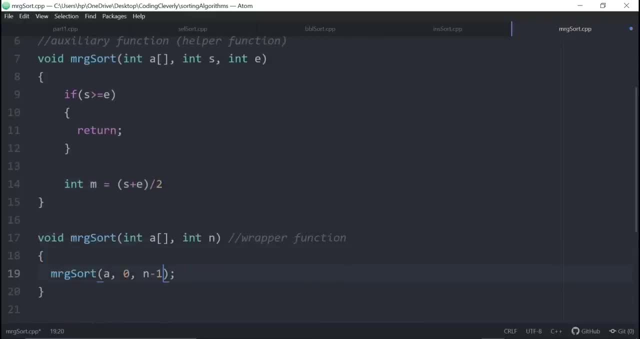 Just like we discussed- And I know that's pretty, really simple, Because this is N minus one- I told you over here that that's the last element. E is indicating the last element And it's just gonna divide it by two. 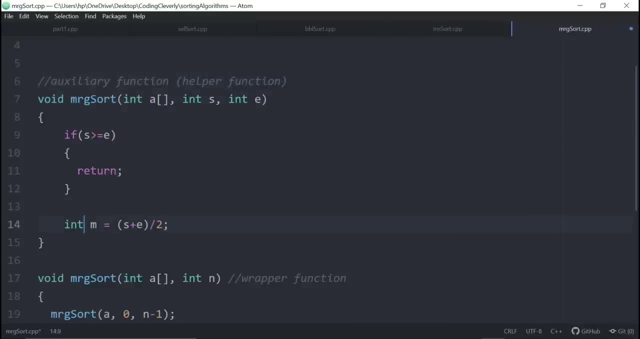 which is give a 4.5,. it's gonna be four Because it's an integer division. Okay, so now let's have that merge sort calling using recursion. That's what I was talking about. It's gonna start from A. this is our starting point. 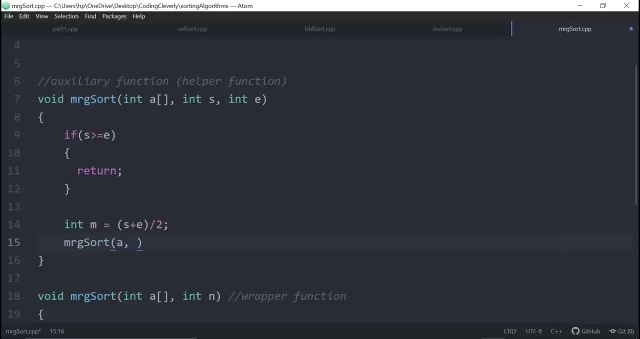 Now careful here that it's gonna. if this is an array, the starting point is S, but the end point is now M. Why? Because now we're gonna try to split into two subarrays with sorted processes. So merge, sort, we're gonna call again. 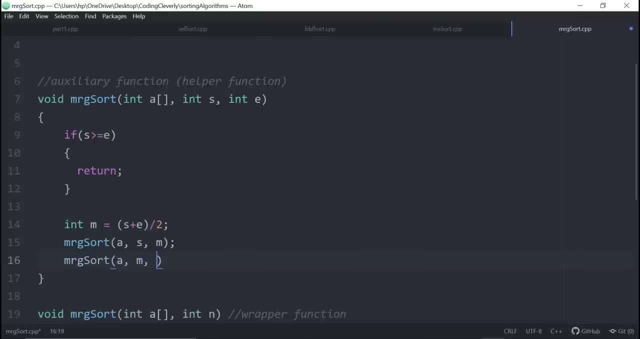 And the second time we're gonna have A array, it's gonna start from M and it's gonna go all the way to the end. So it's gonna be not M, but M plus one, Because now we're gonna have this process. 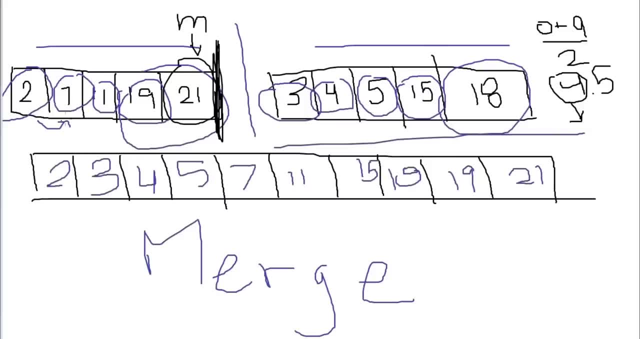 Additional. so over here we have this portion we want sorted and we want this portion sorted. So we're just discussing right now this portion, not this thing over here, not this. right now We're just looking at the top. So I hope you got the point over here. 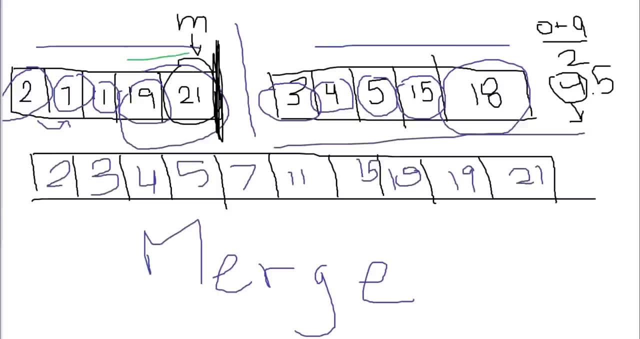 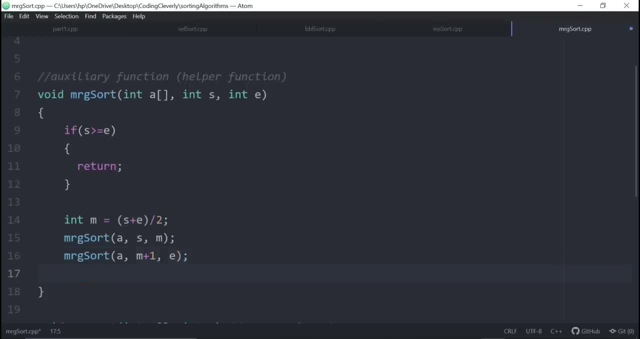 that we wanted this sorted in ascending Ys over here and ascending Ys here. Okay, so back over here we have this M plus one, And now we call one more function, And that function is basically the combined function And the combined function. 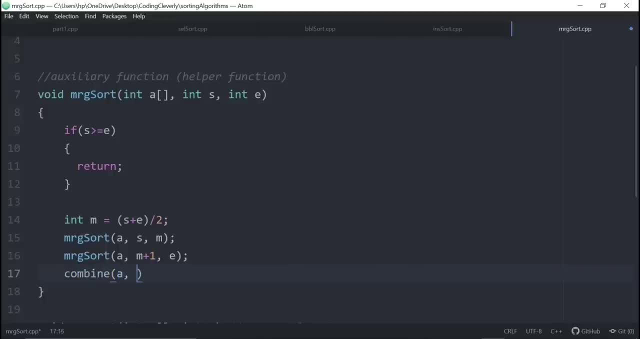 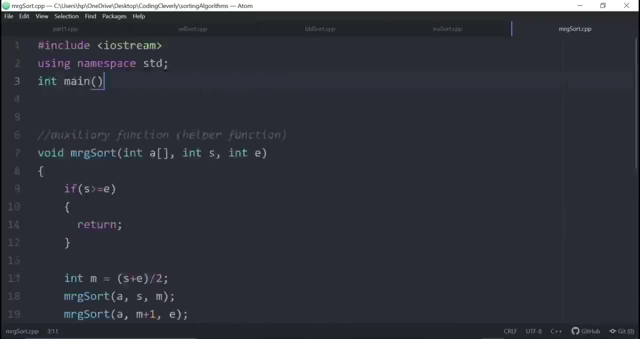 is gonna be pretty much something like this: We have an A array, we have the S, which is the start, We have the middle value, which is M, which is the last value, which is E, And this combined will be defined over here somewhere. 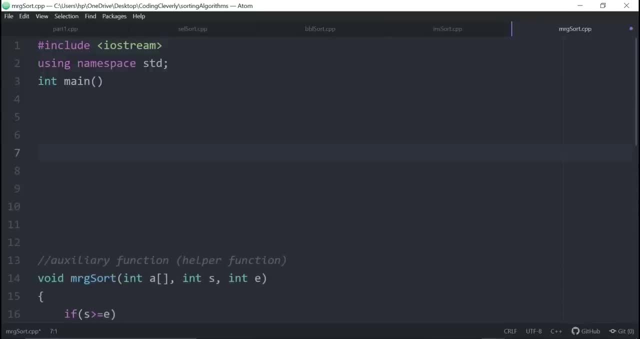 So let's have this combined defined. So now what we're gonna do is basically we're gonna say void combine, And if I have that specified here, I would say int A, And then we have this array right here We have an int S starting value. 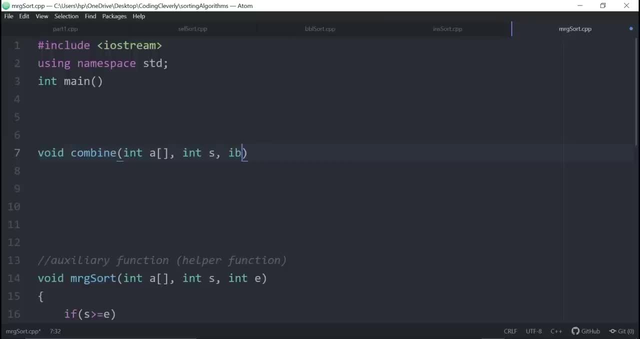 We have an int M, which is the middle value. Forget that right. And then I got the last element, which is end, And what we could do here is that we want a temporary buffer, And I'll tell you why. just hold on a moment. 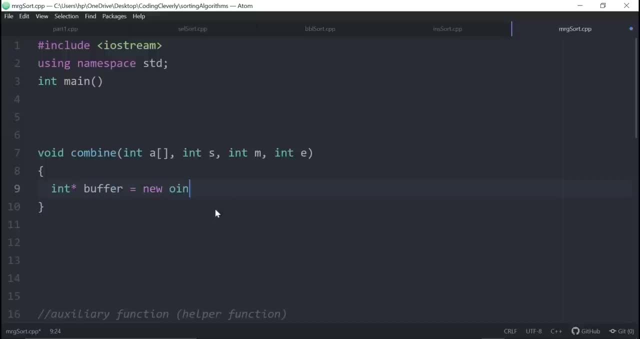 So let's just create a buffer over here And what it's gonna do is basically gonna get some value from the heap or it's gonna get some. so it's gonna be in A, it's gonna be a, an array from the heap that we're gonna get. 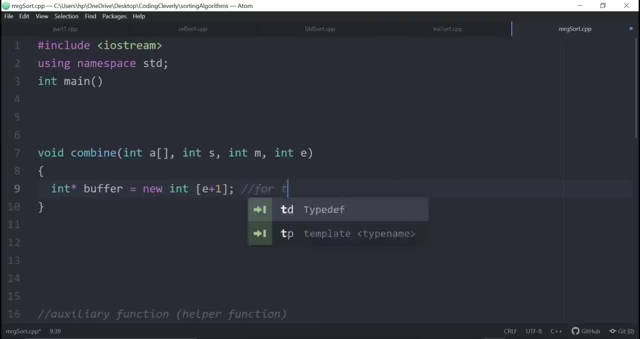 And basically, this is gonna be representing for the total size of the merged array. what we're talking about And what we're gonna do here is that we're gonna have a K is equal to S and we're gonna say while, so while is over here, and we can say K less than equal to E. 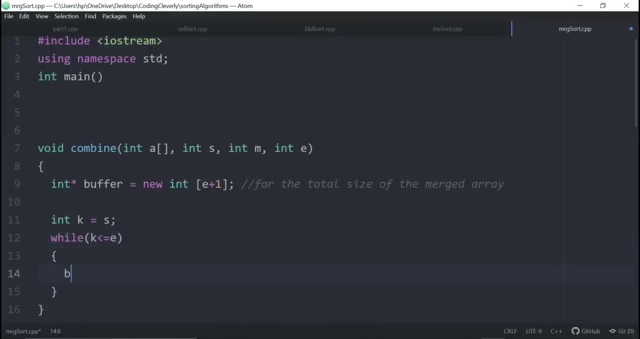 And what we do here is buffer, And we say: buffer, sub K is equal to a sub K, And we would say: K is equal to K plus one. Now, what do you mean by this? Now I'll tell you what this means. 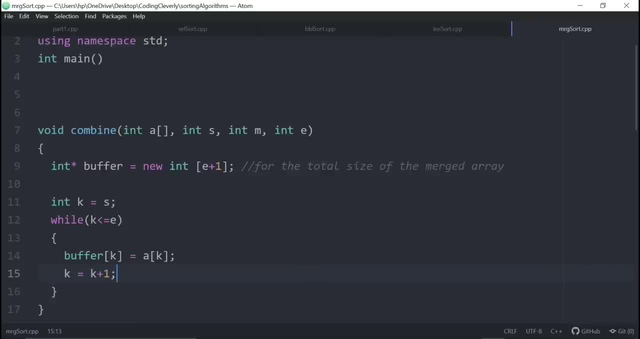 The thing is that we're creating a temporary buffer that we're allocating from the heap and then we're gonna deallocate it using the delete keyword, but before that we're using it because we don't want to reassign it in that existing array. So we want it basically. 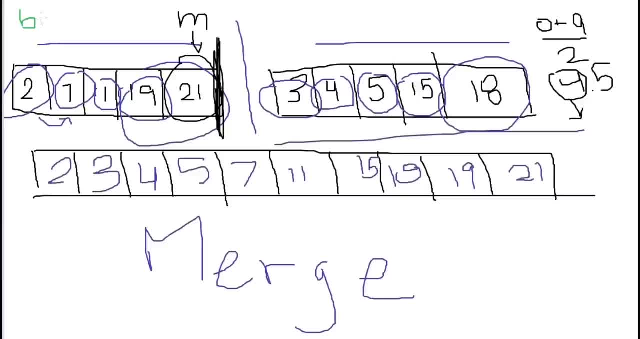 stored And then we want something over here. So I would just say, this portion here, B U F F E R, this is the buffer, this portion and this whole thing. I'm talking about the whole thing. 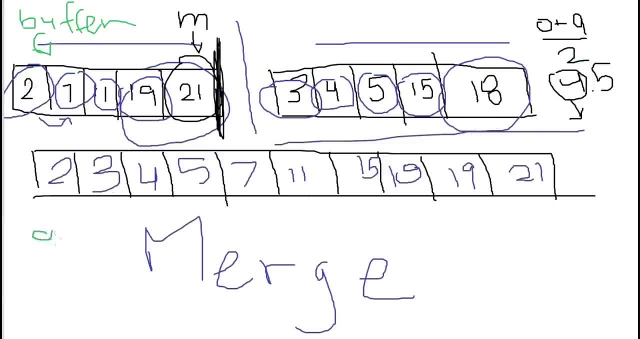 So this is buffer And this is going to be our output array. So this is going to be the sorted array. we're doing in two separate things Because if we sort in just one single array, it's going to cause complexities, much more complexities, as just copying the elements. 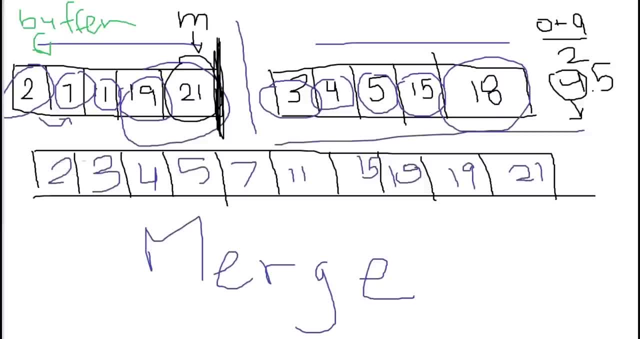 So suppose we have this array, So just ignore this part because it's not sorted right now. And we just created a duplicate array that had all the values. So it started from K and it went, so it said zero all the way to the value last one. So if I go back here you can see that K. 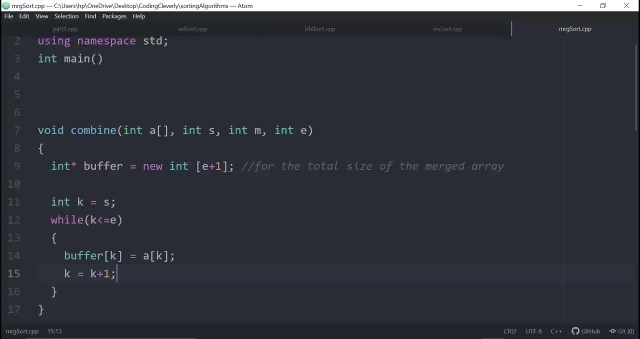 started with a starting value and it was less than equal to n value And it just said buffer sub k is equal to buffer sub k. So a sub k, whatever the values were, it's going to sort in the buffer. So it just initialized all of them and just k plus one all the way to the end. So just copied. 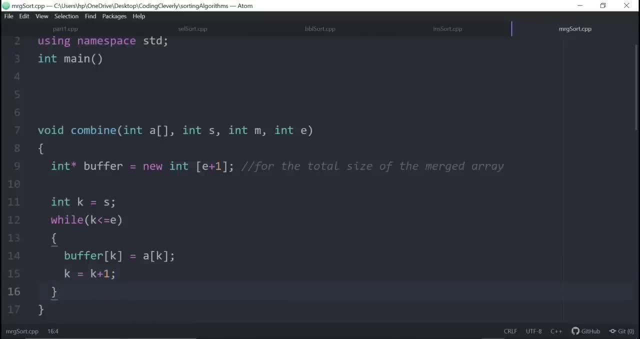 them made a duplicate right. So now, after that we could do is we're going to have something specified here right after this. So once it's copied, we have i is equal to s. Now we're going to have one thing over here, which is j, And we're going to say m plus one, And I'll tell you why we. 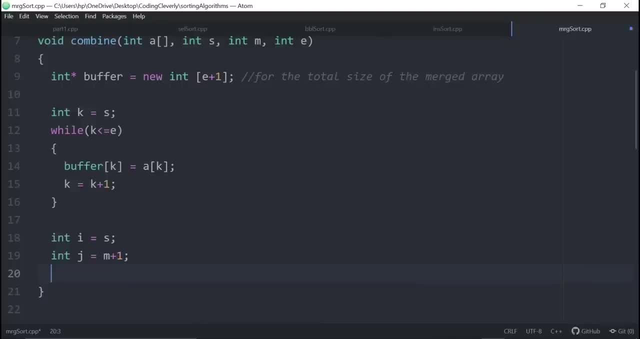 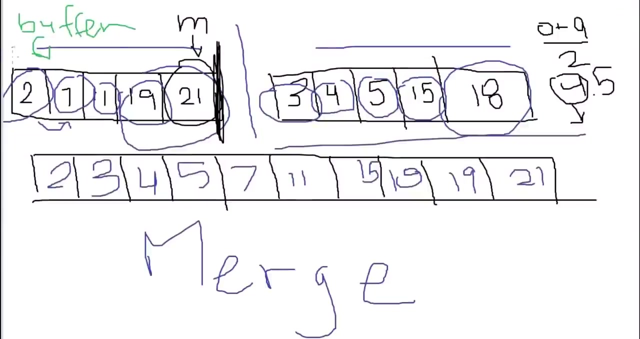 did this And we also have which is k And we said that as s, So i is equal to s. go back here And we have this i and it's going to be over here, which is the starting value. just give me another color over here, I'll just get a little darker, Okay. 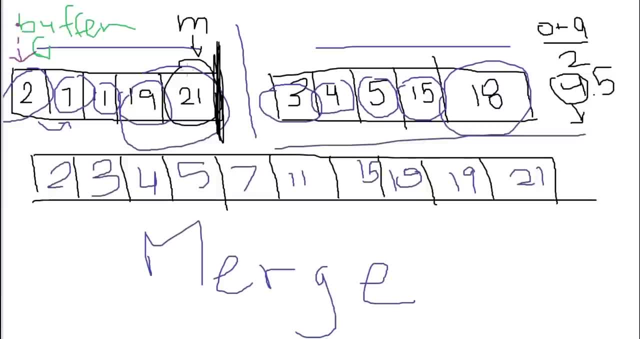 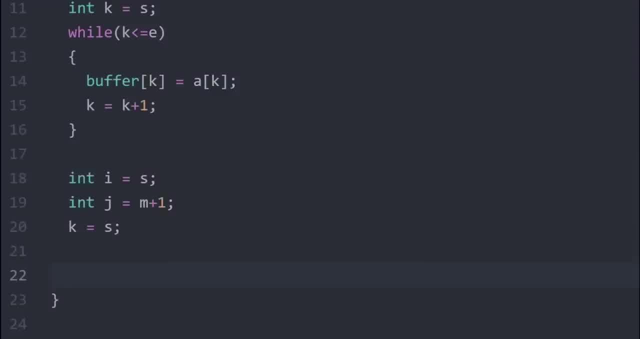 so i is over here, which is right here. And the second one, what we have is this mid. we know that, Okay, so other one we have is: j is equal to m plus one. So if I go back here, we have this j. 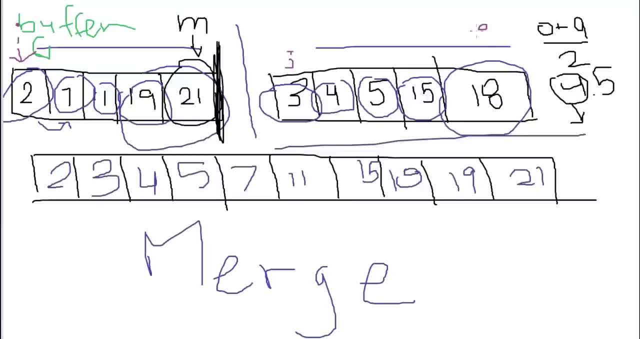 is this over here, And we know that this is endpoint right here: e. So you can see that this i has to go increment all the way to the M- this is its last element- And this j has to increment all the way to the end of portion here. So that's how we're going to compare the values, like two and 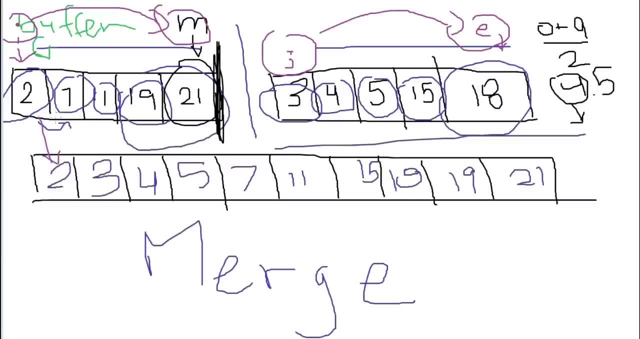 three, which one is smaller? to plant it here, go increment two to plus seven, And then we're going to say seven and three, what is smaller? three smaller planted here, and then put the rest. So that's the process, what I'm trying to implement. 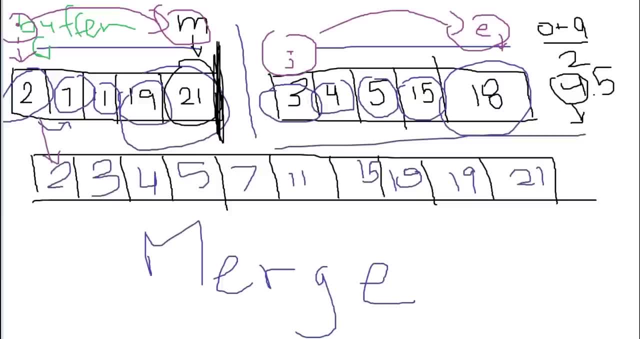 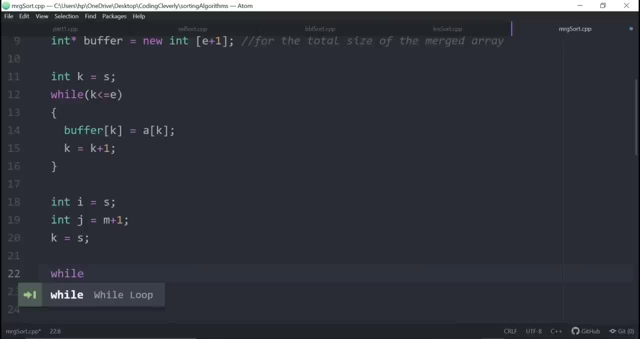 To code. I have to map this out, So that's why I'm using this diagram. That's what we're doing, So we're going to have into k, z to s while let's have a while loop, And this is how this is process. 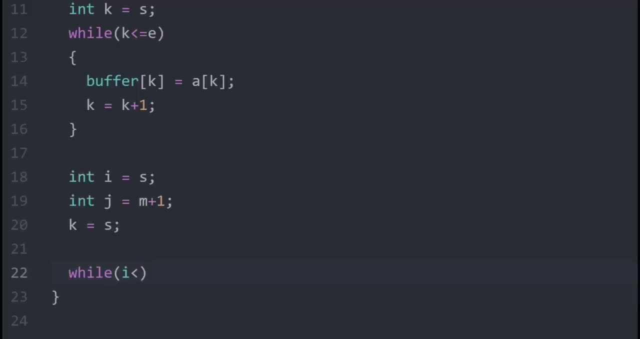 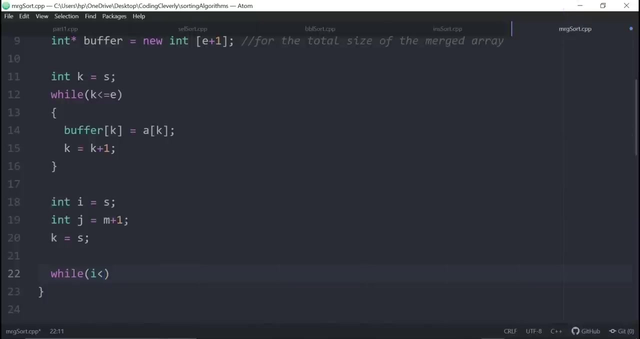 is going to go. I, which is that value, what I told you this over here: I is less than equal to m and j is less than equal to e. this some process is going to go on. So if I less than equal to m, 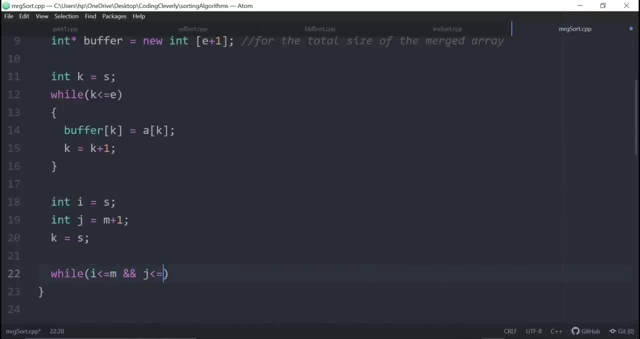 and we have j less than equal to e. we want some process Is going on. So if that buffer bu ff e r ff er is i and then we have less than equal to bu ff er sub j, if this process is done. so if a buffer sub i is less than equal to buffer sub k, 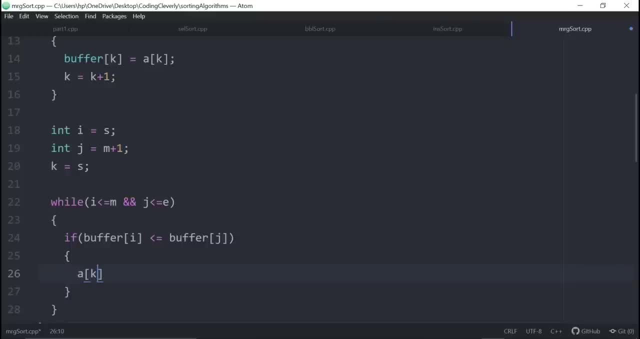 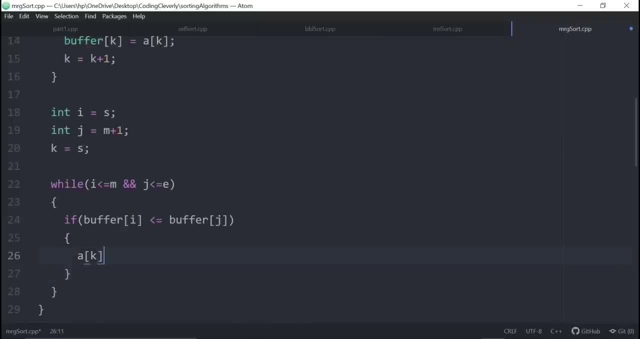 then just copy it inside of that k, then the array which is over here. we want to sort it out. So we're just gonna copy here through buffer. So it's a bu ff er sub i. so in the case, if it's, 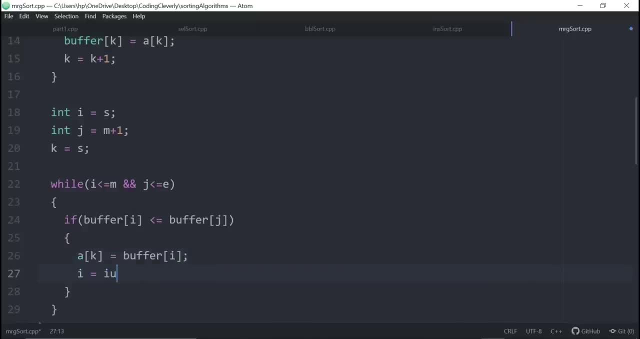 less, right If it's less or equal, and then we just increment: i is equal to i plus one, just what we did over there, just what we did over there. So if if that's not the case, we'll just have an ls. 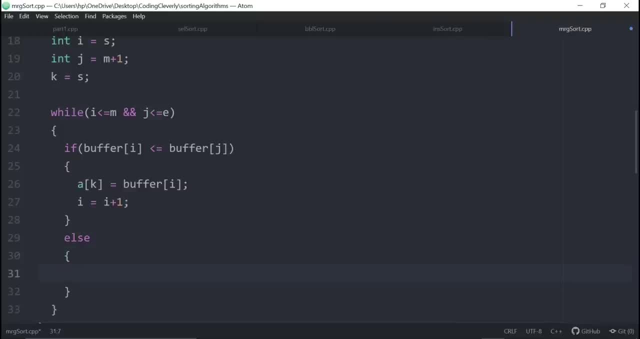 And we're gonna put something in here. So let me just put over here: The case here is that a sub k- a sub k- is going to be over here and it's going to equal to buffer, So it's going to be buffer, and then we're going to have sub j over here, So we're going to have this Jane. 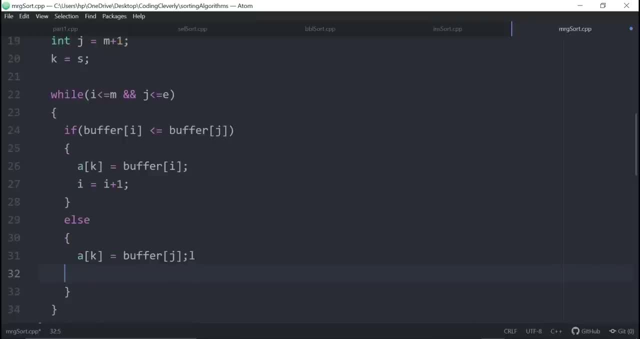 here, which is a sub k, because if it's not the case, it's going to be less right. So it meaning, if it's less, but if it's greater than the J is going to be there, And then obviously we're going to have J being incremented instead of the I being incremented. So we 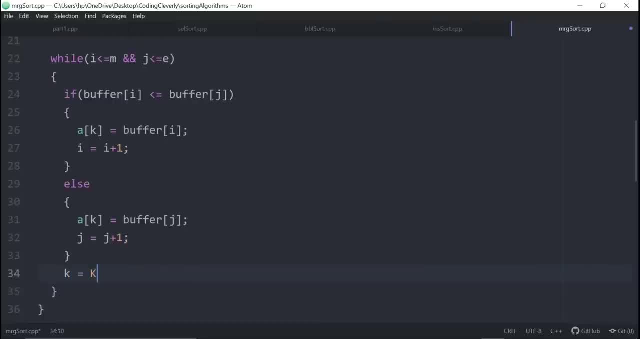 have that and we have: k is equal to k plus one. let me just have that. There you go, And now we have the condition here. So this is this case over here. this is a while loop And we have another while after this condition. Now I'll tell you the reason why behind this. 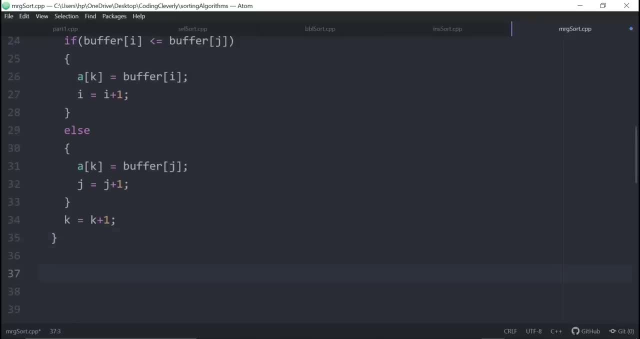 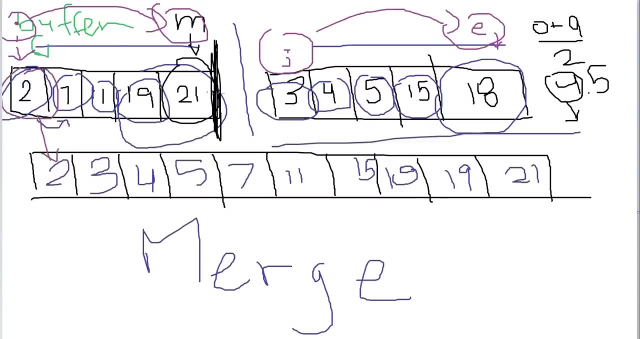 So we have this while loop And after this we have two while loops Additionally. I'll tell you the reason why we need those two. The thing is that if we compare these two- like suppose we had this two and we had this three- we compared it, that two was less and then we incremented it. 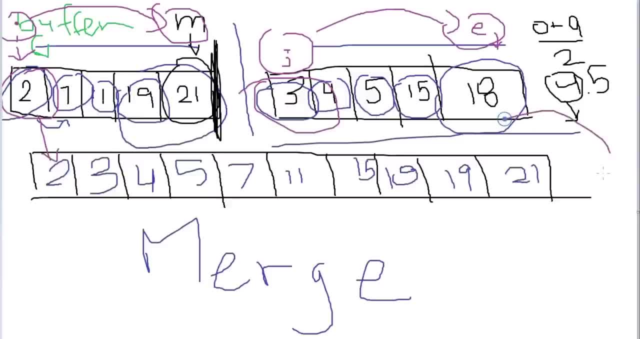 we're just doing plus, plus don't. we did. But the case when we came here, this 19 and 21,. how these come? this array just got full. all of this was full, remember this portion, but then we just appended these last two inside of this. how do we do that automatic process? 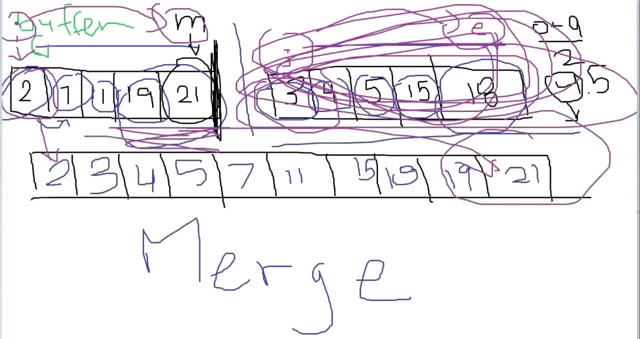 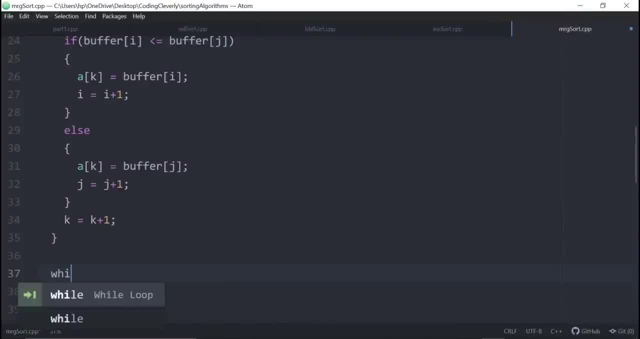 that automatic process was going to be. it's going to be done through two while loops. we're going to be including- and that condition is like: if I is less than equal to m or if J is less than equal to E. Now, this is the two conditions, And look at this carefully. 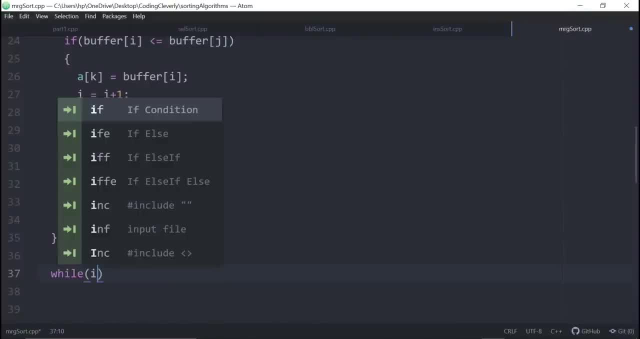 So while we say I is less than equal to m, So if this condition is like still there, like it's true, like it broke out, So the process here is that these two will never become false together. it was always going to be one, one of them and not the other, right? So if that, 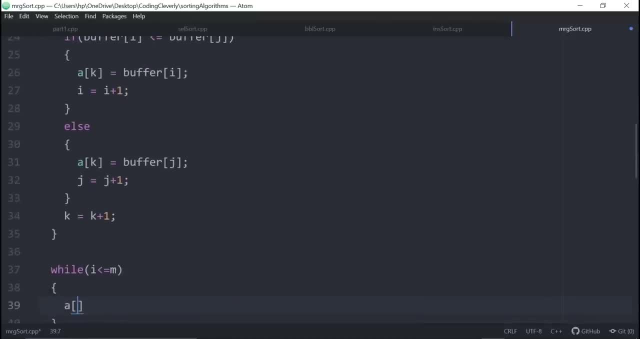 case like J is less than equal to E. that came, and then after that we still have eyes- less than equal to m. what we could do here is that a sub k- And this is the same scenario we did with the example- a sub k is equal to, we're going to say. we're going to say 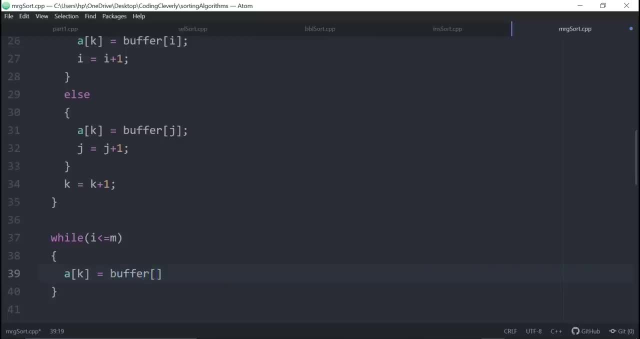 buffer, so that we got the thing from buffer and we said that as J, And what we do is basically, actually we're going to have that set with I, because it's I over here, And we're going to set that with I, and then we we're going to do is I, we're going to increment, I is. 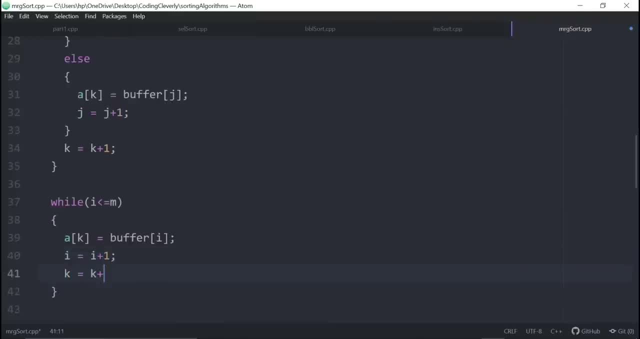 going to I plus one and we're going to increment the case. you get a k plus one And if the other cases there, like while j less than equal to E, we're going to have a sub k. k is equal to buffer And we're going to have that as j Sub. There you go And we 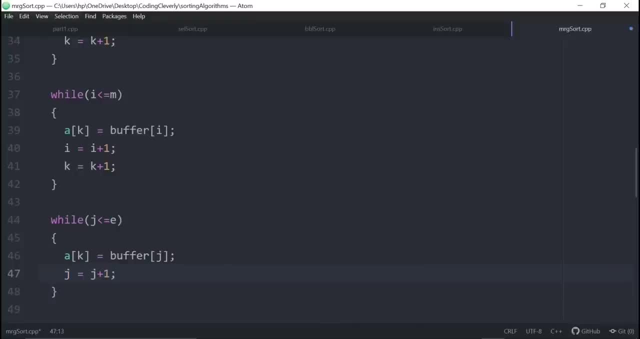 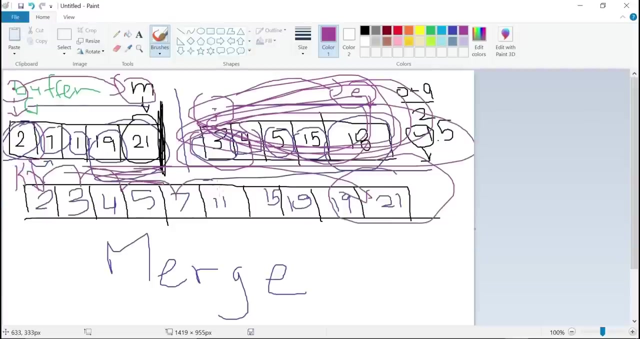 have j is equal to j plus one, And we have k is equal to k plus one. it's just going to increment the k value And you already know where k is starting. This is k, right here. So this portion is k and it's just going to go 12345678910.. All the way when. 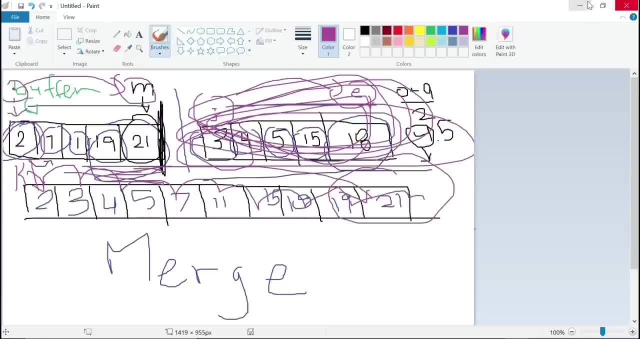 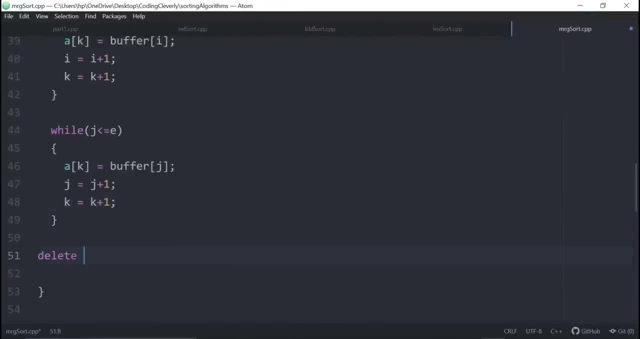 it's done. So it's just even incrementing. you can see the J's over here, eyes over there, And that's the process going behind of it. And then, once we're done with it- we don't want this extra memory- we just delete it. So we just delete our buffer And using this delete syntax is 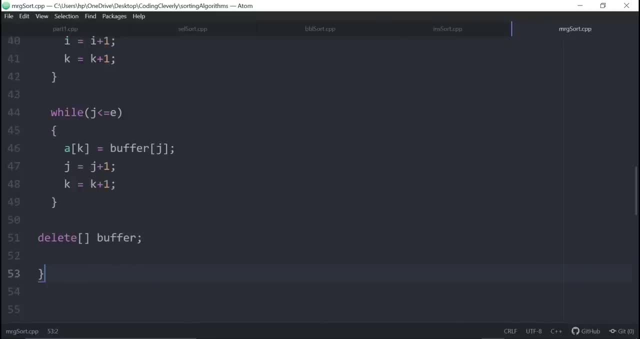 basically, we're going to de allocate it from the memory And that's it. Now let's just have this additional function that we need is basically, I think so it's a printer. So, oh, I forgot my main logic here in main. So this is main. 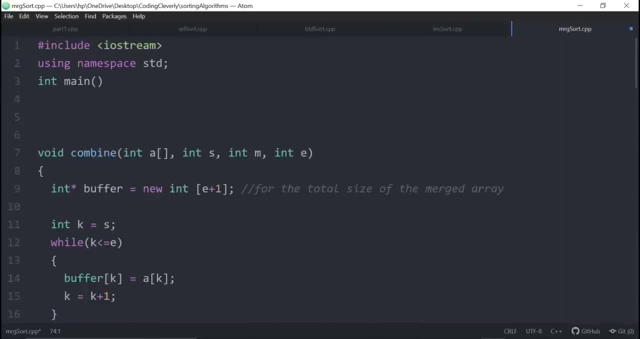 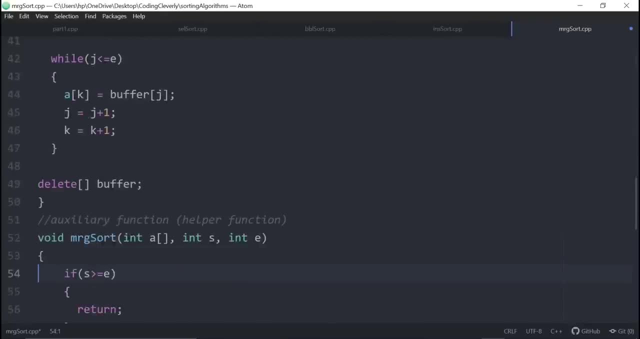 Well, maybe I left it up on the top. Yep, that's a common mistake. Okay, so just delete that portion here And let's just have a display function at the bottom here. So at the bottom value right here, Let's have a display function. So it's going to be called void, we're gonna. 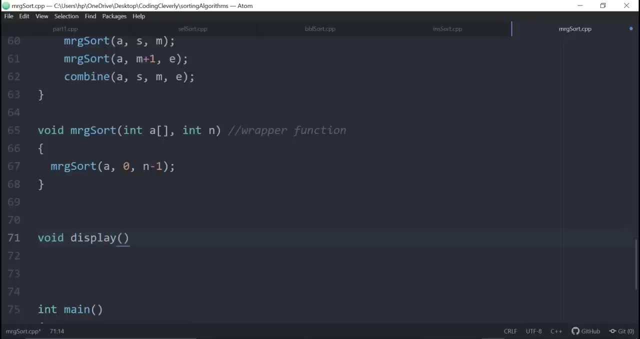 have a display And we're doing is basically having an array, just like the small other ones. So have the size N And we're going to have something which is going to be implementing, like we have temporary and we're gonna have that associated with a sub. what am I doing? 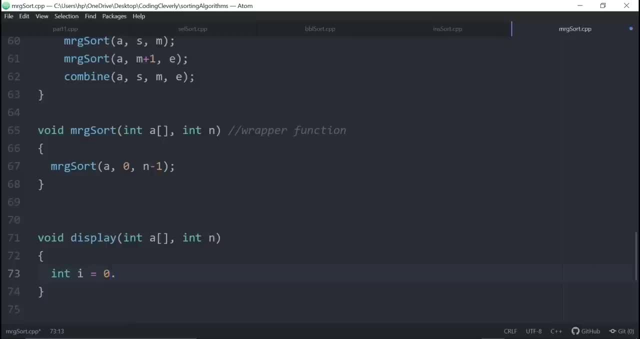 It's not actually that it's. I is equal to zero, my bad, So we're gonna have: while I is less than n, And then we could say: console output the array value, array sub i, and put that comma here, And then we have it. just keep on incrementing, plus, plus And yeah. 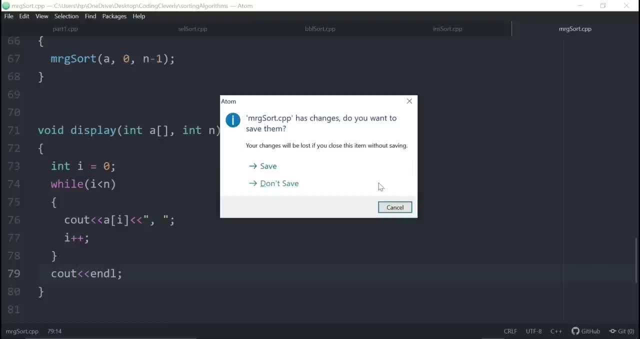 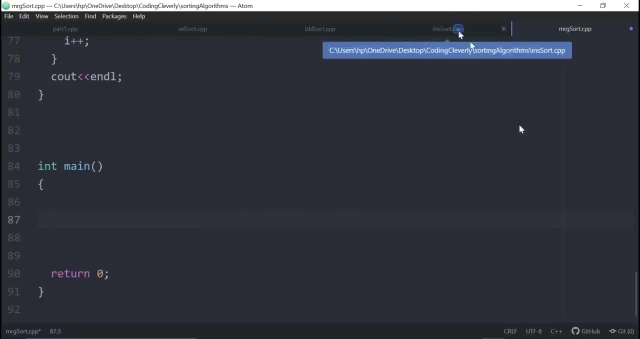 console output here. There you go, And now what we do is basically run the code here. So get a random array again. So let me just get this array, which is right here, copy here, copy and paste it here And let's just change up the thing over here which is insertion. 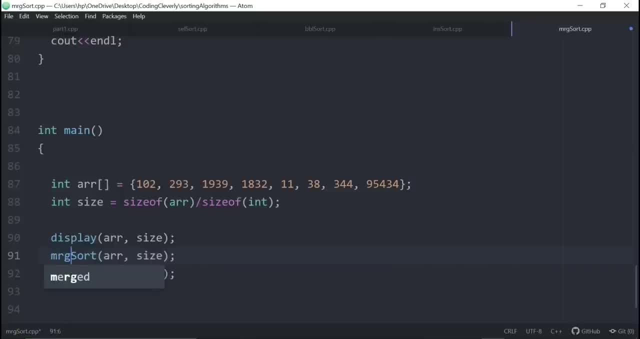 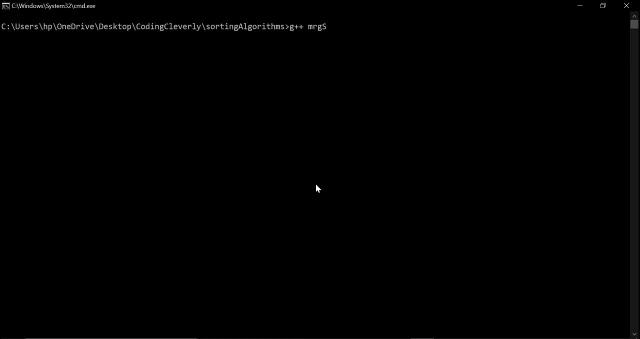 or sort. we're gonna have MRG, MRG, MRG, sort, merge, sort. So let's go back to our G plus plus compiler, G plus plus, G plus plus MRG. so our tcpp I've been: Oh, MRG, MRG, s o r t And a compiled MRG. 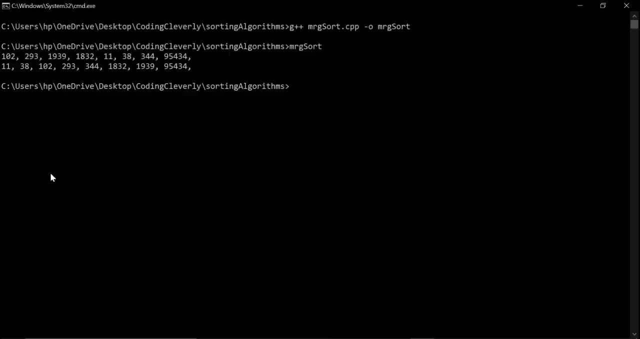 s o r t. There you go, Voila 110. And then 102,, whatever 293, and then all of that and sort it in ascending order. So that was it with merge sort, And this is much, much. 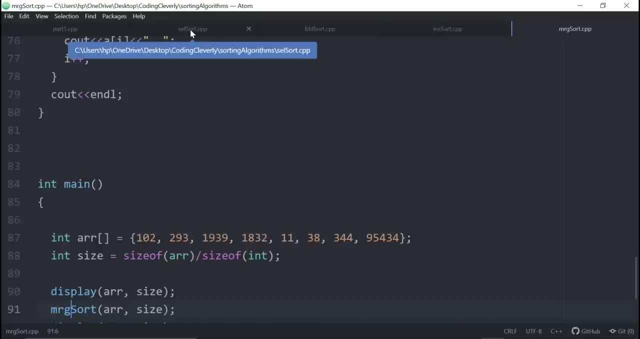 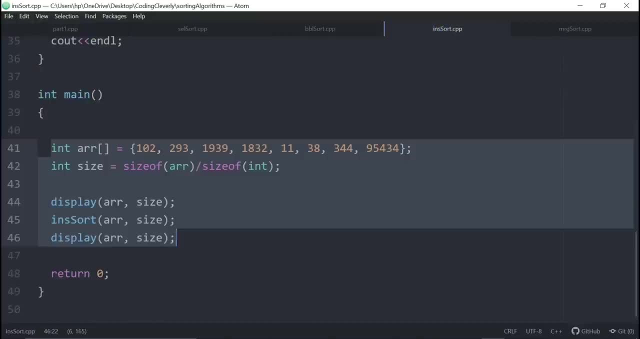 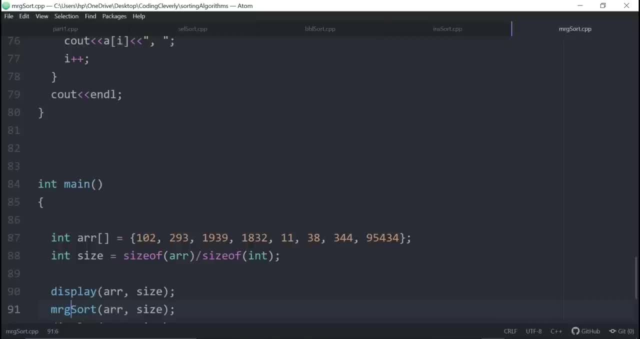 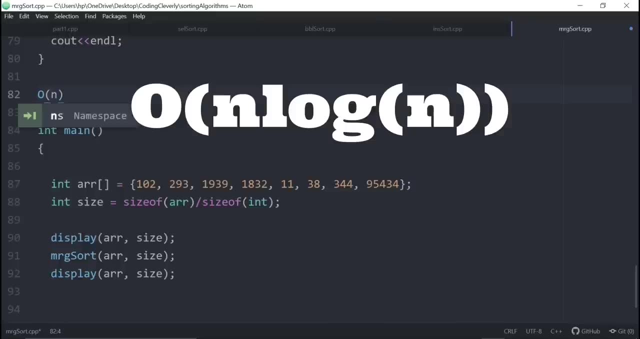 O of n squared. But this merge sort is somehow faster because it's doing the time complexity in O and log of n, So O and then we have n, And then we have log, And then we have that n inside of it And this is much, much more faster as compared to any of the other. 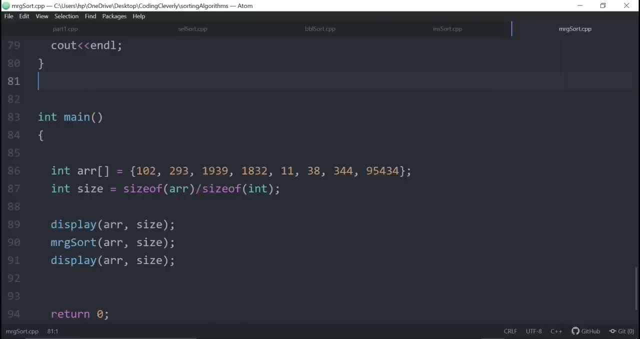 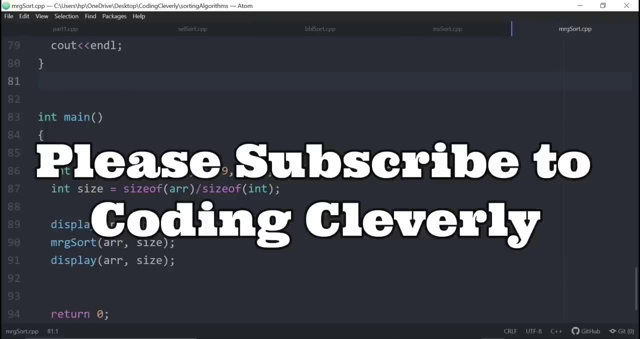 sorting algorithms Now if you get like a set of arrays from a text file that I could be doing in my other videos. so stay tuned for my next upcoming videos on my channel. you're going to be seeing that we're going to have a text files and we're going to be looking and comparing how. 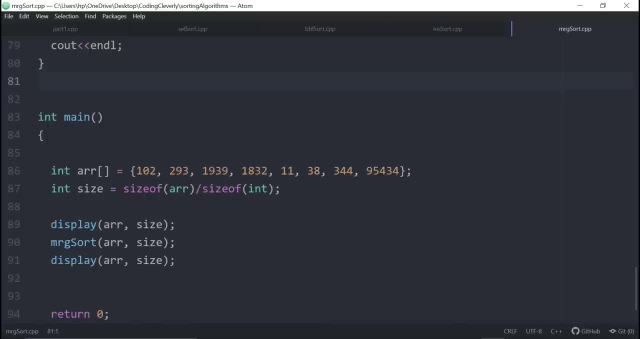 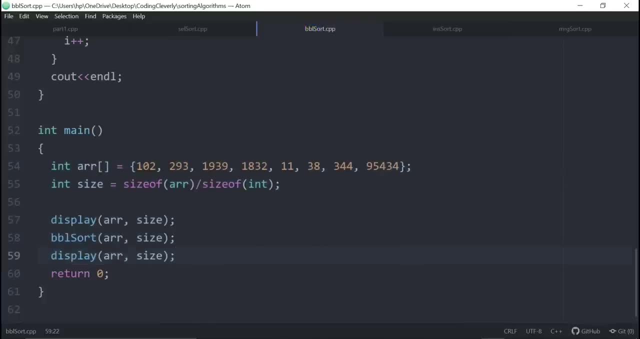 fast. is this compared to other sorting algorithms? Because if we have these O of n squared sorting algorithms, these are going to take much, much more time. as the input value increases, it's going to exponentially grow, But as compared to merge sort, it's just going to be fast. 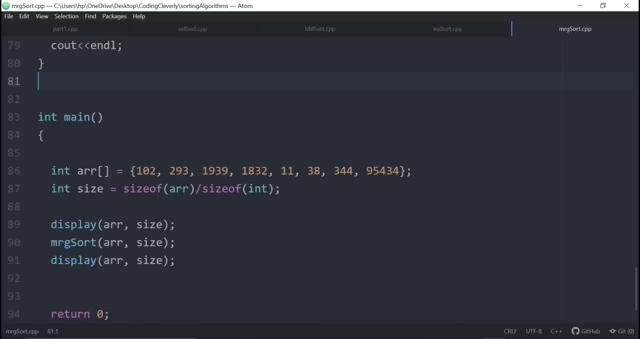 as lightning. So I hope you enjoyed this video, hope you liked it, And please make sure to visit my channel, which is called coding cleverly, where I have so much content of C++ And I've done data structures and algorithms, I have done object oriented programming and I've 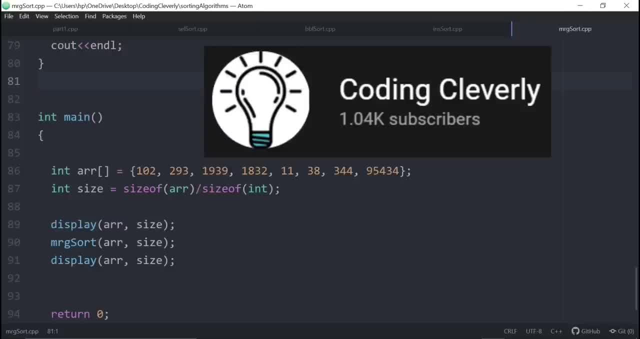 done the basics- beginner level, procedural programming- And I my my goal is to complete data structures And then after that I advanced to other project based videos, as well as new languages and technologies. So make sure to subscribe to that channel And yes, thank.